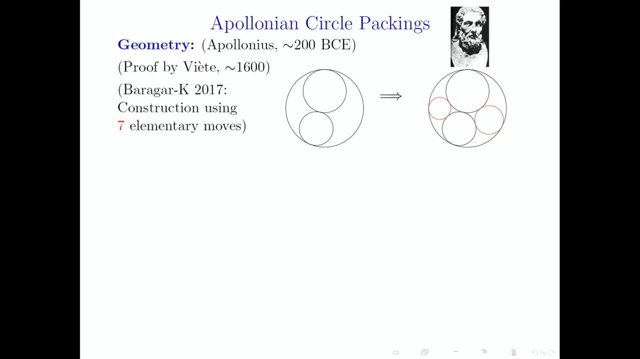 moves of the straight edge and compass which, if you really want, at the end I'll show you. Okay, so that's the Apollonian problem, Once you do that. so Leibniz is the first to have the idea to iterate this. So this is the dynamics of the Apollonian operation, And when you 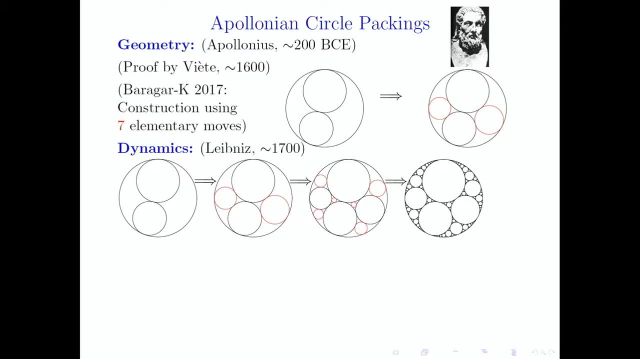 iterate it ad infinitum, you get what's called an Apollonian circle packing. And so the asymptotic growth rate of these circles was studied by O and myself a long time ago. And then the arithmetic comes in from a study by Fredrik Saadi in the 1930s. 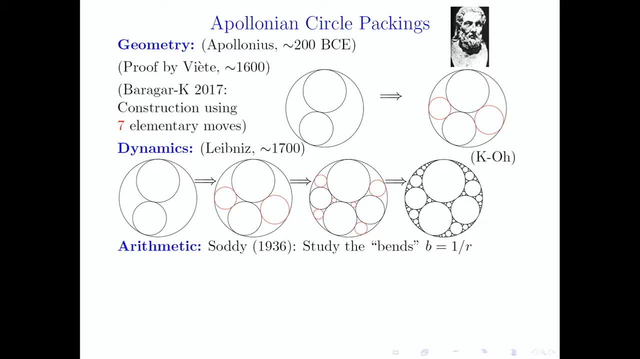 Somehow everybody else missed this before Saadi. But he says: let's look at the for circles it's curvatures, but in general we want to look at the reciprocals of the radii. So let's call those bends For spheres. the curvature is proportional to radius squared. 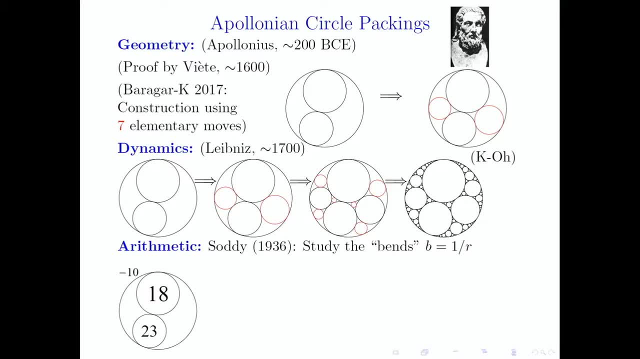 reciprocal of radius squared. So if we have a configuration where the first circles have curvature or bend, 18,, 23, and well, this outer circle has radius 1 tenth, but we want the orientation to be opposite because it's internally tangent, so we'll call that negative 10.. 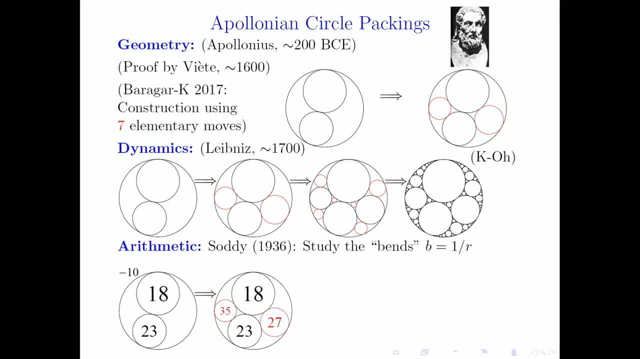 When we do this first operation, this straight edge and compass move, with seven elementary moves, the next circles will have radius 1 over 35 and 1 over 27, and more and more come in and it turns out that they're all integers. 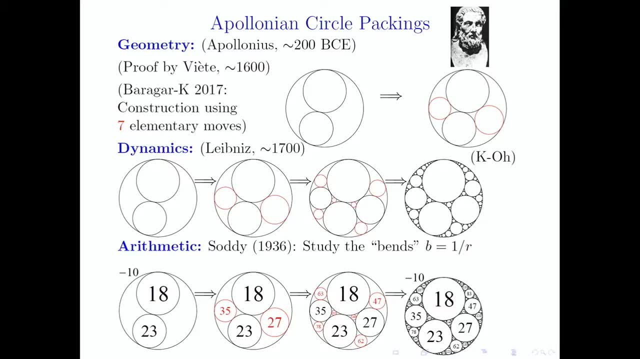 So that's the story of integer, Apollonian circle packings, And, of course, the next question you should ask is what integers arise- and that's something that many people worked on, including work of Bergan and myself, to prove almost local, global. 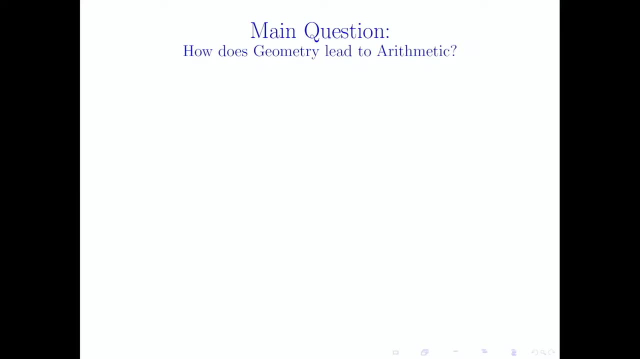 Okay, so that's all very old news. I'm not going to say anything more about that. but the question I became interested in is: okay, there are all these kind of miracles, this. why do these things exist? That's kind of the question I wanted to try to understand. 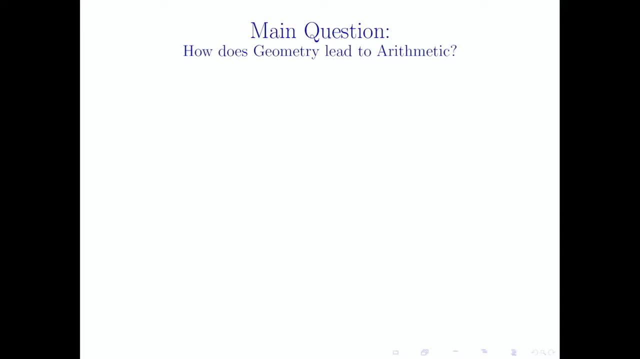 So how does the geometry of the Apollonian construction lead to the arithmetic discovered by Sade? So let's look at this again. So the geometry and the dynamics: well, the packing is generated by dual circles, by reflections through dual circles. 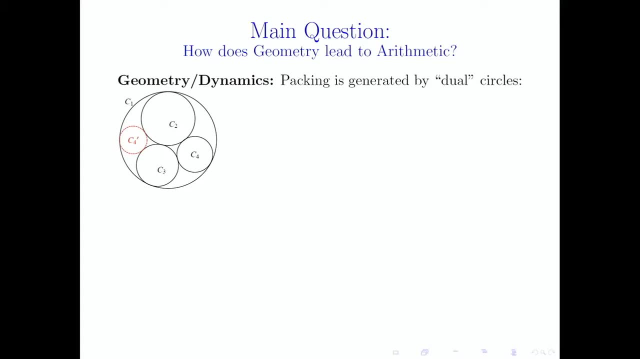 So what do I mean by that? Let's take C1,, C2, and C3 as our initial three circles. They have three points of tangency. Those three points determine a circle. Let's call that circle C4 dual. And then the observation is that if you reflect the image through C4 dual, it fixes C1,, C2,. 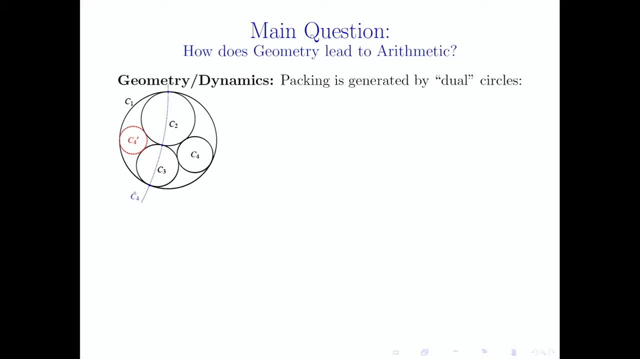 and C3, but sends C4 to C4 prime, the other solution to the Apollonian problem. So these two are dual to one another. And so if you look at C1,, C2.. C3, and C4, now you have a number of dual circles, in fact four. 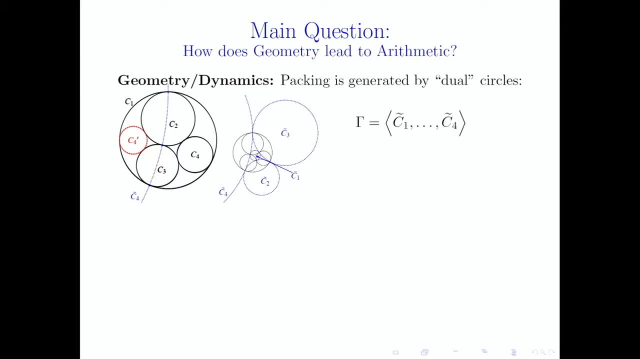 And if you take the group generated by reflections through those four circles and you start moving the initial circles, you get the entire packing And the key idea here, if you want to study this operation, the dynamics, the idea of Poincaré, is to give yourself some complex analysis. 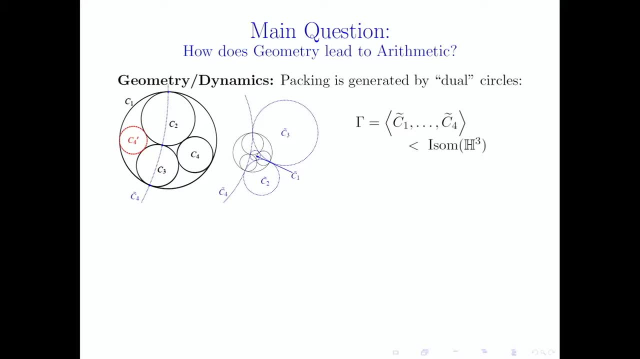 Move away from the plane into the upper half space. So think of this group not as acting in the plane, but as acting in hyperbolic space, so as a reflection group of isometries. So then the picture you see. I don't know if you can see this in the back, but it's the same circle. 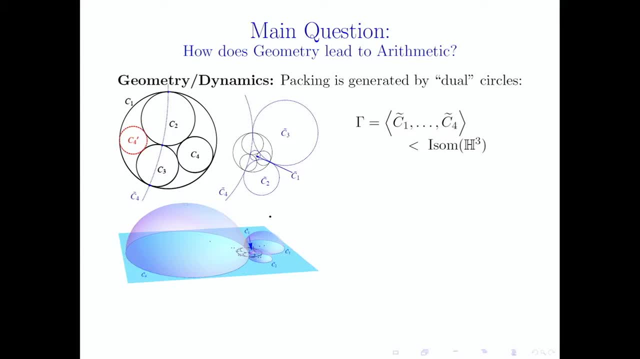 C1, C2, C3, C4, dual. So these are the dual circles, And what's being shown here is an orbit of a single point in upper half space under reflection. So the reflection through C4 brings it here, and then reflections through C2 there and so on. 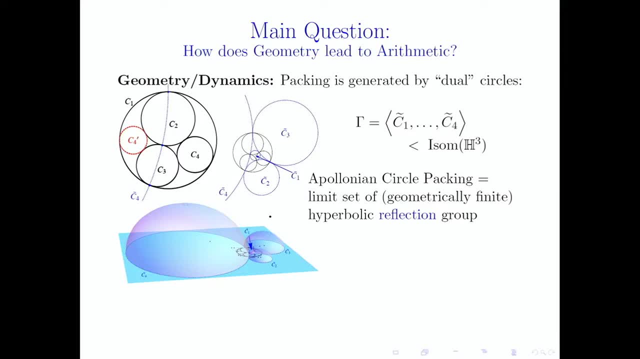 And I hope you can see that the limit set, the limit set of this hyperbolic reflection group is this: It's Apollonian circle packing. So that's another way to realize this object And that's very important for studying both the dynamics and the arithmetic properties. 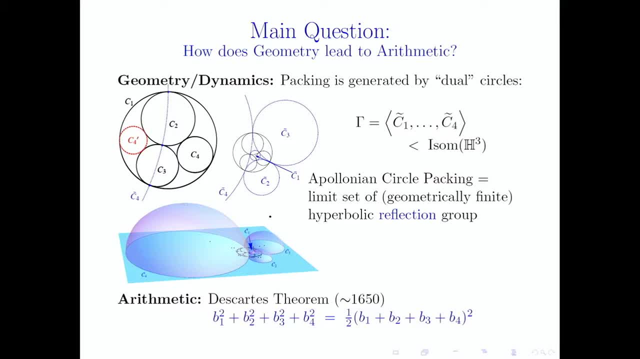 And where does the arithmetic come from? Well, it comes from an old theorem of Descartes that if you have four mutually tangent circles with bends B1 through B4, then they satisfy this nice algebraic relation. And although Descartes proved this and many people followed Descartes and understood his proof, 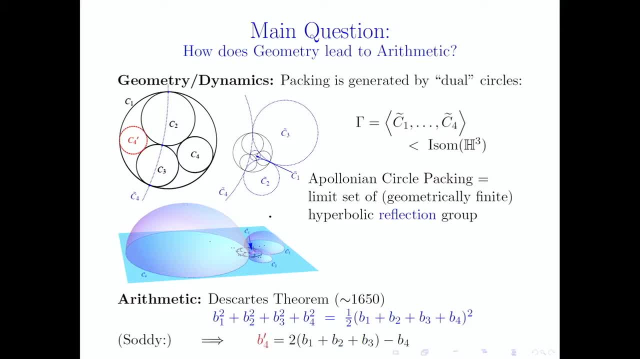 and appreciated it. somehow, none of them took the next step Until Sadi, which is, if you have B1, B2, and B3, then you have a quadratic equation in B4. So there are two solutions. Those are the two possible circles to place there. 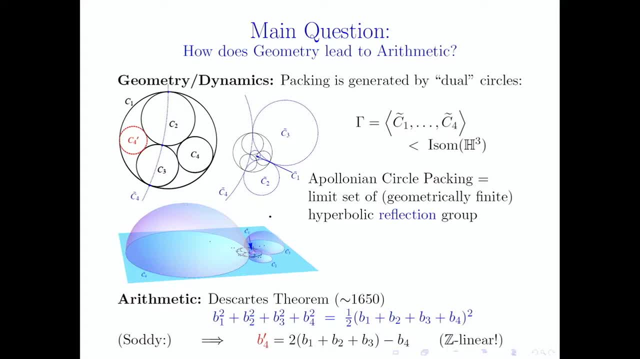 And one is related to the other by an integer linear combination of the previous curvatures. So it turns out that, if so, that's where the integrality is coming from. If the initial four tangent circles have all integer bends, then forever you'll have integer bends. 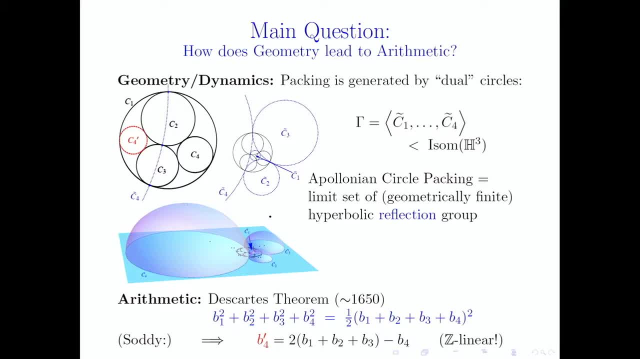 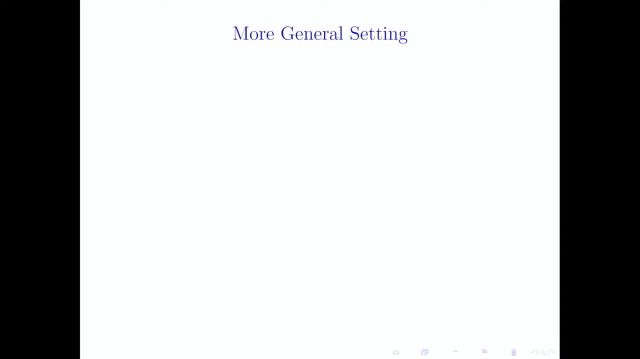 because the bends are linear combination, integer linear combinations of previous. Okay, so that's what's going on in the Apollonian packing, So what's happening more generally. So there are a lot of other- well, not a lot- a handful of other examples. 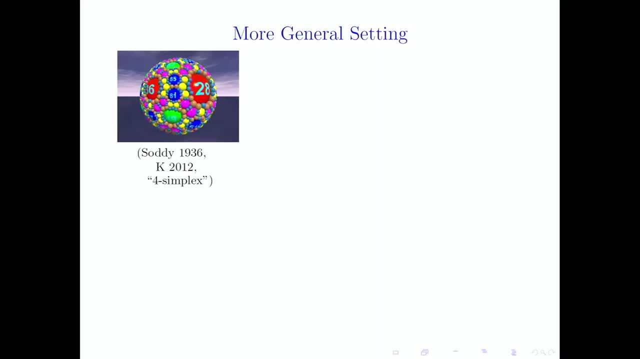 For example, Sadi already studied the sphere packing, the integer sphere packing, which I call the Sadi packing, And I studied the local, global problem in this context. So today we would call this the four simplex. I'll explain where this terminology is coming from. 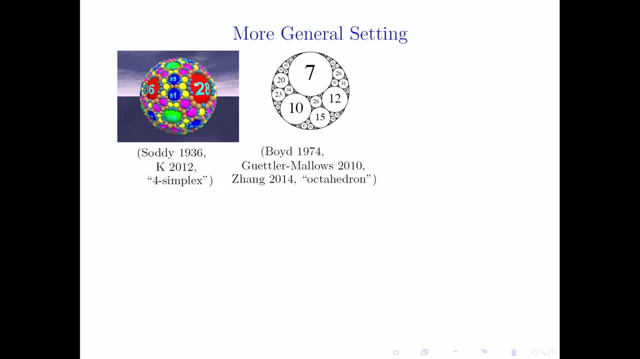 There's a very old paper of Boyd's- in 74,- which I only recently published but I recently discovered has a construction that until now I'd been attributing to Guttler-Mallows, And this is what my student Xin Zhang worked on for his thesis. 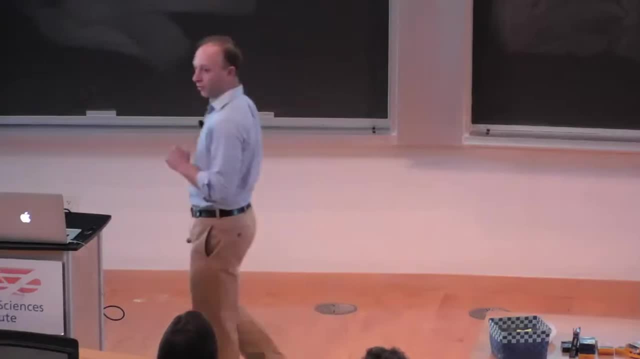 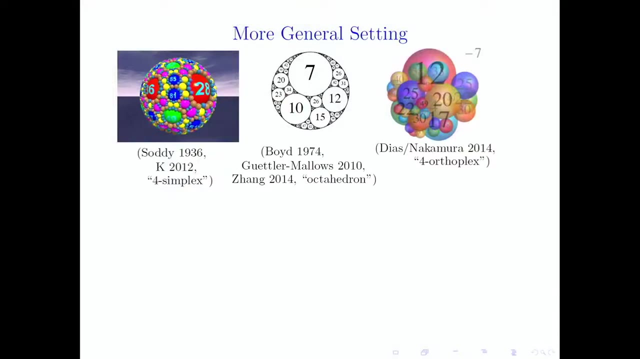 proving the analog of my theorem with Bergan, this almost local, global theorem for these packings. And then the analog of the Sadi theorem was worked out by Diaz and Nakamura for the four orthoplex. So there's some other sphere packings. 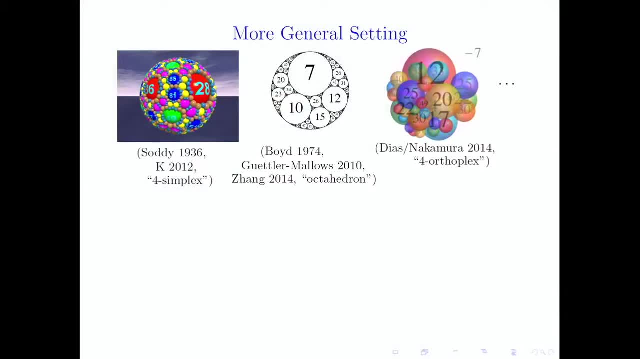 There are a few other examples, notably by Kate Stange and others, by Arthur Baragar and others. So what will I? what's the setting, What's the game I want to play? So I will call a packing of Rn. A packing is an infinite collection of n minus 1 spheres. 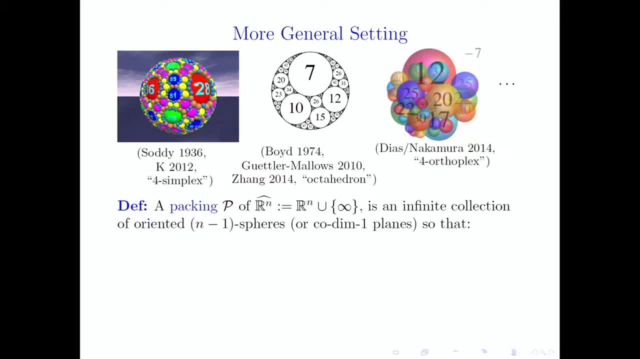 I will want them oriented. So there's a direction. Which way will we call inside? And of course, limits of spheres are okay. So that's planes, hyperplanes, And I will want it to be a packing, So the interiors of the spheres should be disjoint. 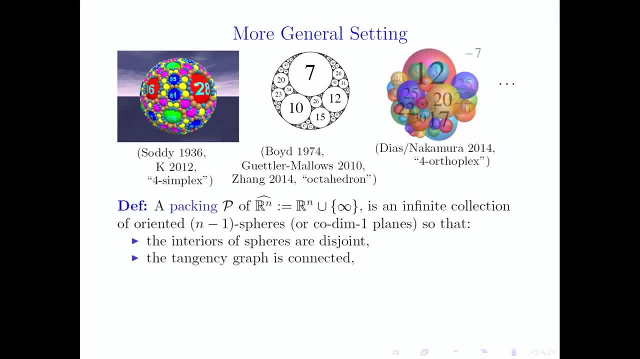 And again, I will want it to be a packing which, to me, says that the tangency graph is connected. Okay, so the spheres are touching each other, And I will want it to be a packing, I want it to fill up all of space. 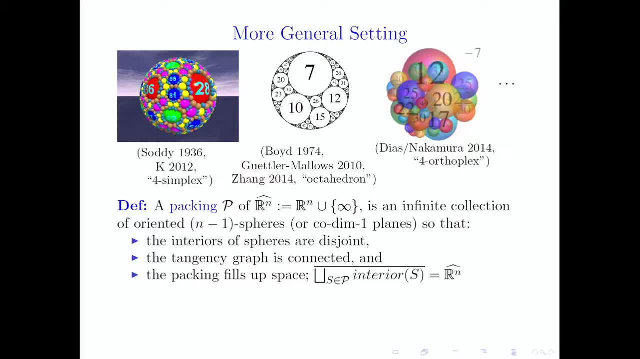 So if you take the interiors of all the spheres and you take the union of those, and the closure should be all of space. Okay, so there's no ball missing from space that's not intersecting at least some sphere. Okay, so this is again unequal packing of spheres, not to be confused with the recent work on E8.. 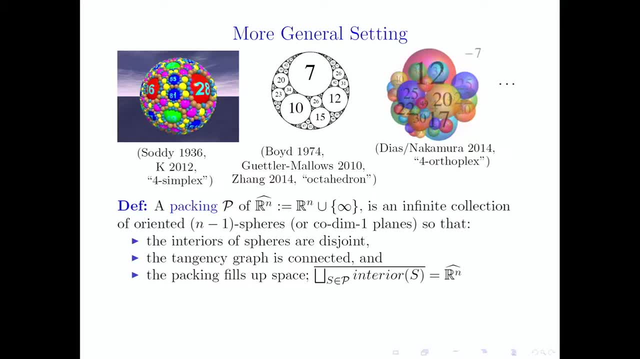 And 24 dimensions. So this is. you see the picture. Okay, so that's what a packing is. Now, as stated, there's no structure, Right? You just arbitrarily make your favorite collection of spheres that just touch and you know. wherever you have space, you stick another sphere in and there's a packing. 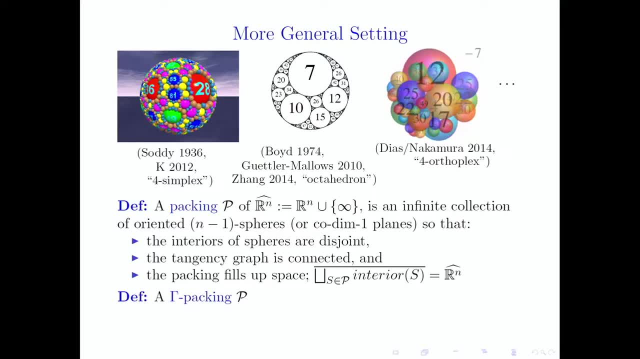 So we need some structure to study this, And the structure I will want is the one that we have for the Apollonian group, namely hyperbolic reflection groups. So I will say a gamma packing is a packing Which Arises at the limit set of some geometrically finite hyperbolic reflection group. 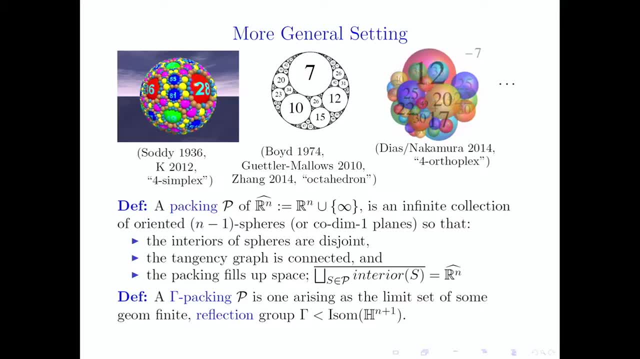 So this is a group acting on isometries on hyperbolic n plus 1 space, As we had, if you saw the initial picture. so we have circles in the plane And you'll very quickly see why I need the computer to draw pictures for me. 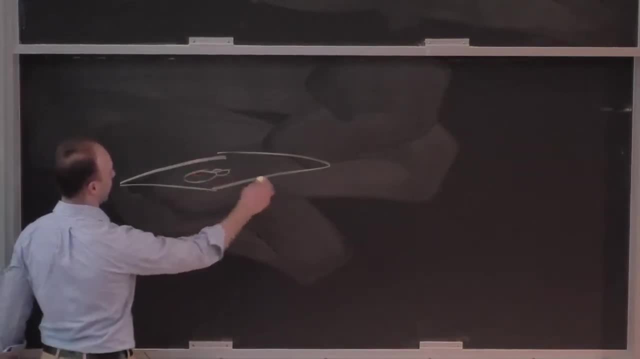 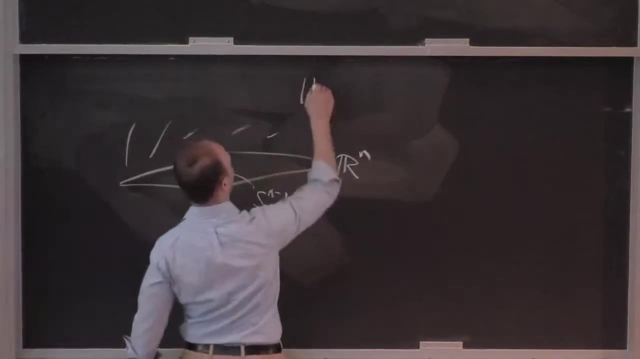 We have circles in the plane and the right thing to think of. so this is Rn And the circles are spherical, So the spheres are Sn minus 1s, But the action is actually taking place in hyperbolic n plus 1 space. 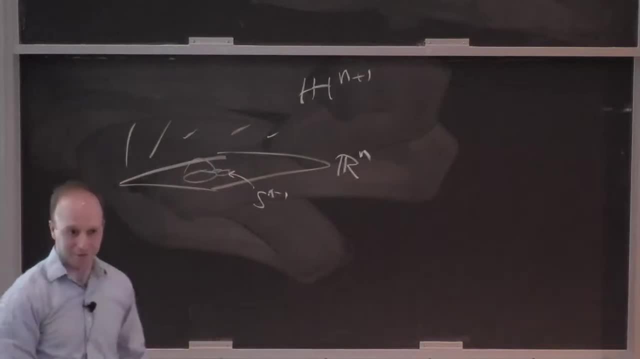 Okay, So that's this inversion through these spheres. Okay, So is that clear? Any questions on the game that I want to play? So this is what I want a gamma packing to be Geometrically, what you're really giving me is not just the packing, but you're also giving me a symmetry group gamma. 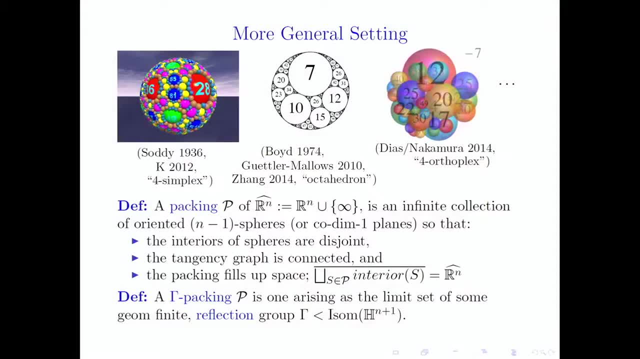 Which, of course, will fix the packing, since, Since it's geometrically finite, it's not a packing. Since it's geometrically finite, it's not a packing. Since it's geometrically finite, it's not a packing. Since it's geometrically finite, it's automatically finitely generated. 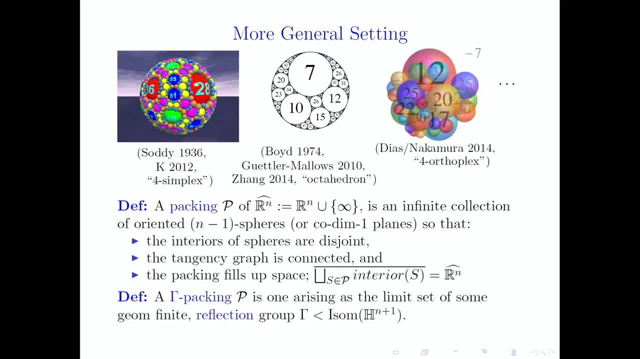 So is it a Zariski dense? I haven't specified that it's a Zariski dense in the definition, But actually it has to be Zariski dense for the packing to fill up all of space. Oh, Any other questions? 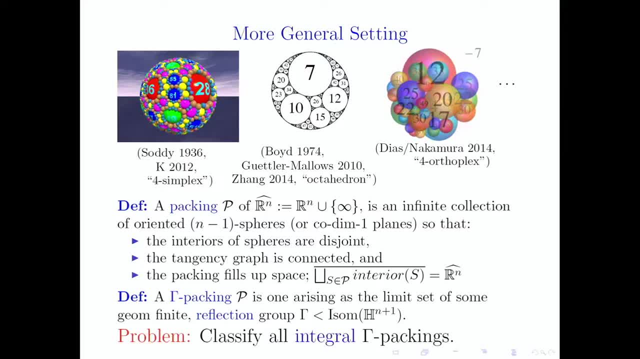 Okay. So of course, the problem then is to classify integral gamma packings, Or so I thought, And it turns out that's not the right problem, And I'll explain why. So Let me explain the notion of superintegrality. So 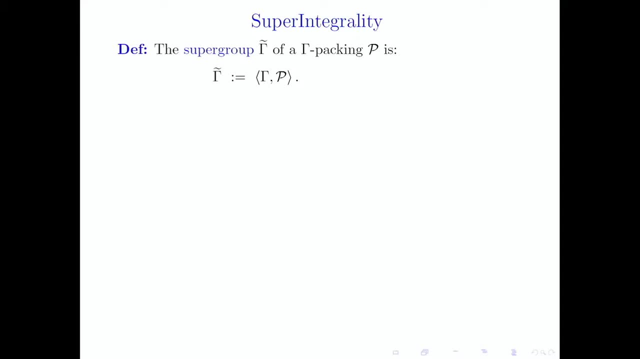 What is a supergroup? Let me explain. So what you do is you're given, Someone gives you- a gamma packing. That means you have the packing and the group acting on it. So the supergroup is the group which is generated by the original group. 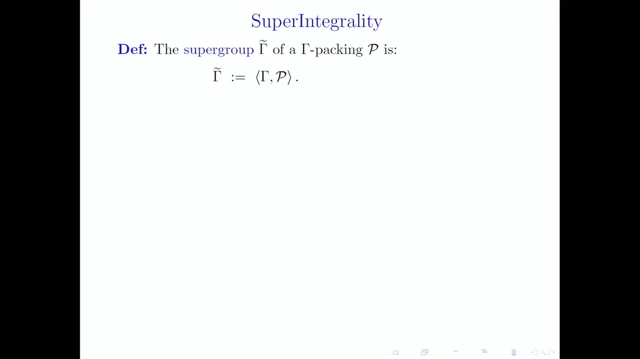 And also inversions through all the spheres in the packing itself. So let's just see an example of that. Here's an Apollonian packing, a strip packing, And the group is the group generated by these four reflections, That's gamma. 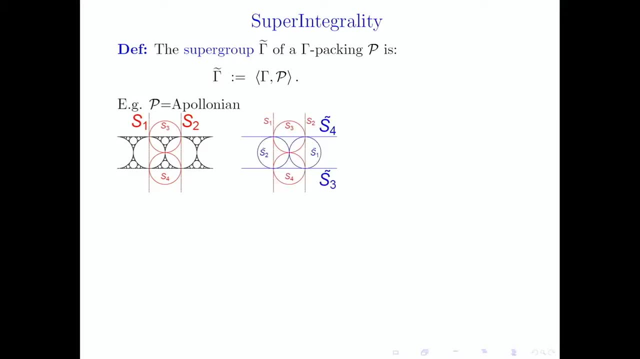 So what's gamma twiddle? Gamma twiddle is the group generated by all the reflections of all these circles, And it turns out it's enough to take the four blue circles reflections through those four in addition to the red ones. Is that clear? 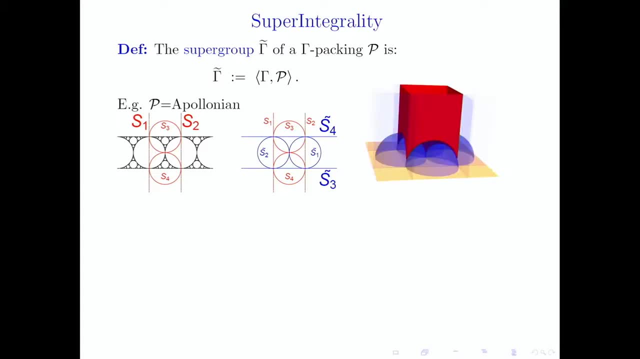 So if you look at this, so this is acting again in the plane. What you should really be looking at is its action in hyperbolic space, And then what you get is a fundamental domain. So the Apollonian supergroup has fundamental domain, which is: 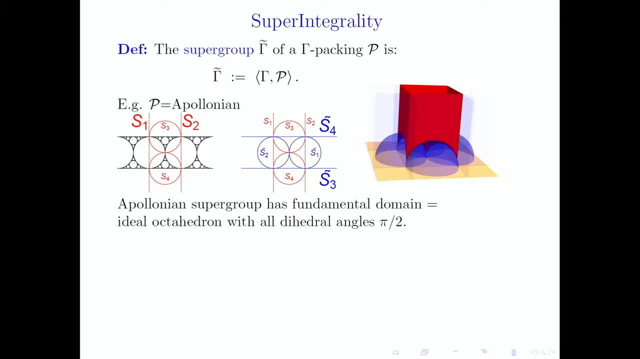 if you work it out, it's an ideal octahedron with all dihedral angles pi over two, And a hint as to what's going on is that that should be reminiscent of something. so this supergroup is commensurate with the Picard group. 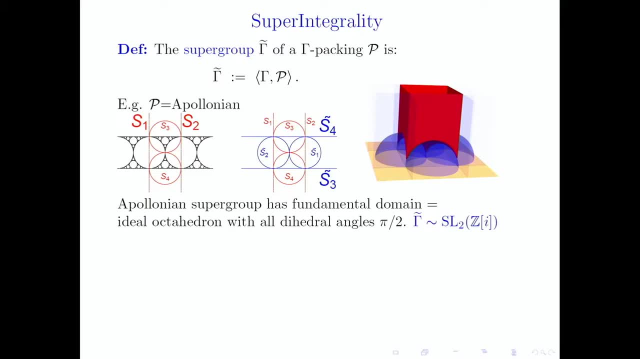 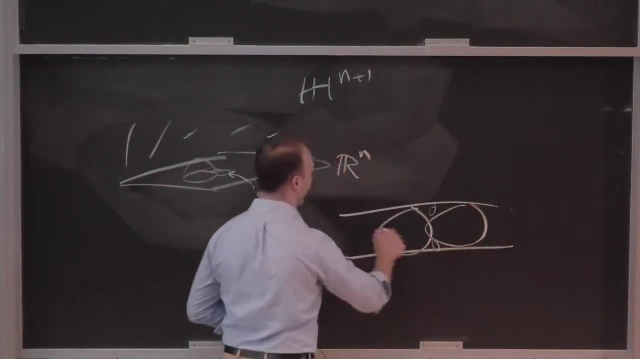 SL2 of the Gaussian integers. So is it clear what I mean by a supergroup. P is a packing, So P is your Apollonian packing. say, Okay, The whole thing, although I won't need anything more of it. 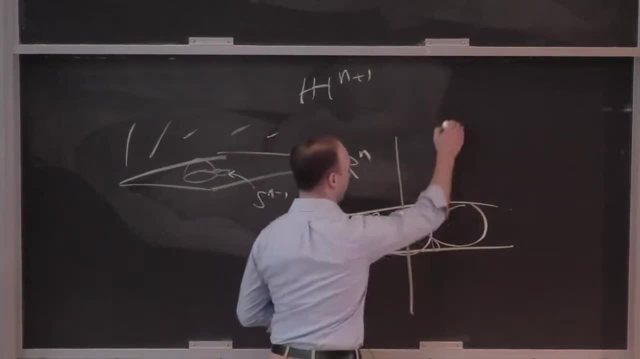 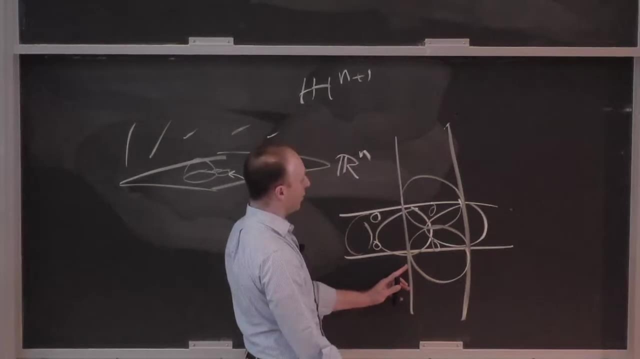 And then you have this: You have the group gamma, which is the group of reflections. So that's generated by these four circles. And now what I want to take is the group generated by all the reflections. So I want to reflect not just through these four. 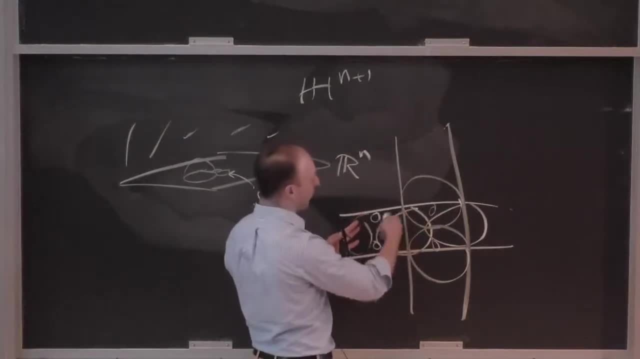 but also through this one and that one and that one and all of them, And it turns out it's enough to reflect just through four more, which are the dual four. Is the picture clear? Okay, Yes, So that's the whole point of having a geometrically finite group. 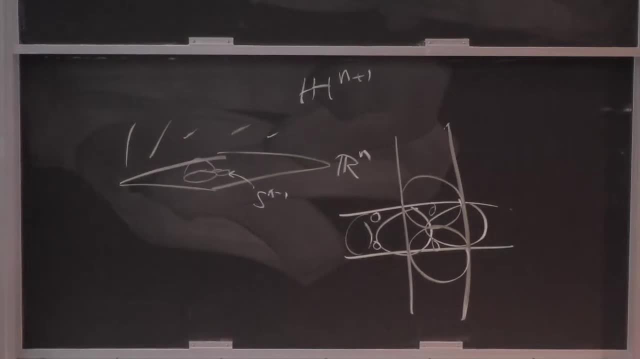 is that being geometrically finite and thin means you have flares And those flares, because the limit set is the exterior of some spheres. you have these regions at infinity that are cut off by spheres, and there's a finite number of them. 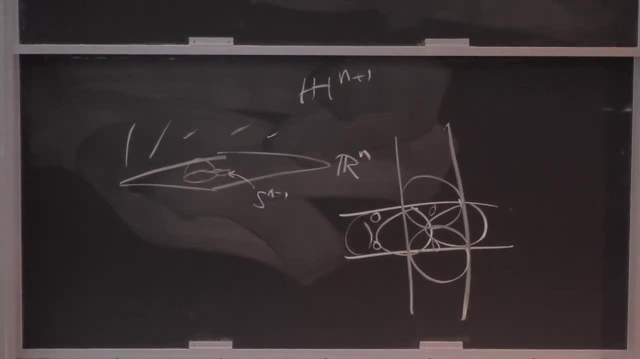 So there will always be only a finite number of circles from the packing that I need to take to generate this thing. So this will be a finitely generated group and, moreover, it'll be a lattice, Since now we've cut off all the boundary at infinity. 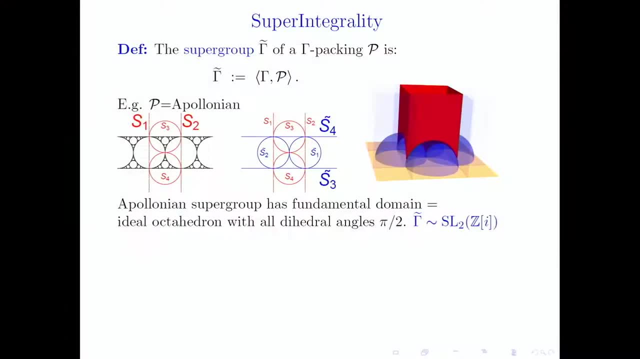 all that's left is cusps. Okay, so this will certainly be a lattice. and that's this group, the supergroup. Okay, So supergroup is okay. Once we have the supergroup, what I want to define is the superpacking. 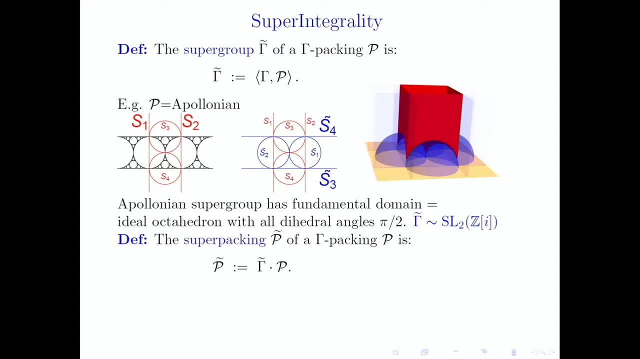 which will not be a packing. but what I mean by that is, you take the supergroup and you act on the packing itself. So what does that look like in the Apollonian case? Well, this is the superpacking. In other words, you start with the Apollonian group itself. 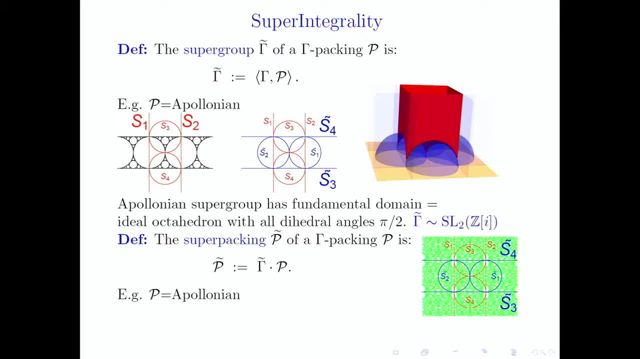 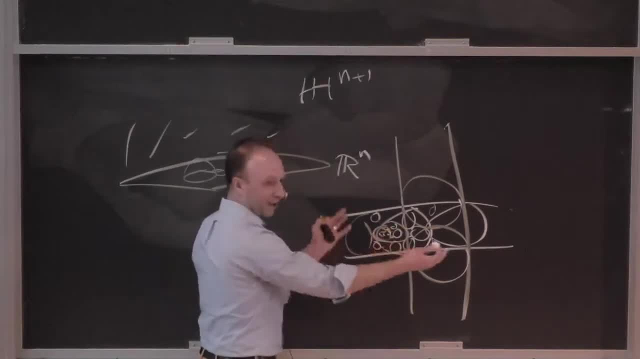 but now you're allowed to reflect through this circle also. So these circles go here, and these circles go here and there and so on. So you get this infinite collection. It's no longer a packing. It's now dense because it's a Bianchi group acting on the plane. 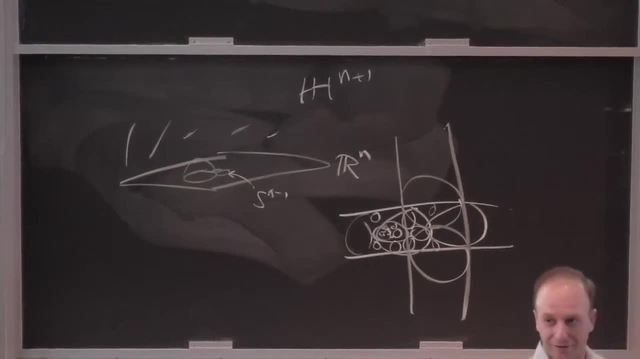 acting on the boundary at infinity. Okay, Is that clear? Is the notion of superpacking clear? So it's like infinitely many packings superimposed on each other. It's infinitely many packings all superimposed. I guess it's too. I put too many circles in. 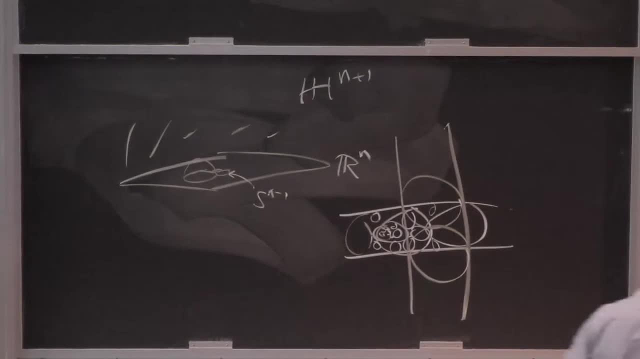 Now you can't see anything. So maybe in this case the hand picture is better than the computer. but yeah, I was hoping for a bigger. okay, I guess someone's taking notes or maybe they'll post this on. maybe I'll post these notes online. 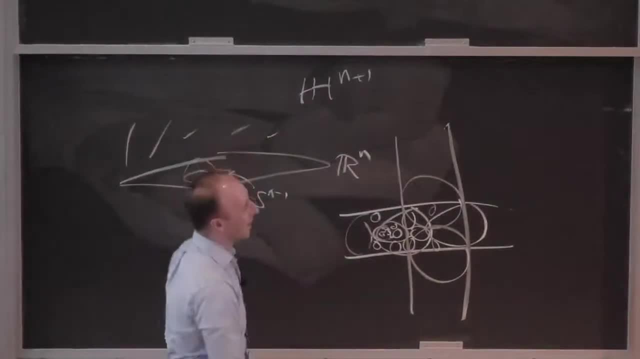 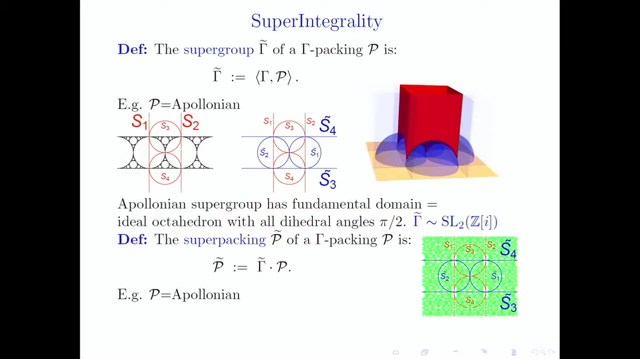 You can zoom in as much as you want, because the picture really does look like this: Okay, So superpacking is okay. Supergroup acts on the packing to give the superpacking. So what does it mean to be superintegral? A gamma packing P is called superintegral. 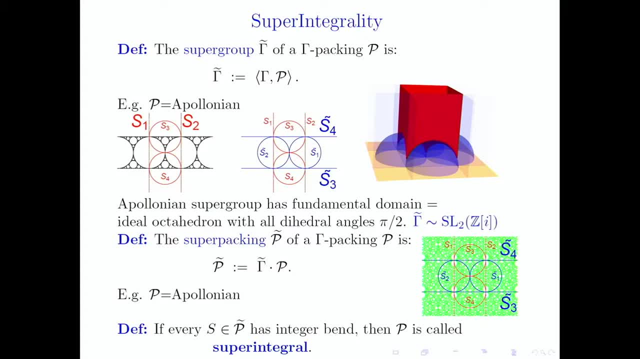 if every sphere in the superpacking has integer bend. So it's not enough to have integer bends in the packing itself, You must have. for superintegrality, you must have integer bends in the entire superpacking. So far, so good. And it turns out that the Apollonian group is indeed superintegral. 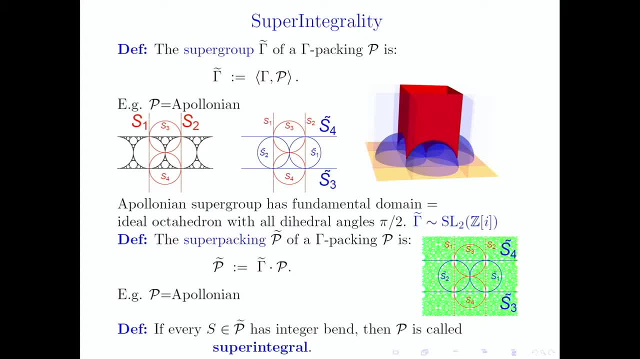 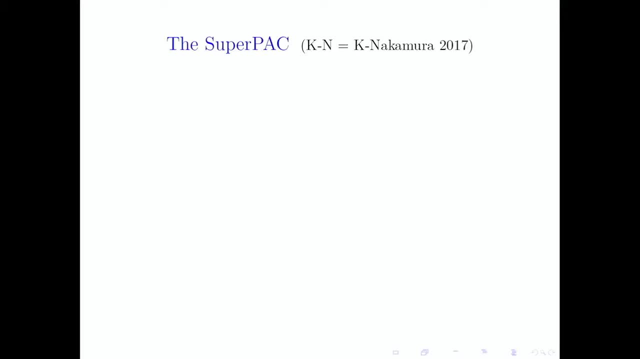 The Apollonian packing is superintegral. Okay, Why do I want that? Because now I can state the superpack. I guess it was the election. So this is, I should have said, joint work with K Nakamura. So our conjecture is the superintegral packing- arithmeticity conjecture. 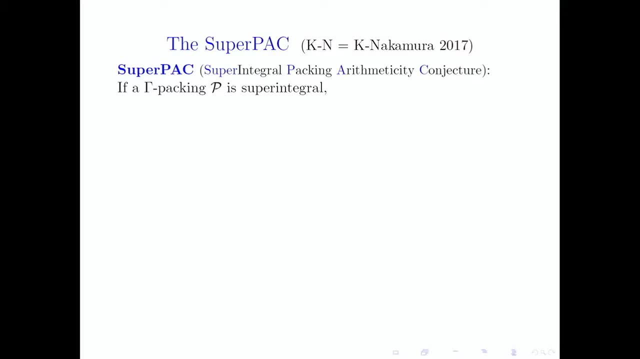 which has the following: If you have a gamma packing P and it's superintegral, then the supergroup, which is a lattice, is actually arithmetic. Okay, That's the main conjecture that I want to highlight and discuss what we can say towards this. 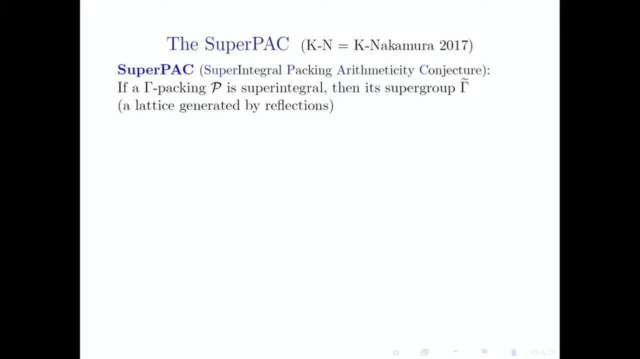 Any questions on the statement? So in the Apollonian case, the supergroup was this fundamental domain, you know, with octahedral, with all dihedral angles, pi over two, And it was commensurate with SL2Z. 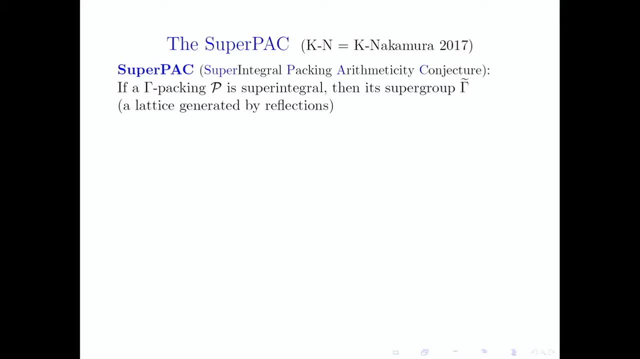 So it was indeed arithmetic. SL2Z is your joint I, Okay. Oh, I was missing a word, That's why you're confused. Is arithmetic? Okay, So this supergroup gamma, which is a lattice generated by reflections, is arithmetic. 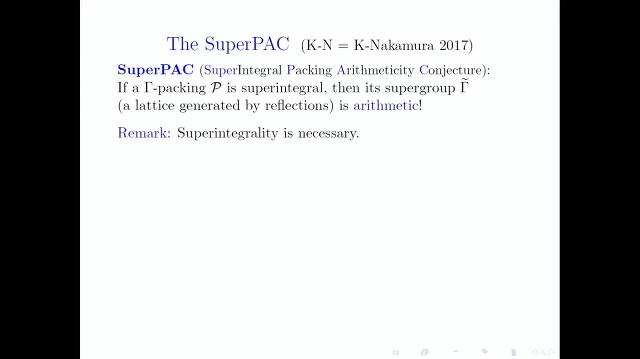 Okay, So let me immediately remark that superintegrality is necessary. So we have. we have examples of integer gamma packings, which are not arithmetic, And I hope to show you that at the at the end, For which the so integer gamma packings. 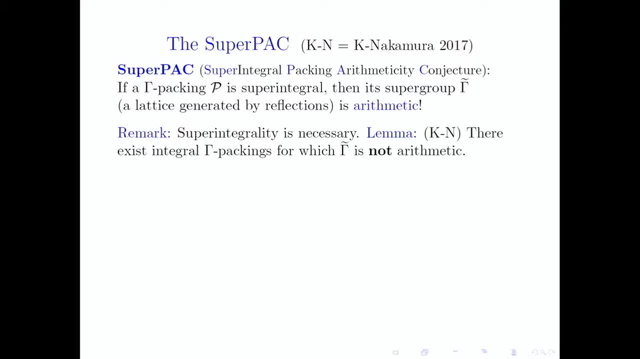 not superintegral, obviously, otherwise we wouldn't be making the conjecture for which the supergroup is not arithmetic And this is somehow related to examples of Deligne-Mostow of non-arithmetic groups. I'll say that later, Okay. 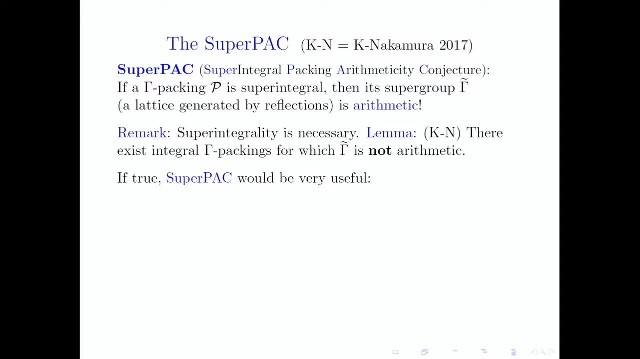 So why do I care about superpack? Well, if we could prove this conjecture, it would be extremely useful for the following reason: There are only finitely many maximal hyperbolic arithmetic reflection groups, So this is a work of many people. 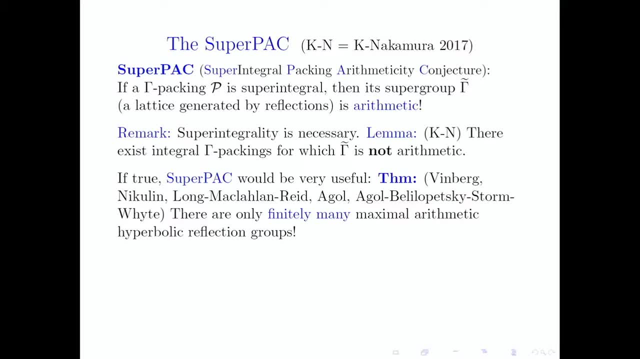 starting, of course, with groundbreaking work of Vinberg, and then Nikulin, and and and many others. So there's a finite list. So if, if you want to, if you, if you think this Apollonian packing was this kind of magical object, 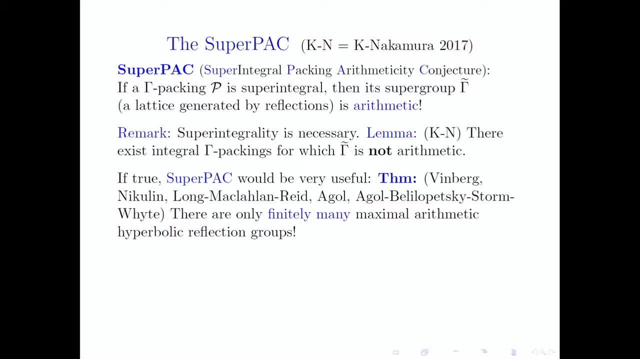 yes, it is magical because it only happens finitely many more times. That's what this conjecture would say, And in fact we know that there. so there, there's a finite number in each dimension and there's a bound on the dimension where 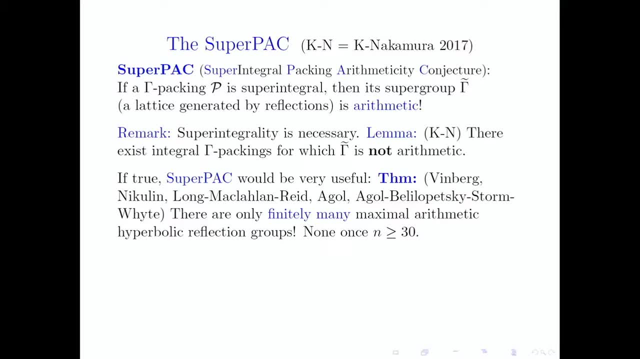 where these arise at all. Okay, So so it turns out as, although initially it was stated as a general problem, it turns out it's a finite dimensional topology problem. Okay, Low dimensional, if 30 is low for you, Okay. 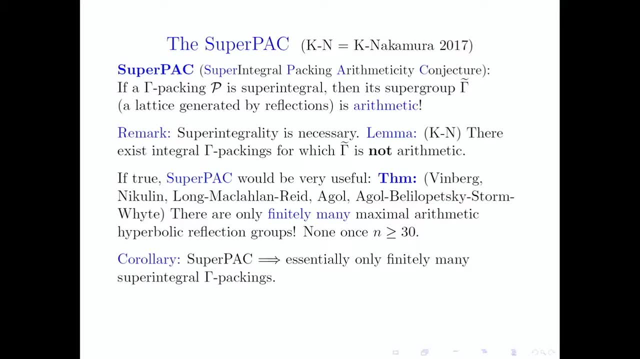 So super pack would tell you that they're essentially only finitely many super integral gamma packings And the theorem that we can prove so far is that the super pack holds for gamma packings- I have to explain what this means: modeled on uniform polyhedra. 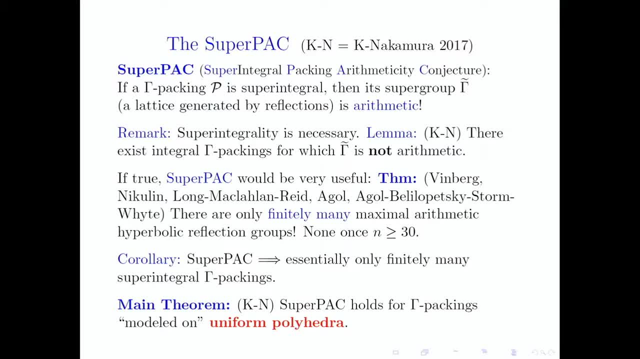 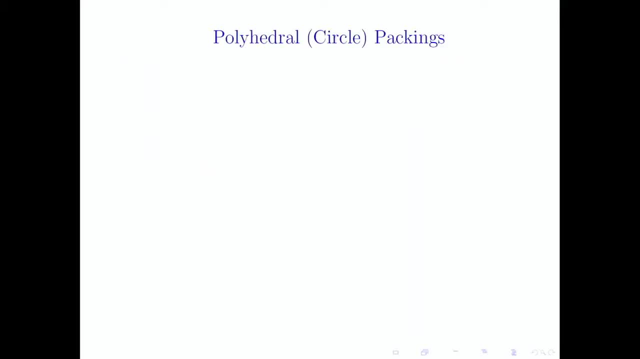 So let me explain what that means. So any questions before the last statement I have to explain, but otherwise is everything clear. Okay, So what is a polyhedral packing? So let me remind you of this fundamental theorem of Kobe Andre of Thurston: 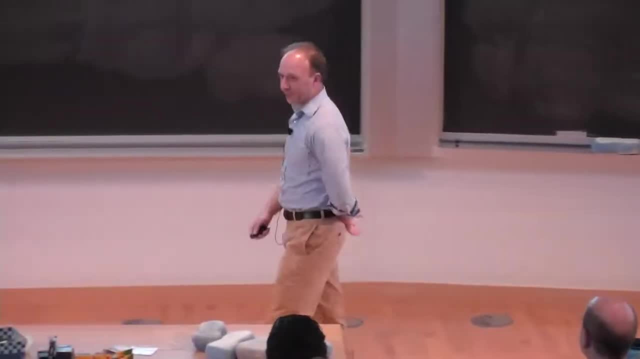 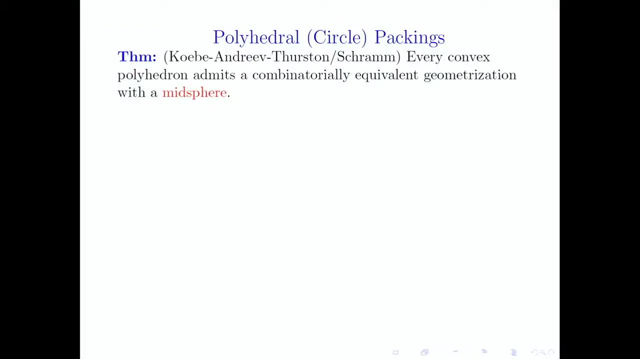 which, in this formulation, was claimed by many people. but the only place where it was actually written down that, or the first place that I saw it written down, was Schramm. So it says the following: every convex polyhedron, so topological polyhedron. 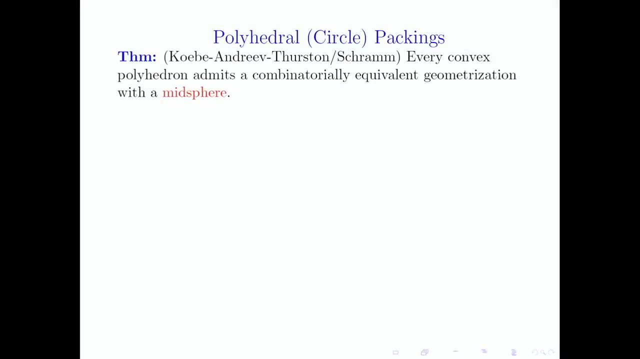 admits a combinatorially equivalent geometrization which has a mid sphere. So what does it mean to be, to have a mid sphere? It means a sphere which is tangent to all the edges. So let me show you an example. So if you don't remember what a cube octahedron is, 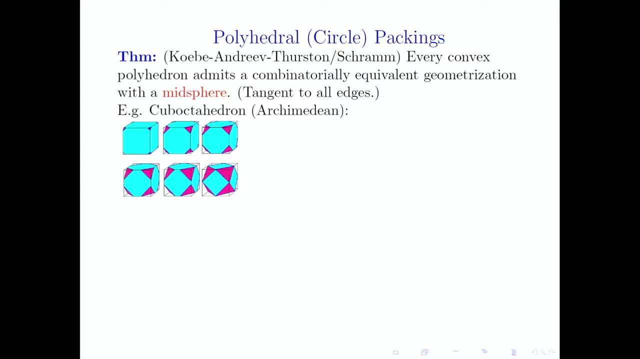 so this is an Archimedean salad. you start with a cube and then you start cutting off the corners. And when you cut off the corners, when you get to this, what is that? an octagon. When you get a regular octagon at the faces. 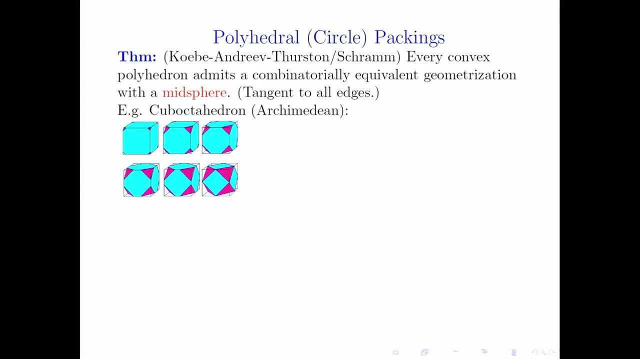 that's called a truncated cube. and you keep truncating a little further until the corners actually meet, and now you get squares again and that's called a cube octahedron, because, if you so, you started with a cube when you did this operation. 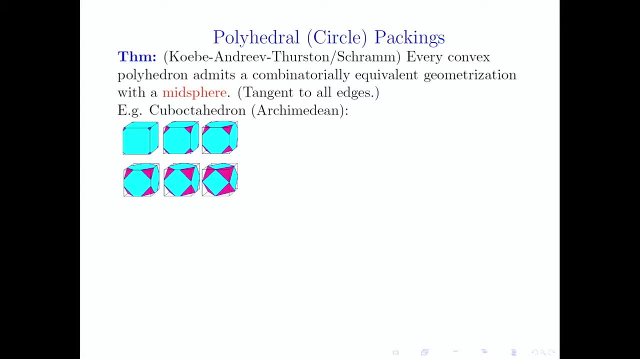 but if you start with an octahedron which is dual to the cube, and you start cutting the corners until you get to the middle, you get the same shape. So that's called a cube octahedron. So topologically, what I mean is: 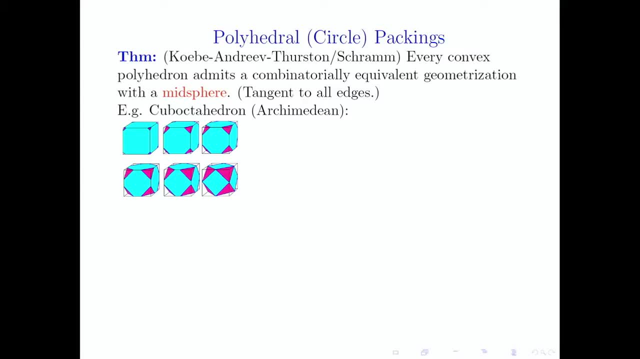 how many vertices do we have? We have four on top, four in the middle and four on bottom. so we have 12 vertices and every vertex has valence four. there are four edges coming out and around every vertex there's a square. 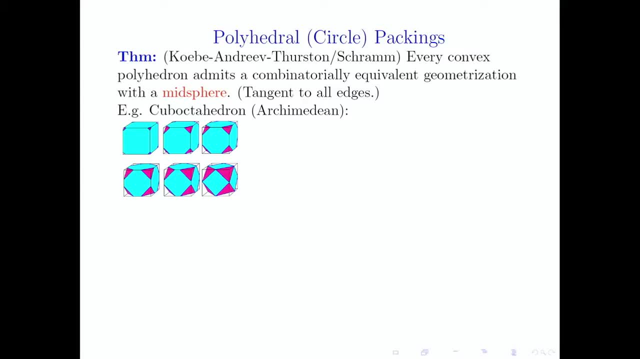 then a triangle, then a square, then a triangle. So that's what makes it an Archimedean salad. Its faces are regular polygons and it's vertex transitive. Every vertex is transitive. Every vertex looks the same. So that's the combinatorial. 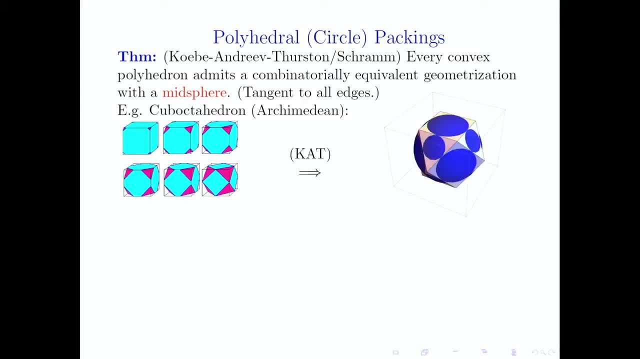 the topological information you are given, and what the Coby-Andrea-Thurston theorem produces is a particular configuration of the vertices in space, such that there's a sphere which is tangent to every single edge. Okay, So I hope you can see the. 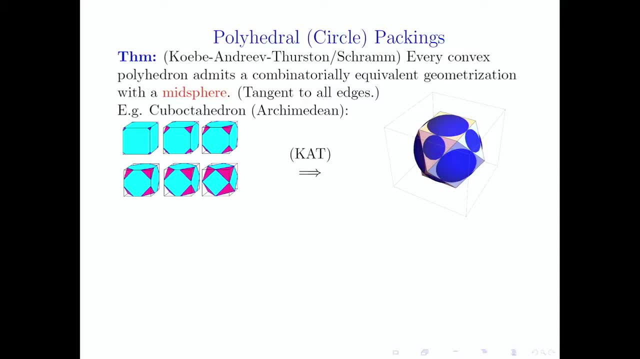 this sphere that blows up and you pull the vertices around in exactly the right way and this is conformally rigid. There's a unique way of out to Mobius transformations of doing this. Okay, They were using this for things like approximations to the conformal mapping theorem. 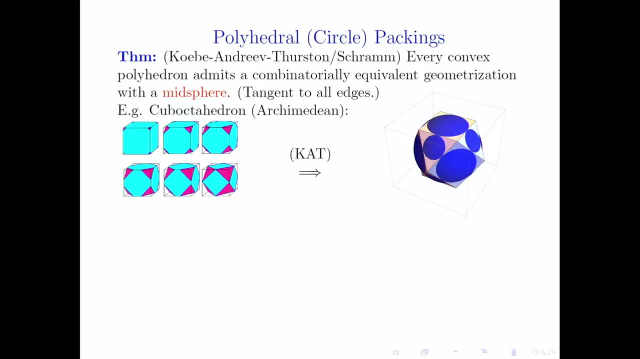 You know doing. it's a beautiful story that I don't have time to get into, But I want to use this for a different purpose. So what I would like to do is to use Coby-Andrea-Thurston to attach. 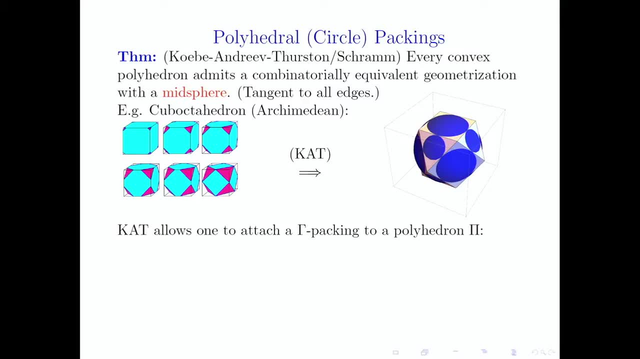 a gamma packing to your favorite polyhedron. You give me a topological polyhedron, I'll hand you back a circle packing. So these are all these circle packings. I probably won't say much about our higher dimensional examples, because it's hard to draw pictures. 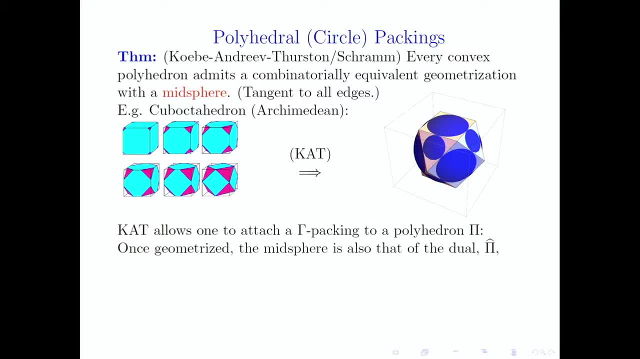 of four-sphere packings. So how do you do this? So once your topological polyhedron is geometrized, the mid-sphere is also the mid-sphere of the dual polyhedron, So the dual of the of the cube octahedron. 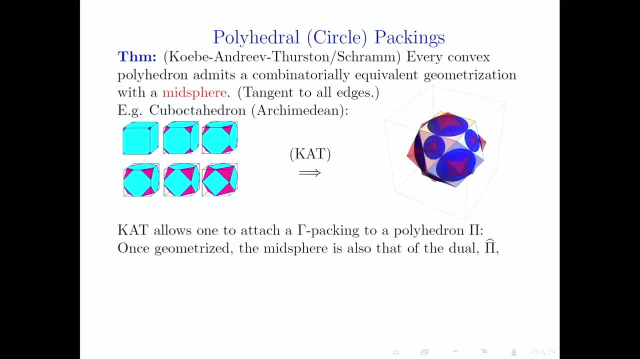 so let me show it to you. You ready, Watch this? There it is. So that's called a rhombic dodecahedron, So every face is a rhombus and there were 12 vertices of the cube octahedron. 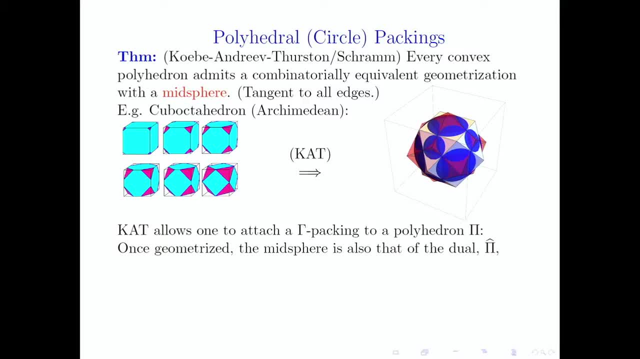 so now there will be 12 faces of the dual polyhedron. So that's a dodecahedron, So it's a rhombic dodecahedron, And you can see that the mid-sphere perfectly chops up these two figures. 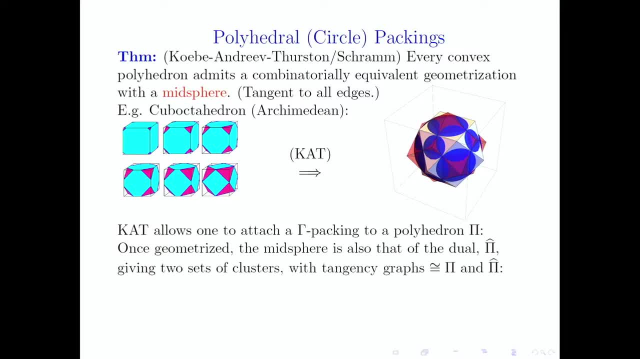 one sitting on top of each other. Okay, so what do you do now? So you get two sets of clusters of circles. So this is a circle which corresponds to that vertex, while this is a dual circle corresponding to this face. So you get circles and dual circles. 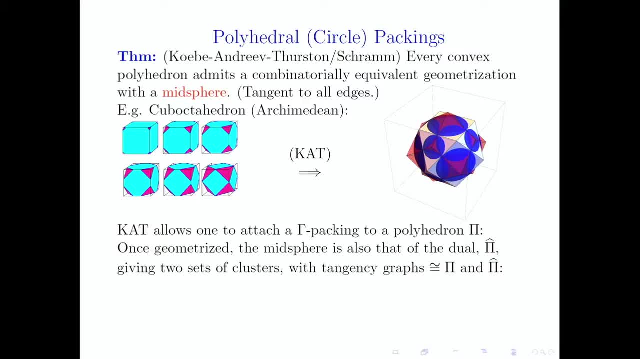 on top of each other, which give you two clusters of circles whose tangency graphs are topologically the same as the original polyhedron and its dual. So let me show you that in this picture here. So this, the blue circles, every circle corresponds to a vertex, right. 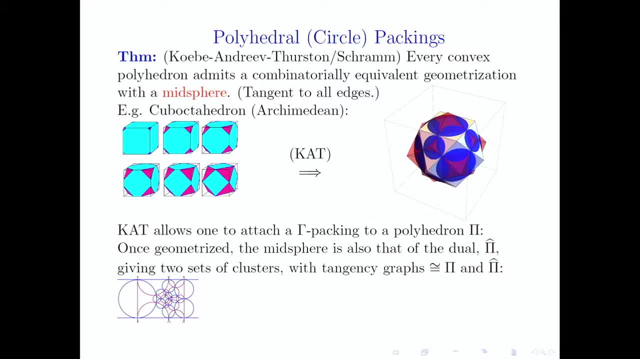 Tangency means the two circles are touching, So the circles are vertices, and an edge between them means they're tangent. So here's a circle. So what you should really see is around this circle. what kind of faces do we have? 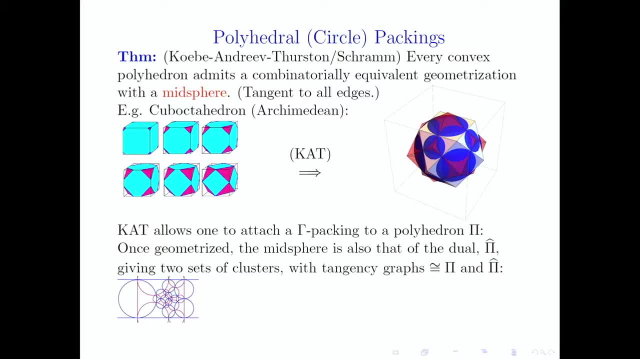 So here's a square face. I hope you can see four sides, And there's three sides and there's four sides, and here there's a triangle, Three sides. So around that vertex is triangle, square, triangle square, just like the cube, octahedron. 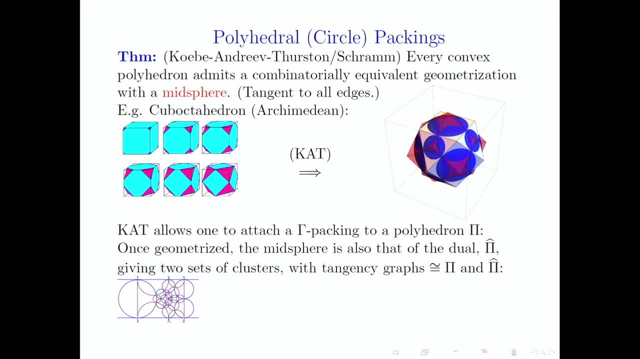 Okay, so the graph, just the tangency graph of the blue cluster, is isomorphic to the original cube octahedron and I'll let you verify that. the tangency graph of the- whatever color that is, red or purple or something. 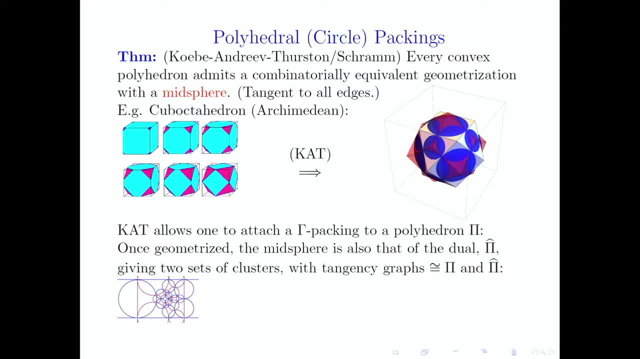 I don't know- is the tangency graph of the rhombic dodecahedron. So is it clear how I'm getting these two clusters sitting on top of each other from Coby and Dre of Thurston. What's a cluster? 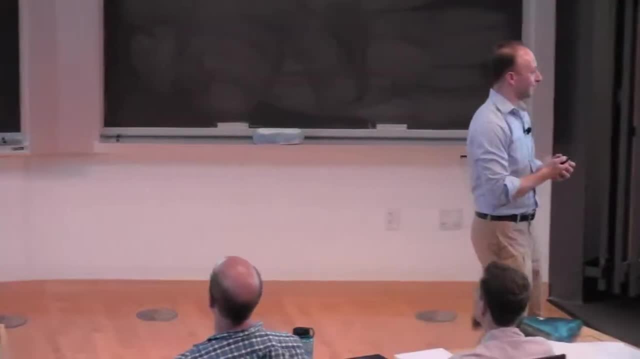 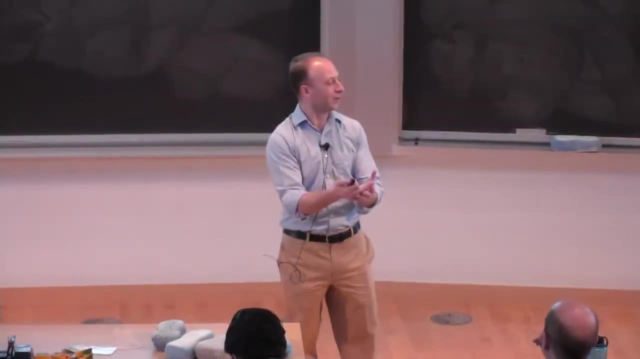 A cluster is just a finite collection of circles. So a finite collection of circles and I, what I want is the tangency graph of that finite collection of circles, to be isomorphic to the polyhedron that you, that you asked for. 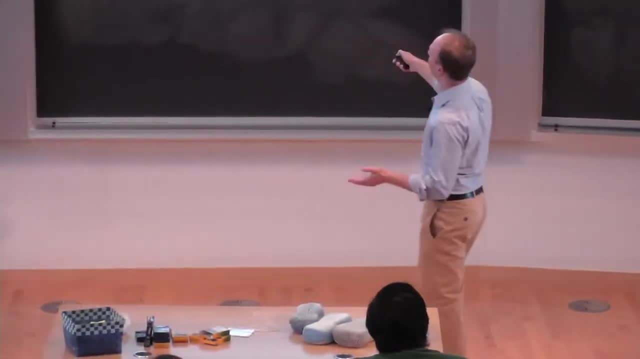 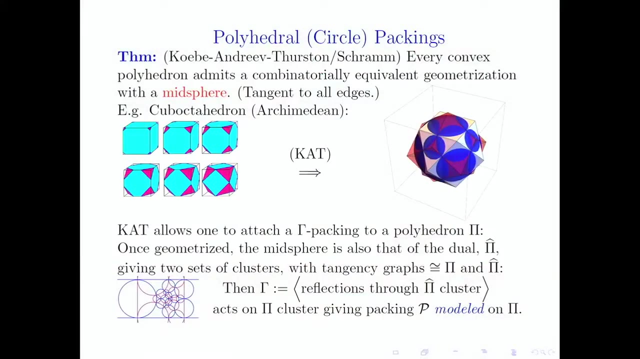 Okay. So once you have this, what do you do? You do the obvious thing: You take reflections through the dual cluster and you let that act on the original cluster and that will give you a packing modeled. what we'll say is that it's modeled. 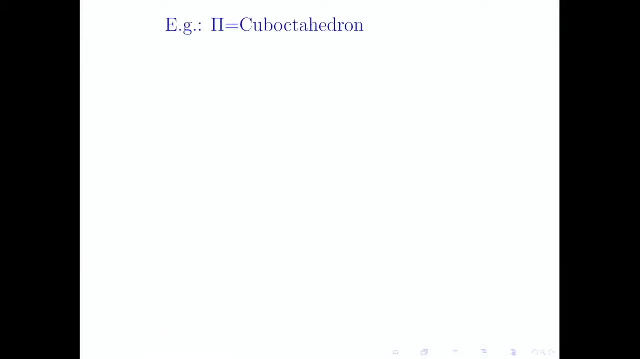 on the given polyhedron. Okay, So let me let's do this cube octahedral example. There's the cube octahedron. again, What you're given is this: communitorics, or the topology, which is the list of vertices. 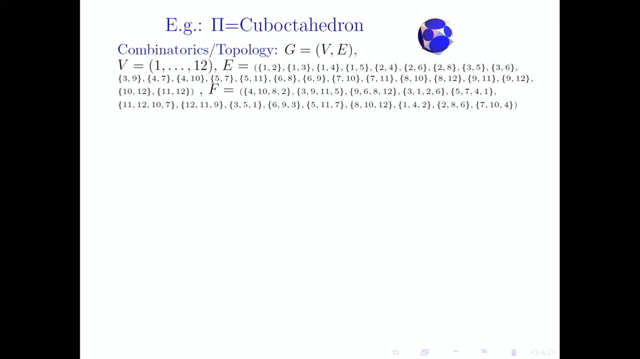 and list of edges from which you could construct a list of faces if you really want to. All we need is the one skeleton. So then you geometrize. Here's Coby and Dre of Thurston. That gives you a cluster again. 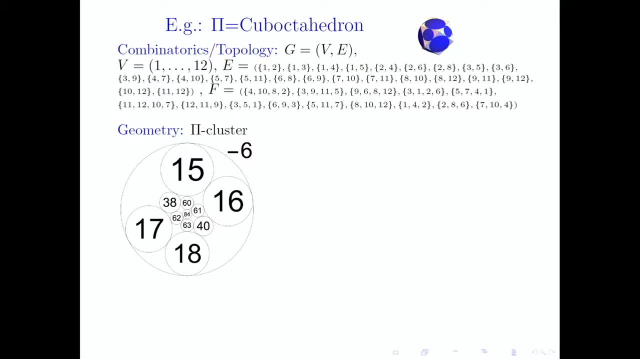 around the circle labeled 17 is a triangle, then a square, then a triangle, then a square. So that's the cube octahedral configuration. That's the same for any circle. And then, when you let the dual group act, you get the packing. 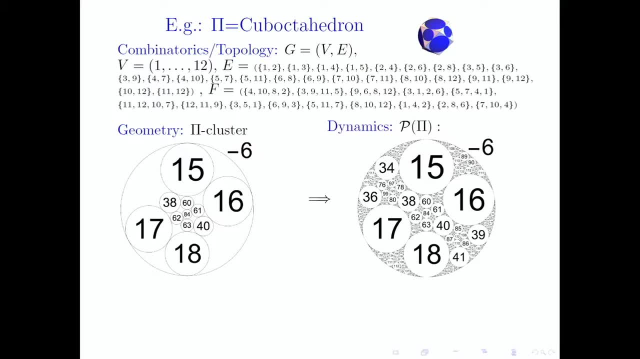 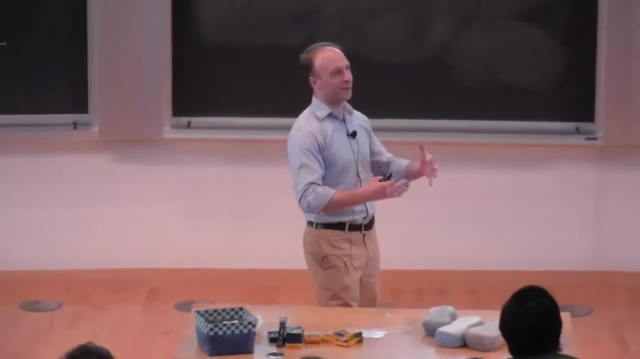 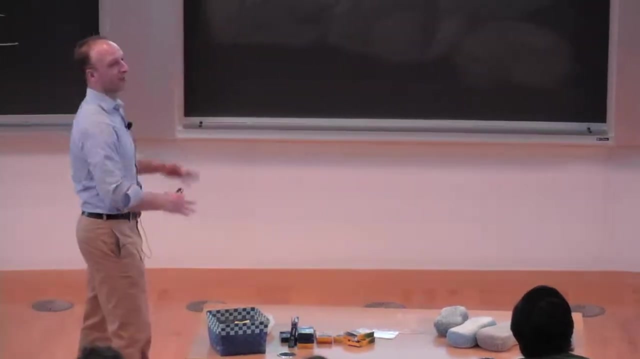 modeled on the cube octahedron. Okay, Is this clear? So the graph: what does it mean to be a combinatorial polyhedron? It means to be a three-connected planar graph. That's an equivalent statement. So these are all planar graphs. 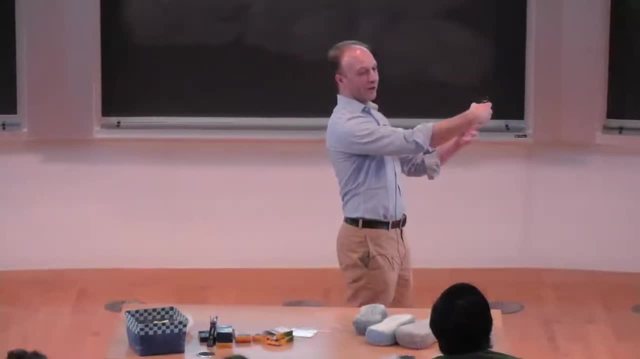 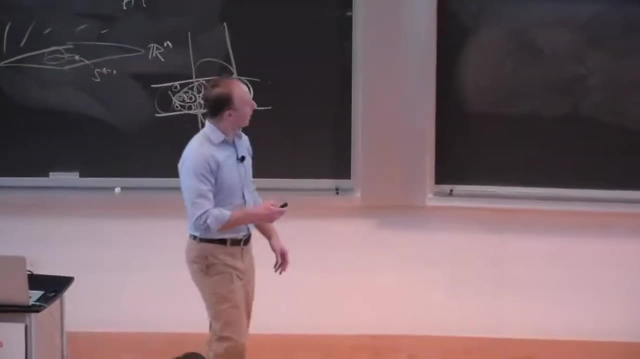 And in higher dimensions we'll need simplices of one dimension higher, If that makes sense. It's similar to what's going on here, this extension, Okay. So is it clear how we let the dynamics of the dual group act and we get this gamma packing? 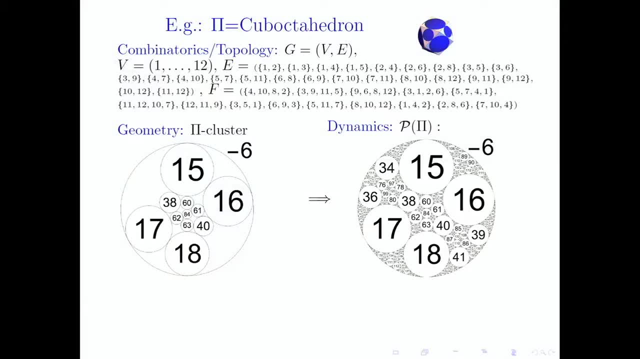 modeled on the cube octahedron And, as you can see, this one's integral. So the cube octahedron is integral And we'll call a polyhedron. we'll extend the definition of superintegrality to the polyhedron, or integrality. 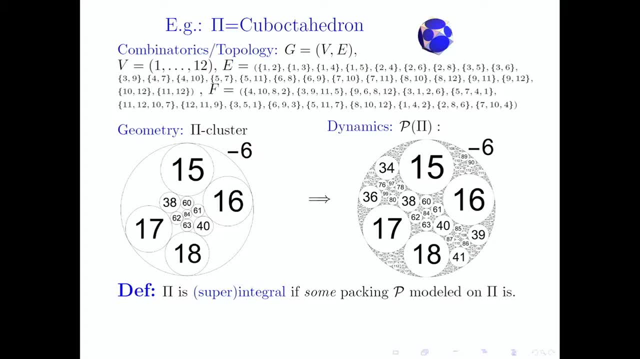 So a polyhedron is superintegral or integral. if there exists some packing modeled on it which is integral or superintegral, Does that make sense? So lemma, the cube octahedron, not only is it integral, as you can see here. 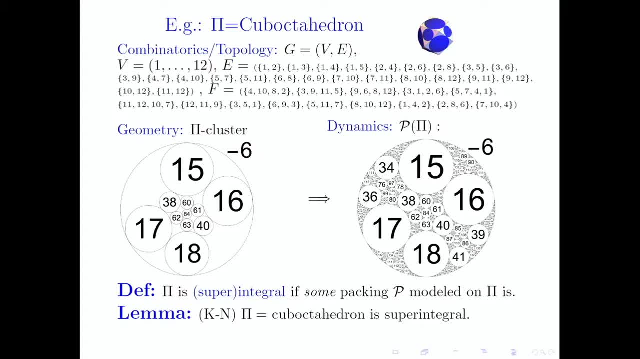 it's actually superintegral. When you take the superpacking, you will also get only integer curvatures, only integer bends. Okay, So the real problem is: classify superintegral gamma packings and a subclass of them is classify superintegral polyhedra. 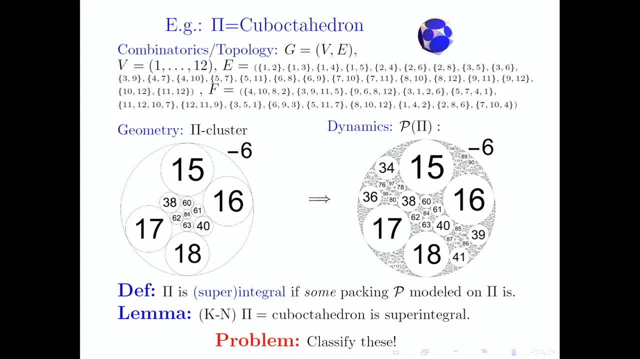 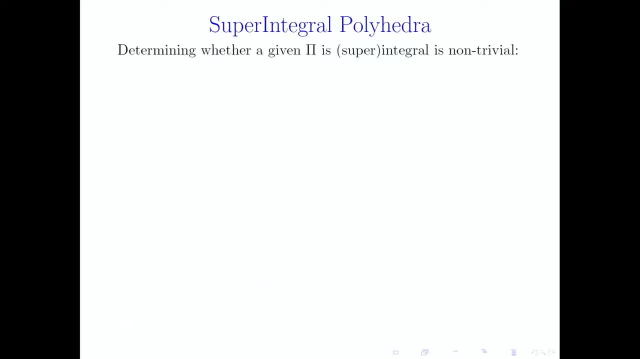 Which polyhedra are superintegral. And again, the conjecture is there's essentially finitely many. So lemme explain why this is not so easy. So first of all, if I give you an arbitrary polyhedron, I give you a three connected planar graph. 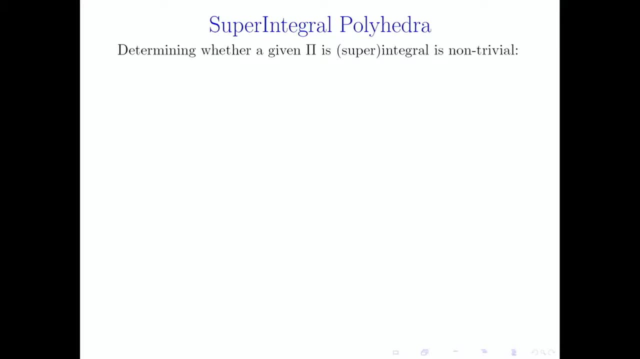 Three connected means you can remove two edges and it'll still be connected. Okay, So that's the same thing as just draw me any polyhedron you like. I take my kid's magnetiles and just randomly stick them together. I get some polyhedron. 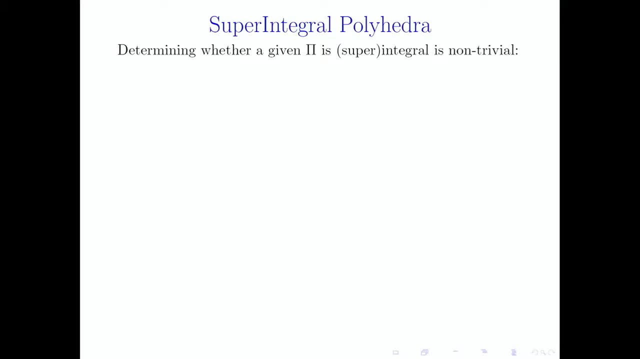 Is it integral? Is it superintegral? Well, how do you do this? First of all, Coby and Jerry of Thurston is an existence proof. It's not a. it doesn't tell you what the answer is. It says there exists. 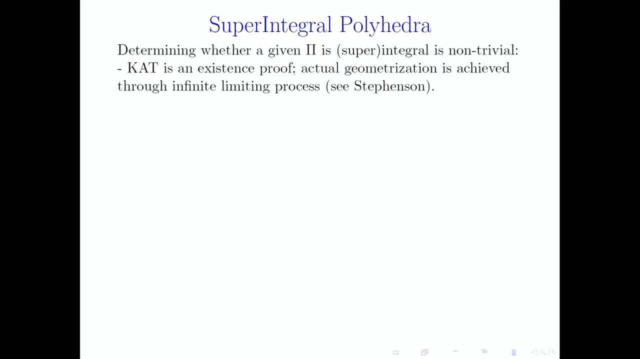 some way of pulling these things So the actual geometrization process is achieved. there are beautiful algorithms by Stevenson and others that let you do the geometrization, but it's an infinite limiting process. So how are we ever gonna know if 2.9999999. 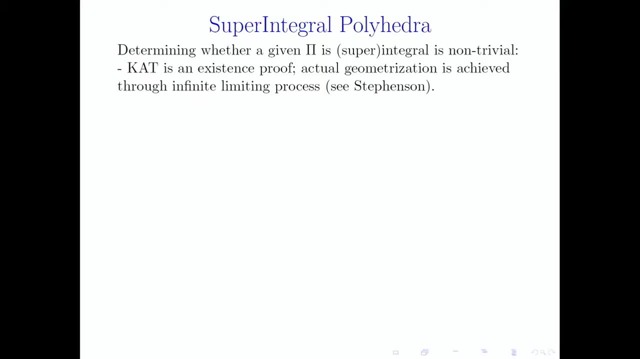 is actually three. Well, there's a, there's a savior: The the the most our rigidity comes to the rescue, and the fact that we are actually getting lattices in hyperbolic three space tells us we have rigidity. 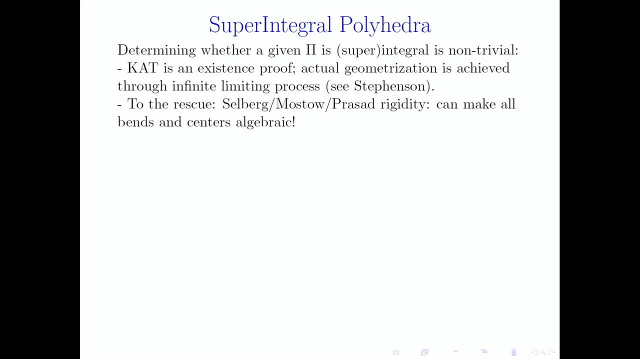 And rigidity means you can make all the bends and the centers algebraic. So when you see 2.9999999, what you do is you guess that it's three. Once you see enough decimal places, you guess what the algebraic value is. 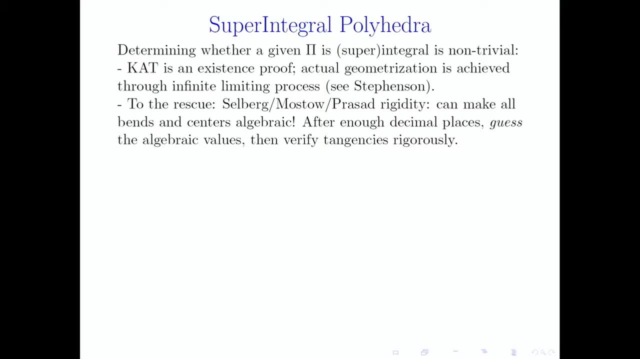 Then you go back to the tangency and see: do those algebraic values actually give me the tangencies I require On the nose? Okay, So in in practice, this is a finite process which then tells you whether or not a given guy. 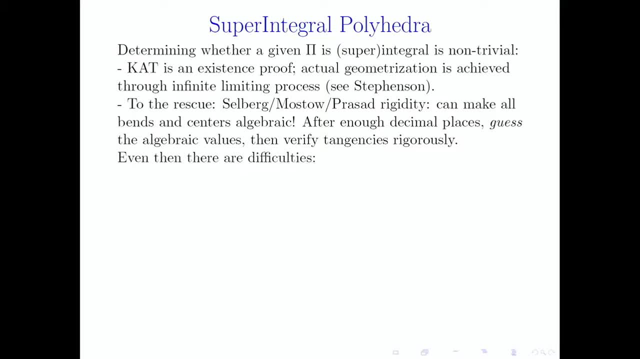 is integral, super integral, Okay, So, um, it's not, it's not trivial, but it's not so hard. But even then there are difficulties with the classification. So here's the theorem of ours Um, infinitely many polyhedra. 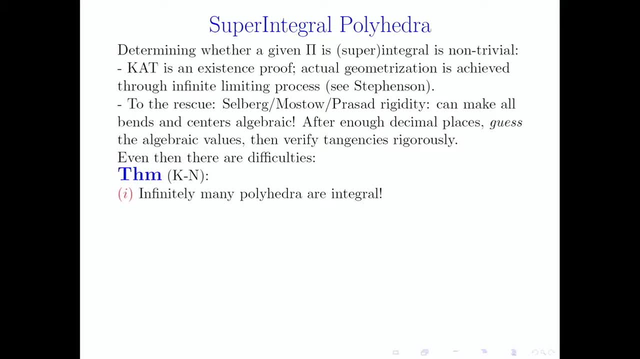 are integral and super integral. Well, uh, that's an immediate corollary of the fact that infinitely many distinct polyhedra actually give rise to exactly the same circle packing. So there's a symmetry group, there's not the symmetry group. 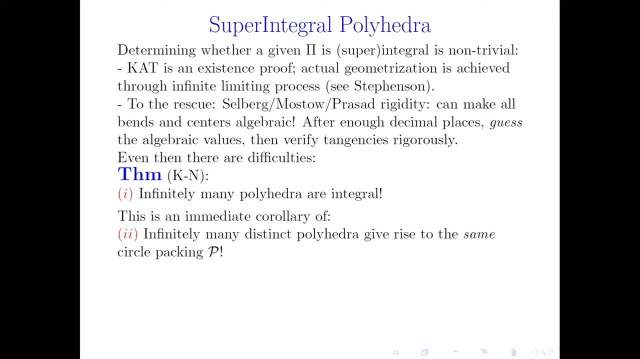 Of course, any normal subgroup of your hyperbolic reflection group has the same limit set, So there are lots of ways of realizing the same packing with a different gamma And, moreover, there are genuinely non-isomorphic integral circle packings, and infinitely many of them. 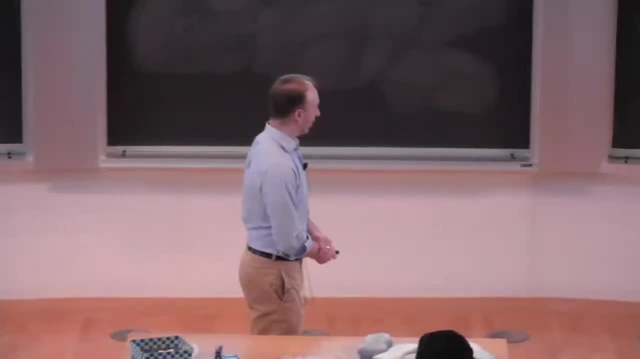 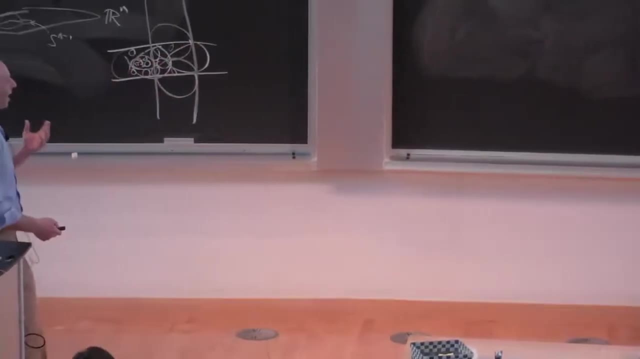 all of a sudden are super integral. Okay, So if this seems like it's contradicting what the consequence of super pack is supposed to be, which is the finiteness, it's actually not contradicting it because, um this, this theorem is proved. 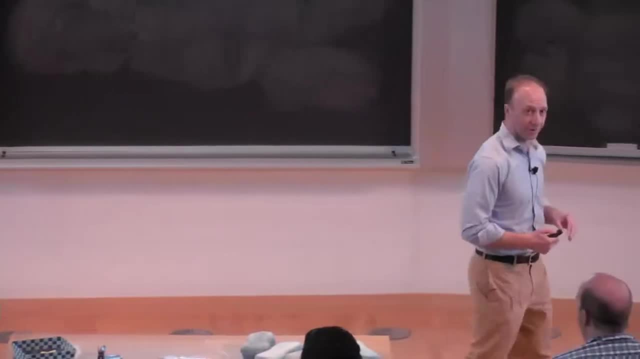 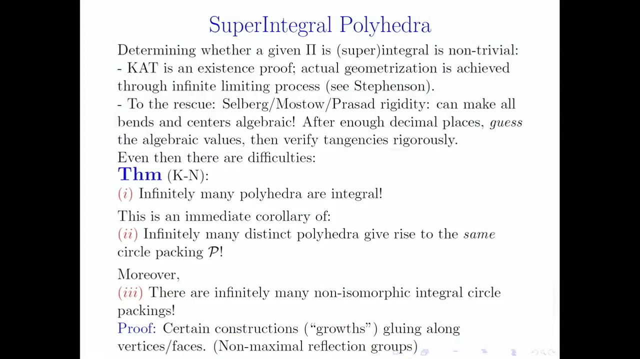 by certain gluing constructions along vertices and faces, which I'll I'll talk about a little bit later. Um, these are non-maximal reflection groups, So they're families. so we can produce infinite families from a given super integral. uh. 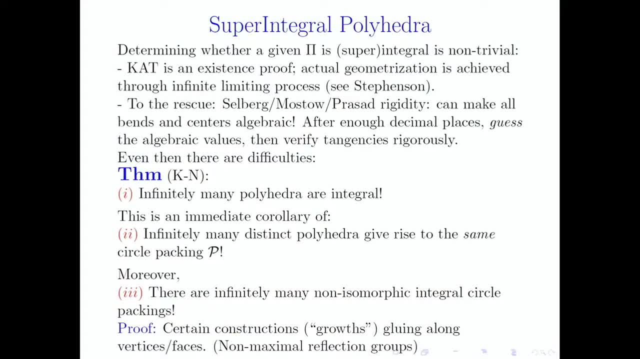 packing. Okay. So there is this infinitude, which makes it hard. if you hand me a, if my kid just puts some triangles and squares together and says: here, daddy, you know, do something with this. Um, I have to figure out. 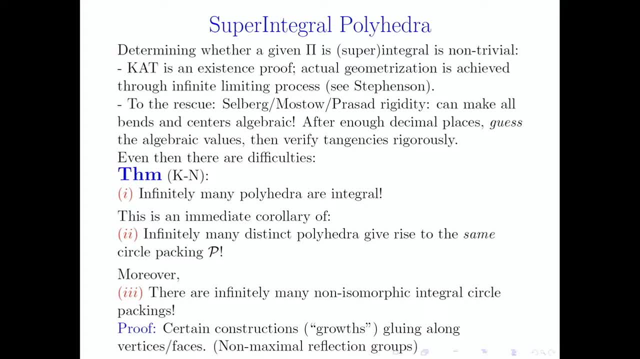 if it lives in one of these families. But up to maximality. we do believe that there's a finiteness. That's what the that's what super pack would predict. Okay, Does that make sense? So these are non-maximal. 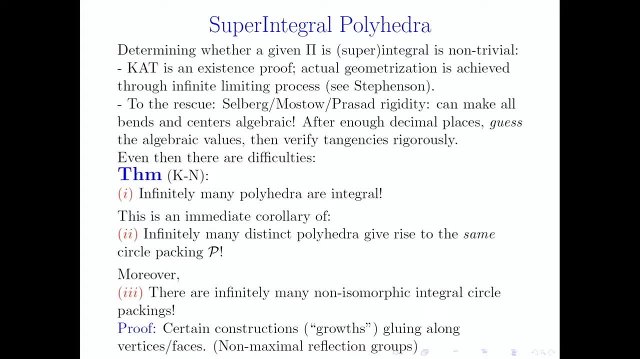 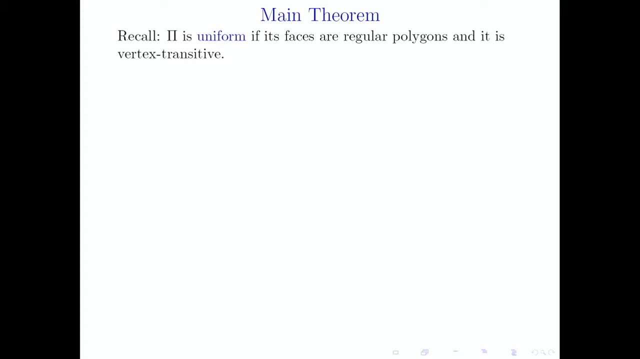 uh, reflection groups that are generating these infinitely many integral circle packings. Any questions on that? Okay, So, um so let's talk about the main theorem again. So what does it mean for a polyhedron to be uniform, As we said? 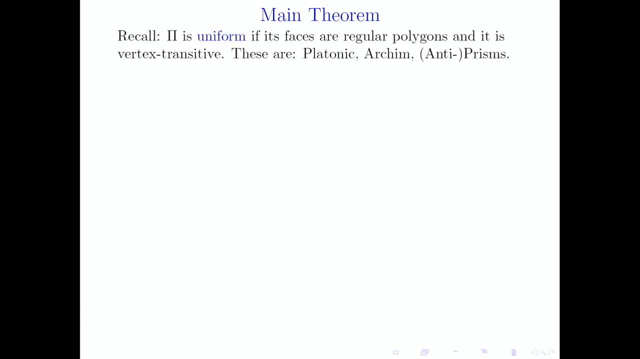 its faces are all regular polygons and it's vertex transitive. Every vertex looks the same, And so, uh, there's an old classification, essentially due to Archimedes. but he, he, for some reason threw out the prisms, so Kepler put them back in. 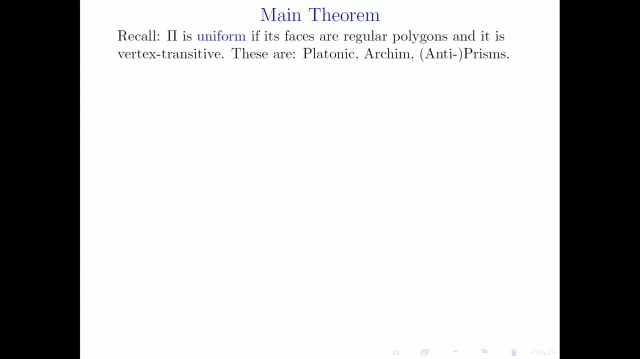 So, uh, the the uniform polyhedra are the platonic Archimedean solids and prisms and antiprisms, And the reason we wanted to look here first is if you're gonna see arithmeticity th- these things have. 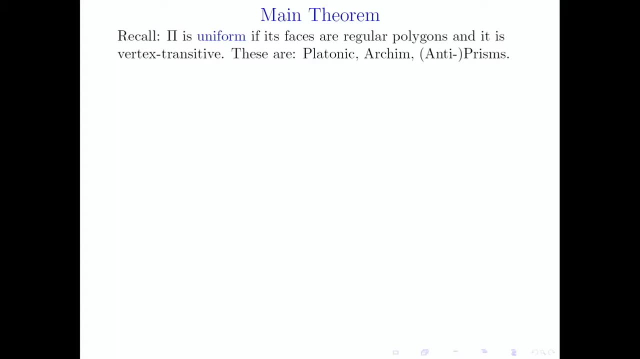 HECA opera- they're very highly symmetric, So these are kind of the most symmetric objects we could think to try And uh, here's the classification. So, as I said, the main theorem is that super pack holds four gamma packings. 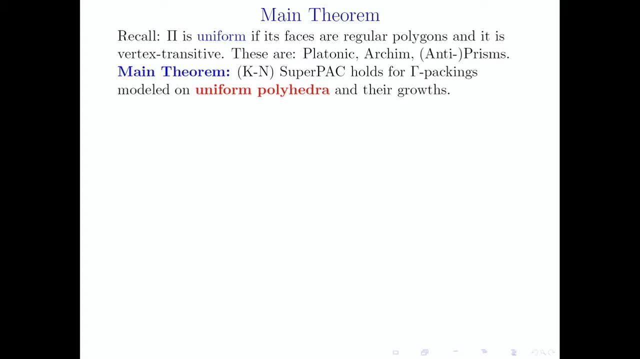 modeled on the polyhedra and also their growth. So, all of these, uh constructions of infinitely many super integral circle packings, all of them have arithmetic super groups And, uh, here's the complete classification. So, among the platonic solids, 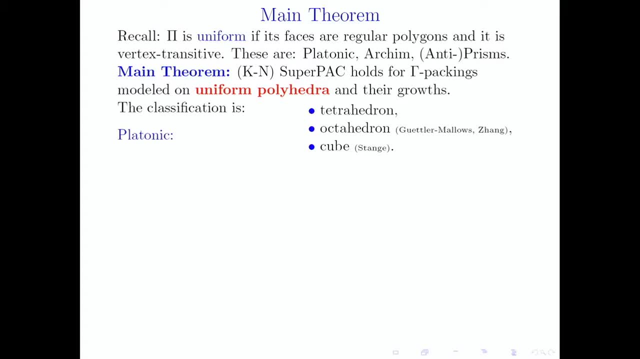 the super integral ones are the tetrahedron. What's a tetrahedron? The classical Apollonian packing is the tetrahedron because it's four. it's four circles, all of them tangent to each other. So the tangency graph. 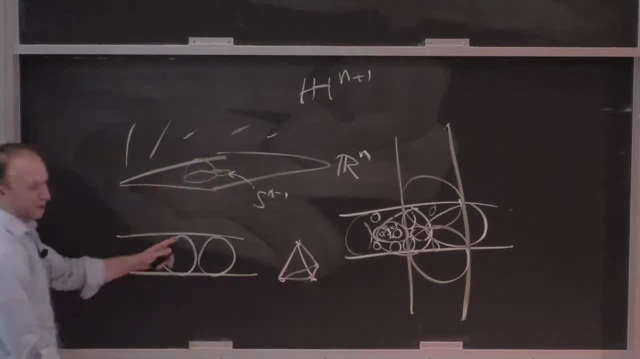 is the same as the tangency graph of a tetrahedron, right Complete graph on four vertices. Okay, The octahedron is what we discussed. this is, and Boyd Um the cube appeared in work of uh. 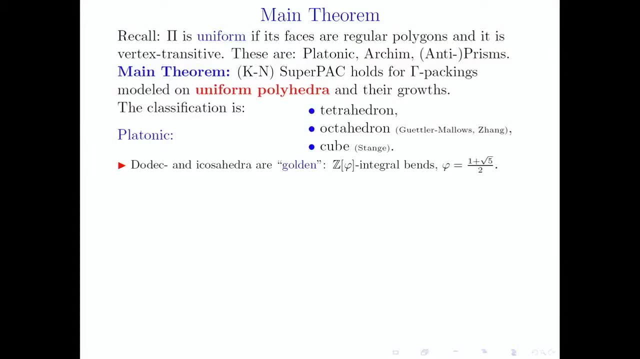 Stange. Uh, if you look at the dodecahedron and icosahedron, they're not integral and hence not super integral, but you but they are, uh, what we call golden, So you can make a cube octahedron. 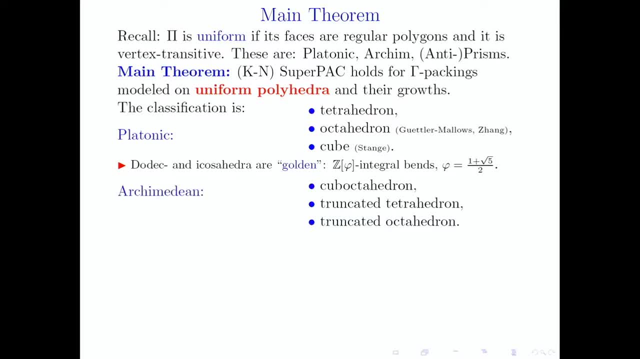 out of a cube octahedron Among the Archimedean solids. the cube octahedron that we discussed is super integral. The truncated tetrahedron, also the truncated octahedron. you can sort of imagine what those guys look like. 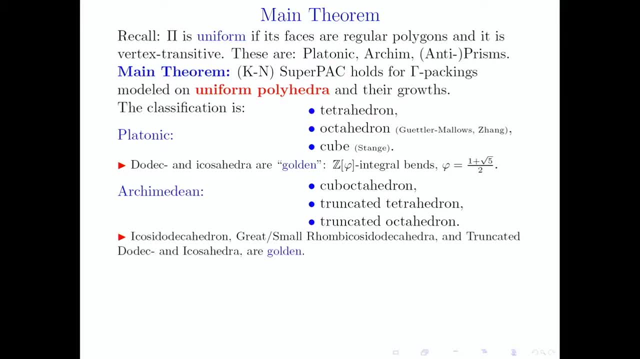 Then there are a couple more: the icosahedrodecahedron, which is similar to a cube octahedron, Then you have the uh Rhomba icosahedrodecahedron and his cousin. 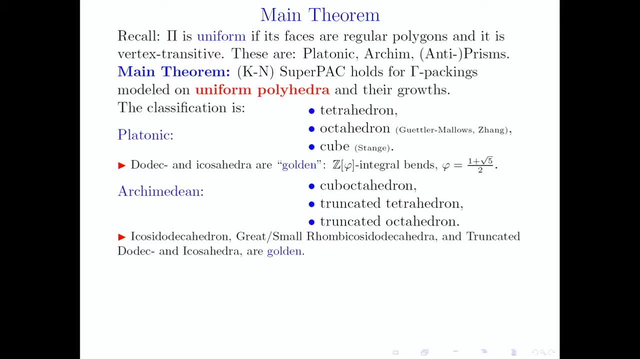 great and small and the- if you, if you don't know the zoology, never mind, But a bunch of them are golden. Then you have a truncated cube, octahedron. that is silver. So silver means that there I learned this. 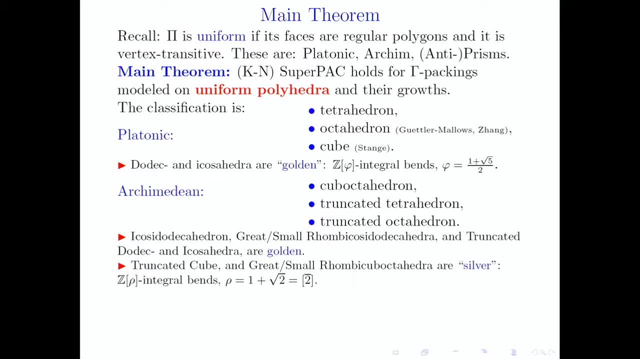 from Wikipedia, the silver mean apparently, is all twos instead of all ones in the continued fraction. So so these guys are not quite as good as gold, Uh, silver. but when you go to, for example, the snub cubes, 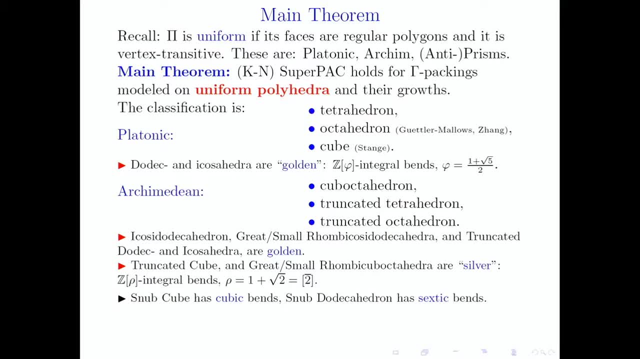 so you know what a snub cube is. You take a cube- I should have brought my magnetos. You take a cube and you pull it apart, So that would give you, like a, a rhombic, what break it and you. snub means crooked nose, right. 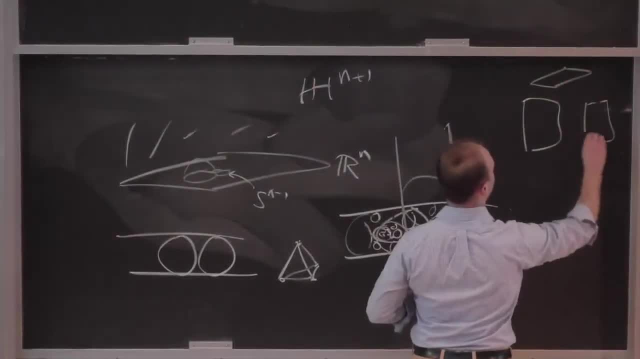 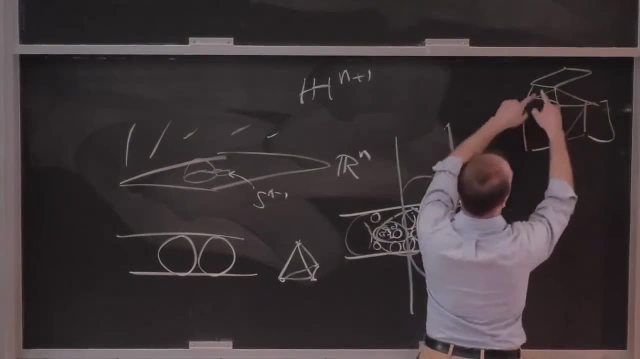 So you take a cube and you pull its sides apart and what you would have here is rectangles. but then you twist the rectangles so what you get is triangles. So, anyway, around each vertex is like four triangles and a square. So that's the. I think that's right. 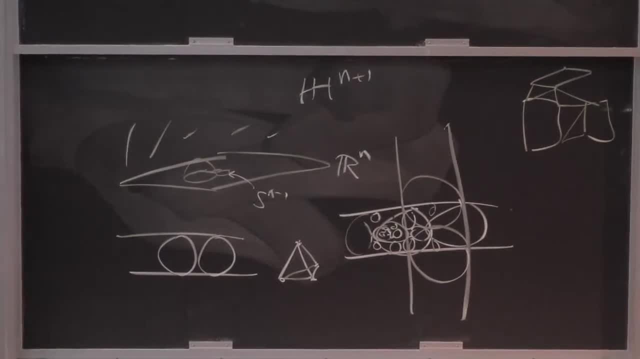 So that's a snub cube. It has cubic bends, not integers, And the snubbed dodecahedron has sextic bends. So I don't know. when I said, master rigidity tells us these are gonna be algebraic. 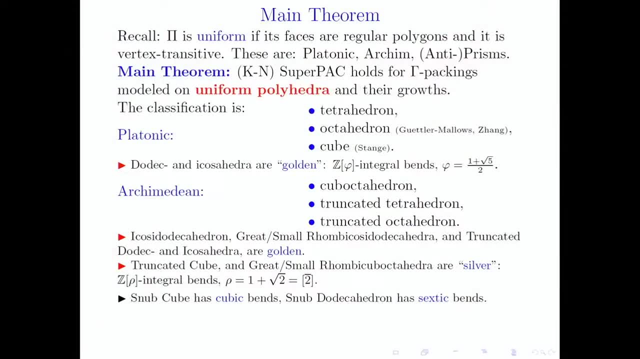 I don't know the degree, And presumably the degrees are unbounded. I don't know if they're bounded or not, But the interesting thing is we're no longer for these much less symmetric guys, we're no longer getting even integers. 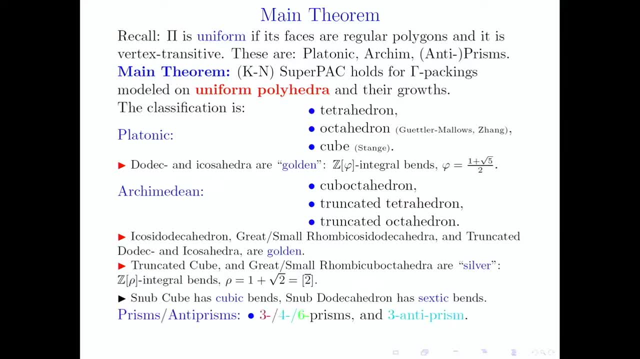 algebraic integers as bends, And among the prisms and the antiprisms. this is where it gets interesting. The three prism, the four prism and the three antiprism are all so you know what a prism is. 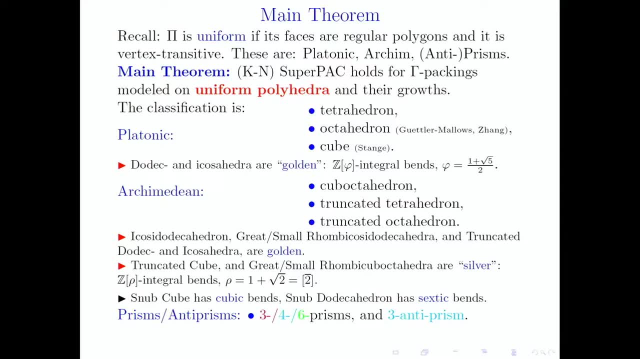 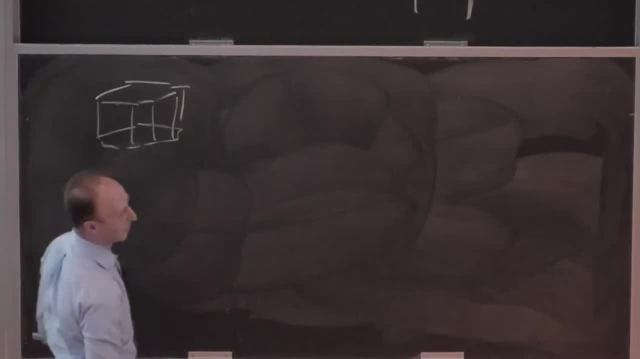 So a prism is: you have an n-gon on top and an n-gon on bottom and you just drop squares in between, right, That's a prism. So what's a four prism Cube? right? So that's cheating. that's why it's in green. 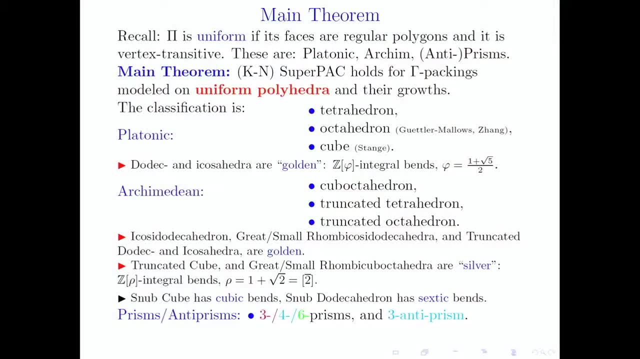 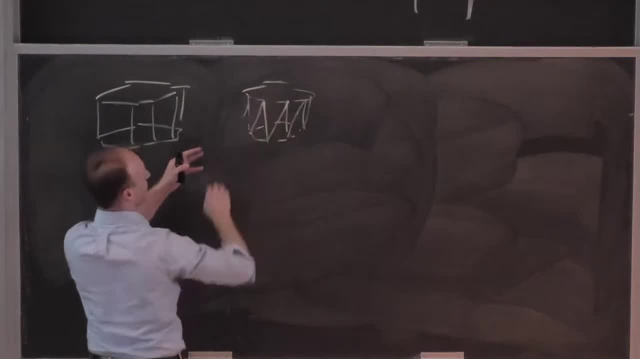 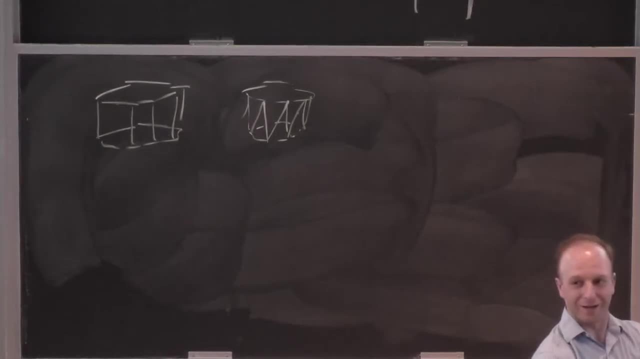 What's an antiprism? You take a n-gon and you twist it by half a rotation and then you connect by- like Homer Simpson hair- triangles Like a drum or something. So what's a three antiprism? Take two triangles, snub it a little bit. 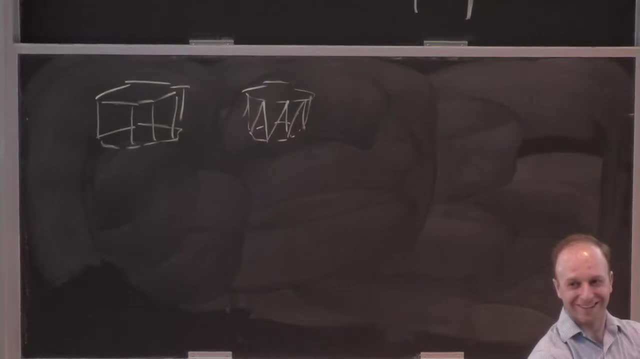 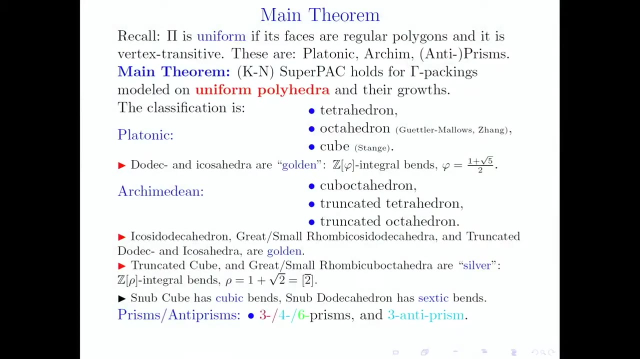 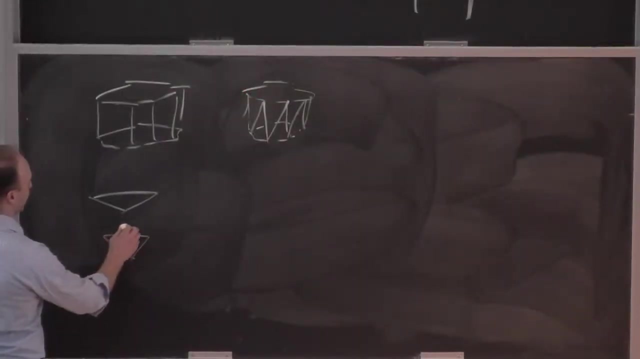 and connect triangles, Octahedron. Okay, so those are not new. So the four prism and the three antiprism are not new. Let's talk about the three prism. The three prism is also not new Because the three prism is the gluing along a vertex. 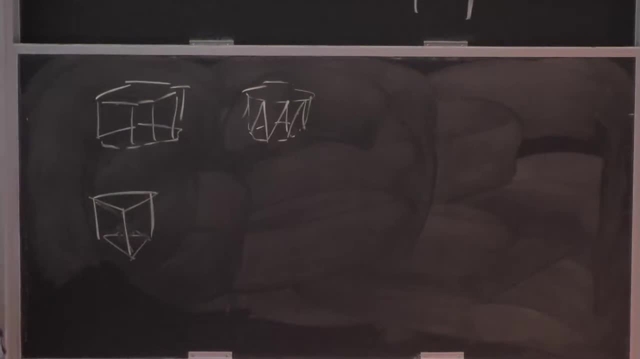 So what's a three prism? Let me draw the three prism. There's a three prism. This'll be the same as if I take a tetrahedron and I double it across the vertex and then I remove the vertices And I so I'm gluing along a vertex. 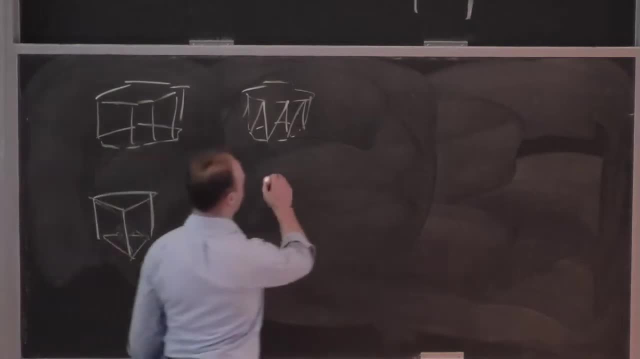 This is the operation of gluing along a vertex. So what does that mean on the level of circle packings? So if I start with my, I'm gonna do a couple. if I start with my, I'm gonna do a couple, I'm gonna do a couple. If I start with my, I'm gonna do a couple, I'm gonna do a couple. 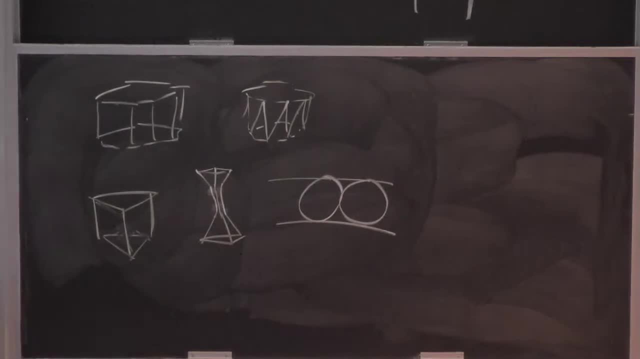 my Apollonian circle, packing one of the vertices. let's say, this vertex is the one that I'm gonna remove, So I invert through it and then I remove it. So that's the doubling along a vertex. So it's not new, because it's super packing. 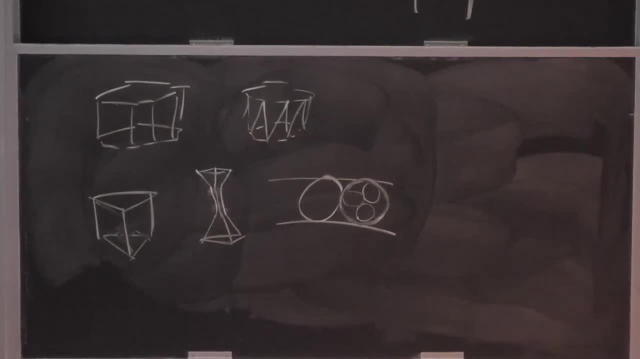 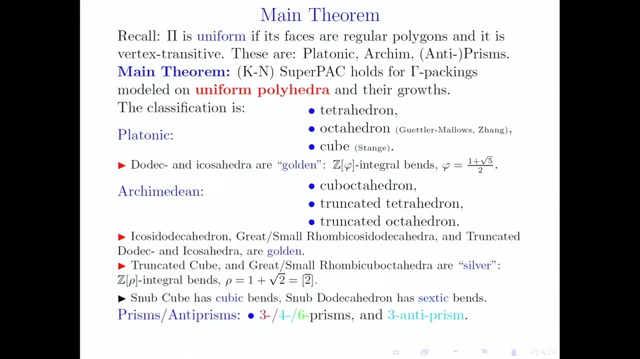 is a sub packing of the Apollonian super packing. That's what makes it super integral. It lives inside something else that's non-maximal, That's the non-maximality of this three prism. Does that make sense? Is that clear? 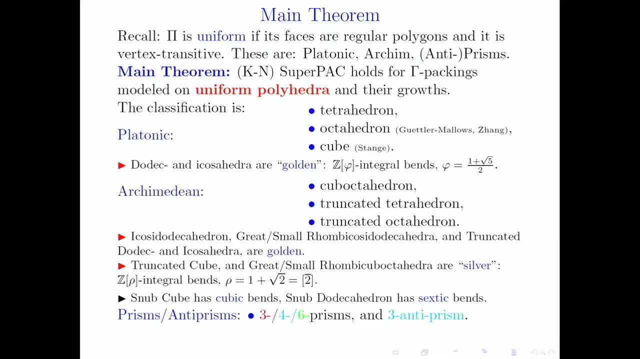 The six prism is very interesting and I'm gonna talk about it later. This is in whatever color, this is light green or something. It's integral, it's not super integral and it's super group is not arithmetic. So this is my Deligne-Mastow example. 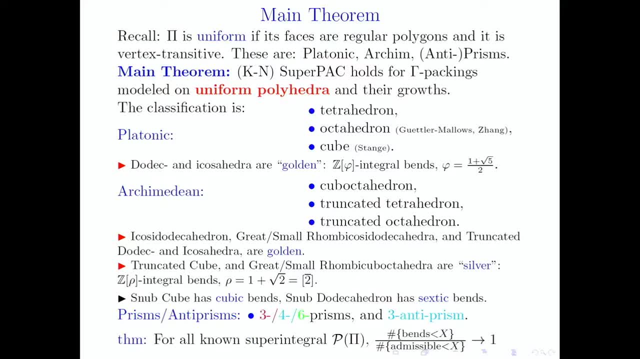 So I'll come back to this one And a theorem with the little t, because the details are still written up For all of these super packings. you get the same theorem as what I had with Bergan about the almost. So the bends up to x, you find relative. 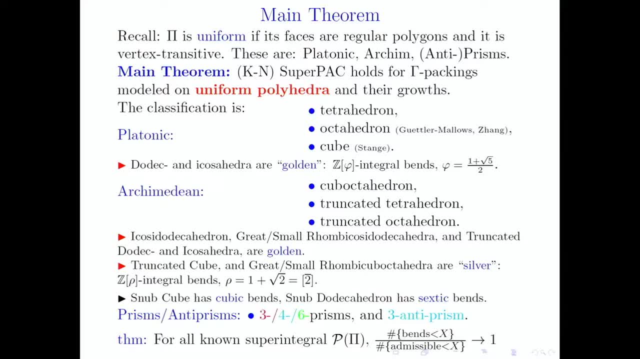 to the ones you should find tends to one, And I think Elena is speaking about parts of this on Friday, So you'll get to hear: Sorry, this is not an analytic number theory talk. The analytic number theory is hidden in probably this one. 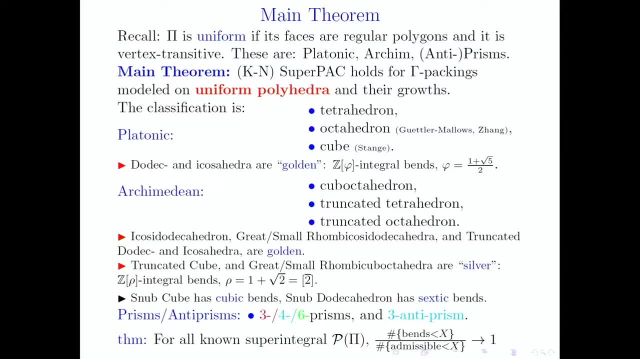 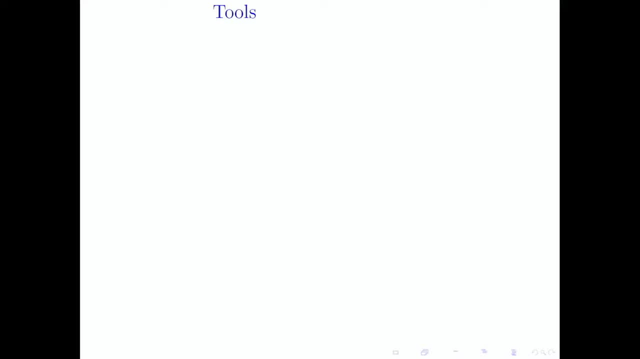 So there's a circle method there, There's expander, There's this. You'll like it, Go to Elena's talk, But that's not what I'm gonna tell you about, So let me spend a little bit of time saying how we get all this stuff. 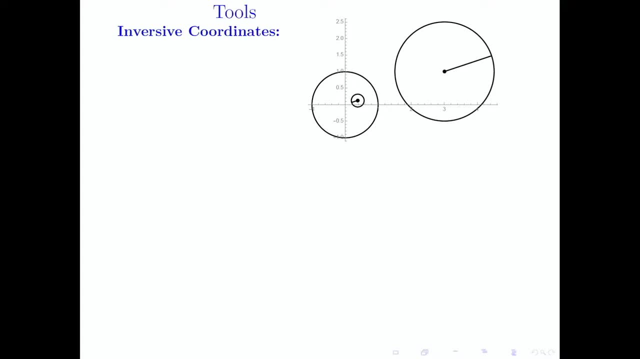 Where is this coming from? So what tools are we using? The basic tool is to- and I learned this from Jeff- is to use inversive coordinates. So in some form these go back to what. Clifford Darbeau- These are kind of the guys I found. 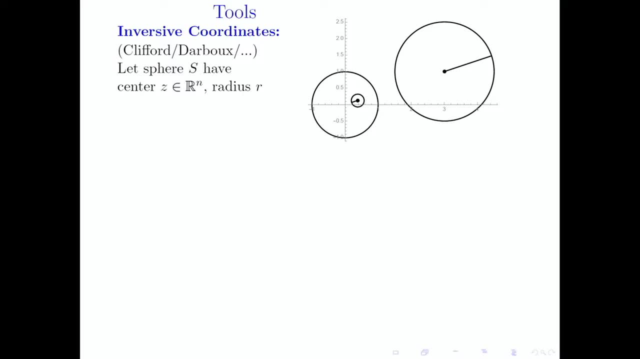 So if you have a sphere in space and it has center z some point in space, and radius r, what's the co-radius? The co-radius is the radius of the sphere you get by inverting through the unit sphere. So I'll take this sphere. 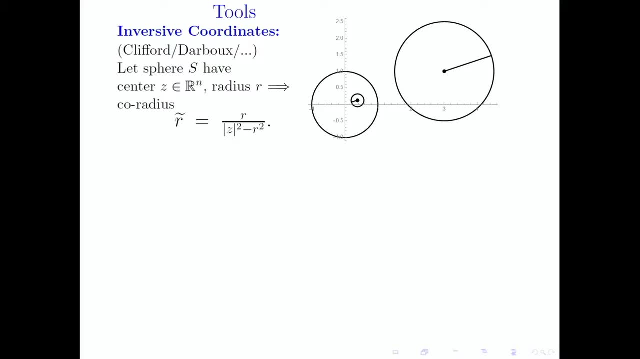 I invert through the unit sphere, I get some other radius. That's this co-radius exercise. The co-radius is equal to the radius divided by norm, z squared minus r squared. If you're bored, go do this exercise, Okay. So once you have this, you do a little bit of algebra. 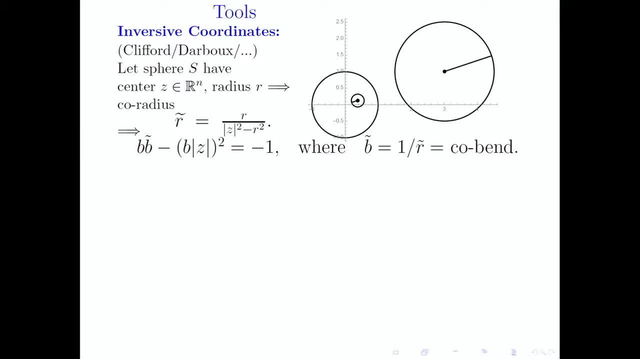 very simple algebra from here And you find that the bend, the bend is the reciprocal of the radius, The co-bend is the reciprocal of the co-radius. So bend times, co-bend minus bend times, center, quantity squared is always equal to minus one. 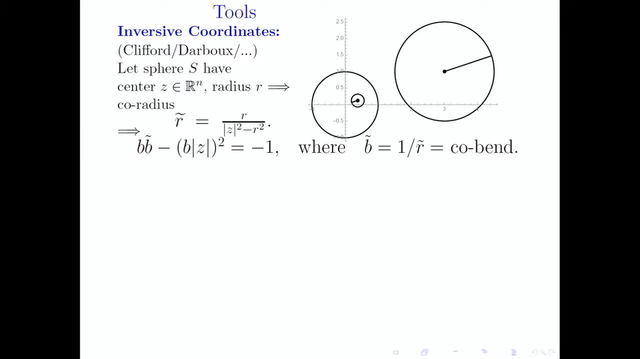 This is just algebra from the first equation. So what does that suggest to you? It suggests quadratic forms. So what you should do is to a given sphere you should attach what we'll call the inversive coordinates, which are bend, co-bend and bend center. 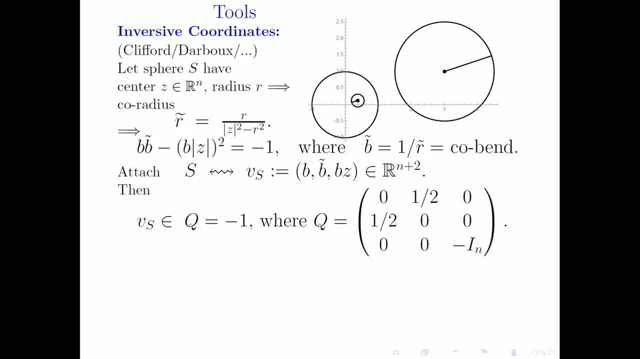 Then that will lie on the on the uh one-sheeted hyperboloid q equals minus one, Because look where q is this form, a half, a half and minus the identity, Because look at what's happening here. 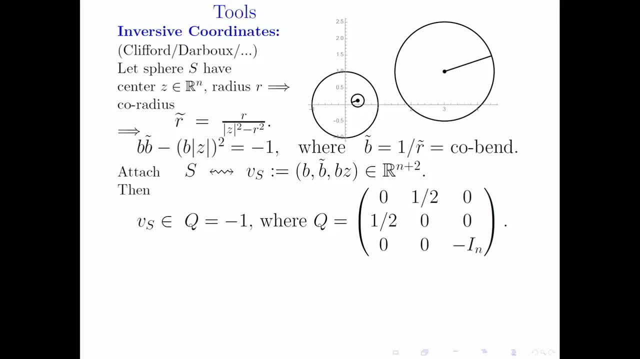 It's a half, a half, b, b, b, twiddle and then, minus the sum, some of the squares, Okay. So is that clear? That's where this, this is a universal quadratic form, regardless of what circle packing you're talking about. 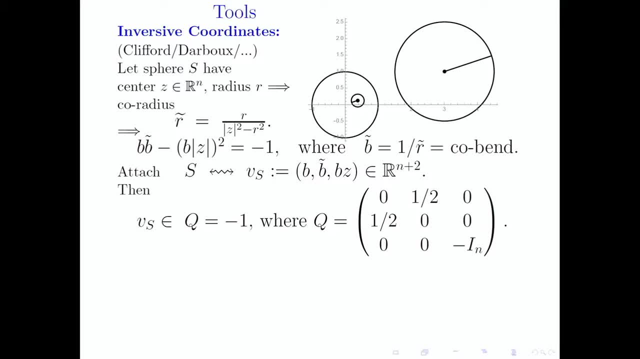 And it looks the same in all dimensions. Okay, So this, this pointed r n plus two actually lies on this one-sheeted hyperboloid q equals minus one, or the real points of that. Is that clear? That's just algebra. 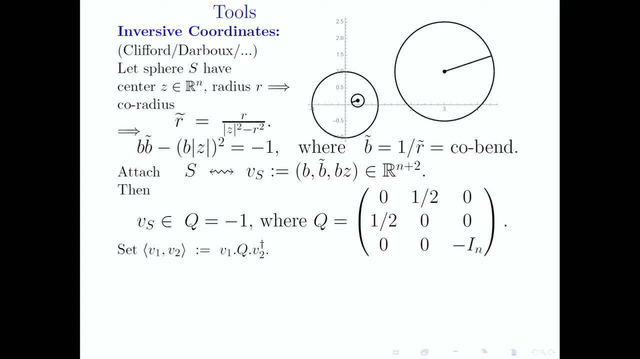 So let's use this q as our inner product matrix. So this is sometimes called the Lorentzian inner product. Some people like to make a change of variables first. I like. I like q just as it is. The signature of q is one n plus one. 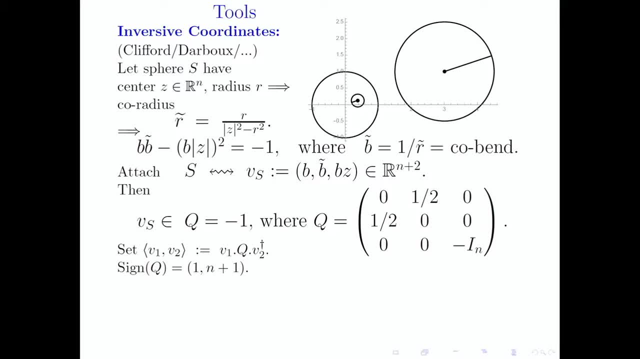 So that's why minus one- maybe you're used to minus one. being in two-sheeted hyperboloid, My signature is one n plus one, So this is a one-sheeted hyperboloid. And what's really going on again? 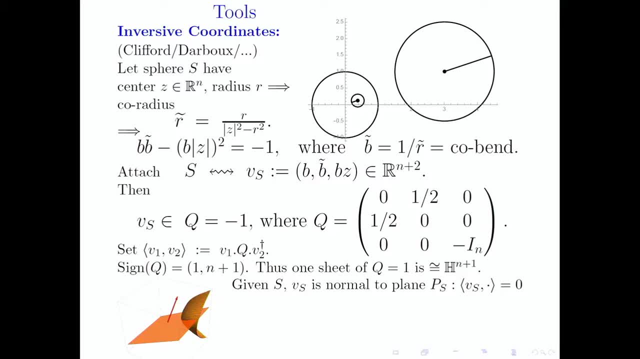 maybe this picture isn't the isn't the best one I used to have chalk. There we go. So what's really going on is: q equals one is a two-sheeted hyperboloid And there's another sheet there, The point v. so what? where does this? 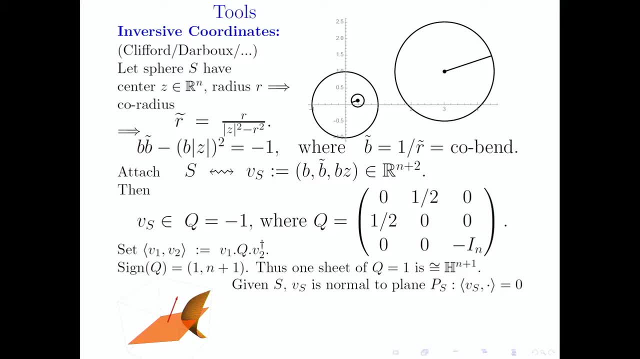 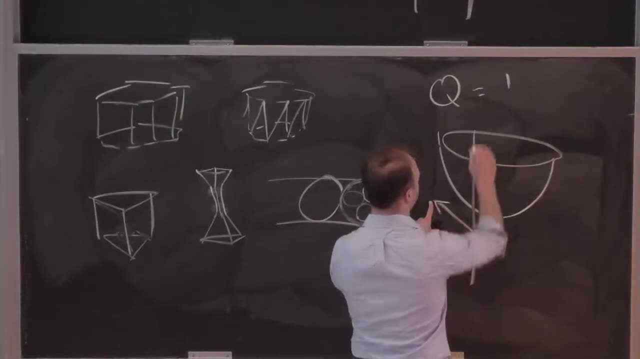 what does this v have to do with the sphere, the initial sphere? It's very pretty. V has norm minus one. These are the points that have q norm one. V is the normal vector to a plane. So if you take the Lorentzian normal, 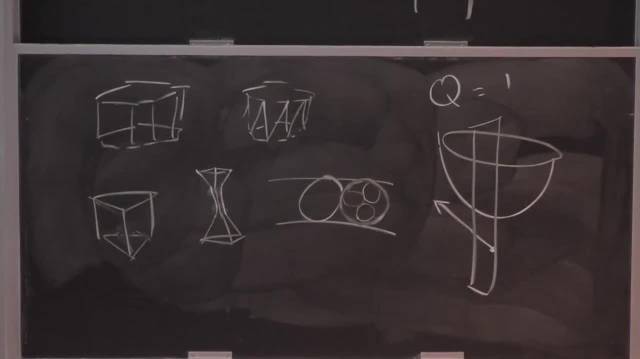 the plane of all things orthogonal to v under this q inner product. the intersection of that will be a codimension one hyperbolic space. Okay, so the intersection of this plane with this one sheet of the two-sheeted hyperboloid is a one-dimension lower hyperbolic space. 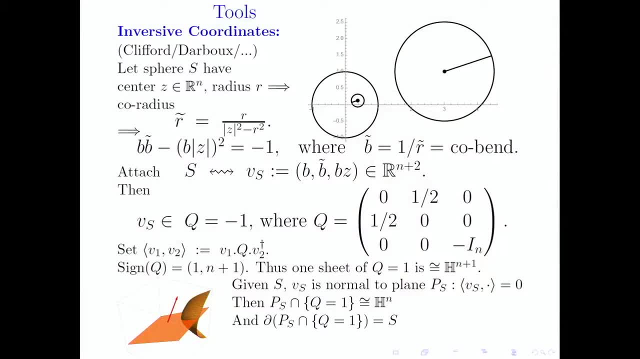 And the boundary of that in your favorite compactification. unfortunately, I can draw. I can only draw in three dimensions, whereas it's supposed to be a four-dimensional picture, right signature three, one for circles. So this is the circle. The boundary of this plane is the original circle. 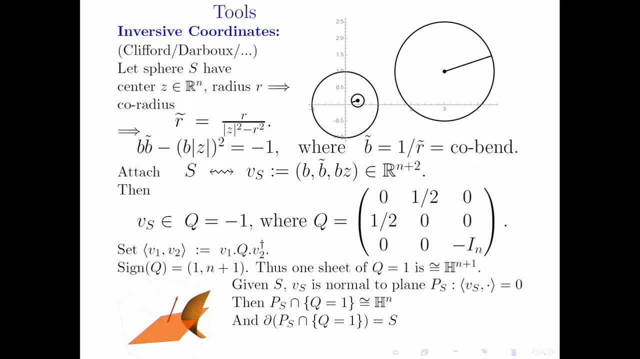 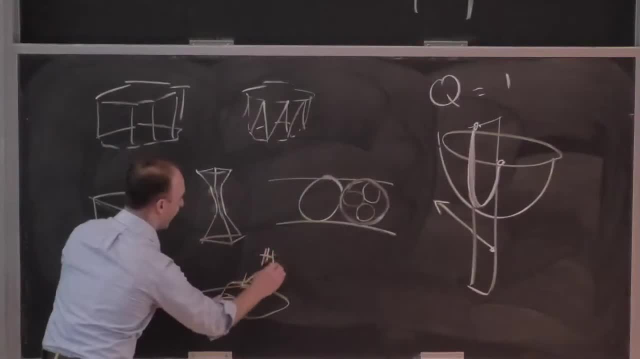 So what's really going on is- I guess the picture's up there, I'll draw it again- here You have your circle. That circle is the boundary of a hyperbolic plane. This is hyperbolic plane which sits inside hyperbolic three space. 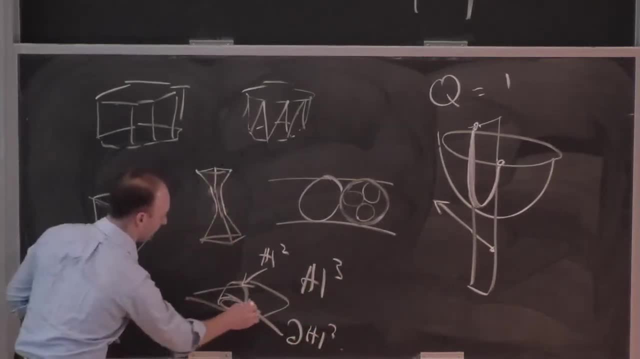 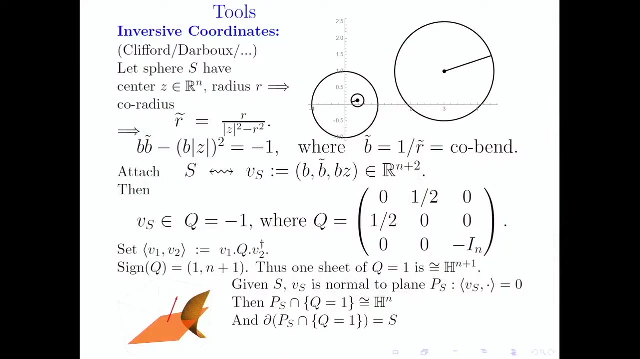 And this is the boundary of the hyperbolic plane, the circle. Okay, so that's what this picture is explaining. What this? why these coordinates? Okay, there's some equation that told us what to do? No, they're very natural coordinates. 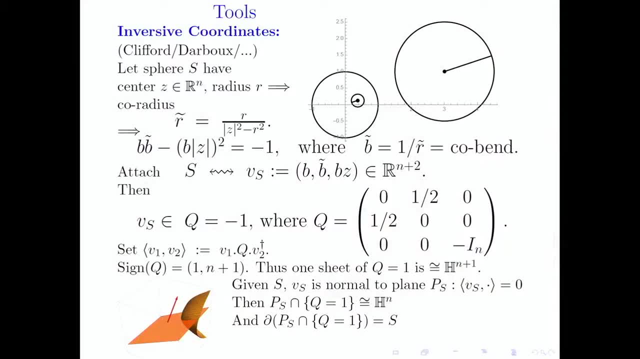 They're coordinates describing this model of hyperbolic geometry. Okay so, and once you have this model, it's obvious what we're gonna wanna reflect through spheres. How do you reflect through a sphere? Well, once you have this model, 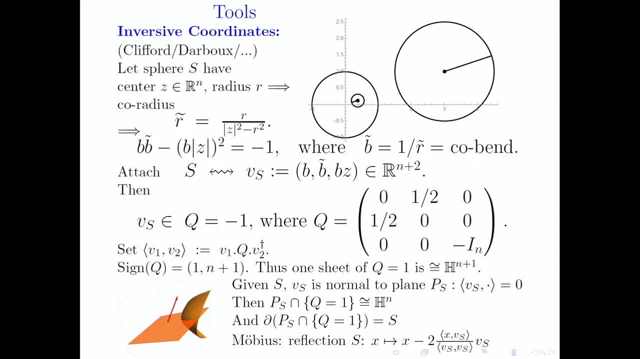 it's just reflection through this plane. And how do you reflect through the plane when you're the normal vector? It's this completely well-known fundamental formula for reflections. Does that make sense? So I'm just setting up a little bit of notation for what we're gonna do. 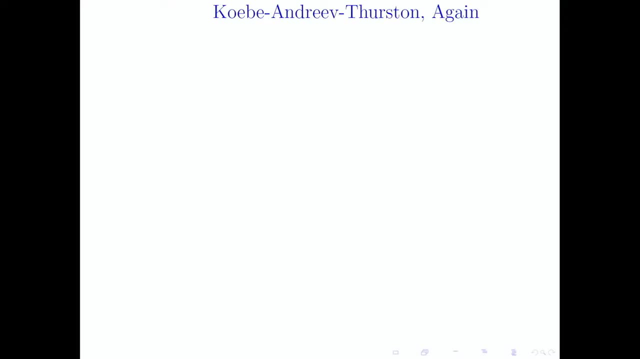 Okay. so let's look at Coby-Andrea Thurston, Coby-Andrea Thurston from this point of view. So what is it saying? So another thing you should know is that this inner product measures the hyperbolic distance. 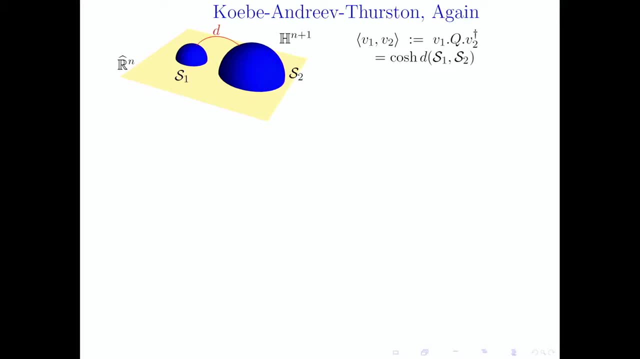 or the cost of the hyperbolic distance between these two planes. So if I have a sphere S1 and a sphere S2, and I take the hyperbolic planes for whom they are the boundary, then the hyperbolic distance between them. 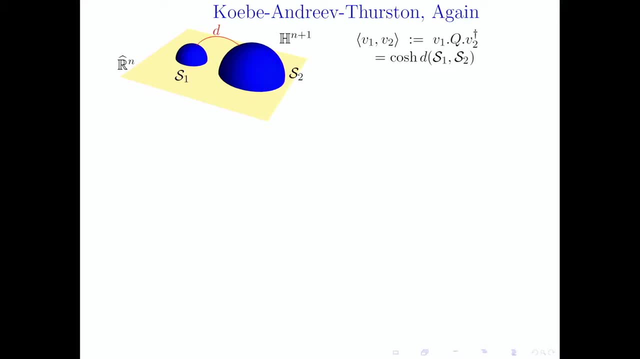 or the cost of it, is exactly what this inner product is measuring. Okay, so what you can see from that is: well, we already know that, if you have, if the sphere, if V1 is equal to V2, then we're taking norm of it squared. 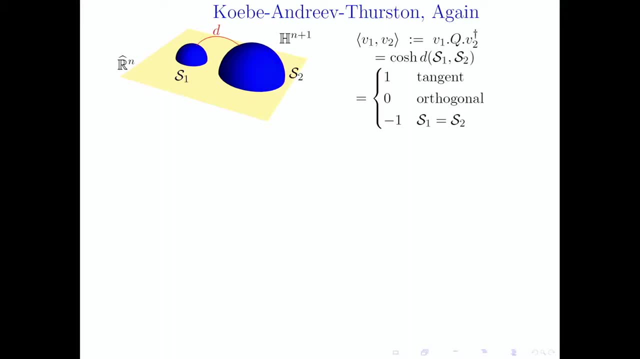 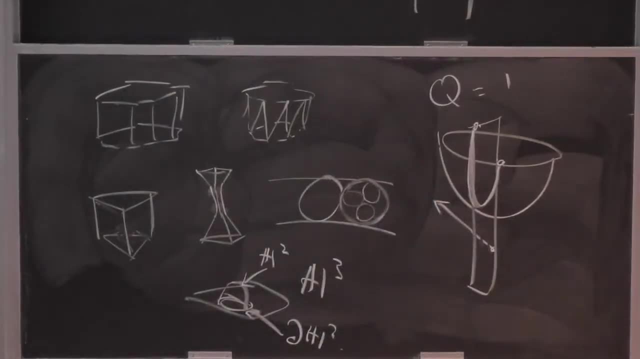 and the norms of all of these normal vectors are minus one. These lie on Q equals minus one. So this Vs Vs has Q of Vs equal to minus one, whereas the hyperbolic space is at Q equals one. Two spheres have inner product one. 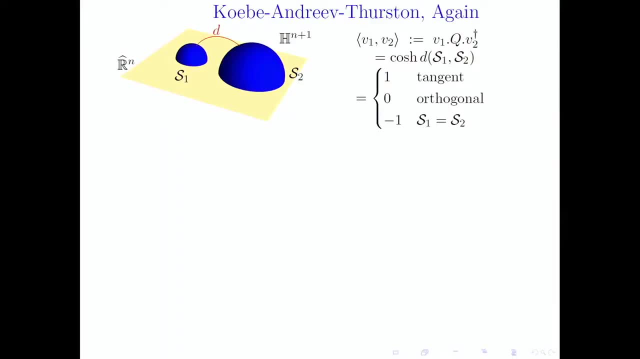 That means the distance between them is zero, That means they're tangent, And the cosh being zero means the distance is complex, which means cosh turns into a cosine, which means the two spheres intersect orthogonally. So spheres intersect orthogonally if, and only if. 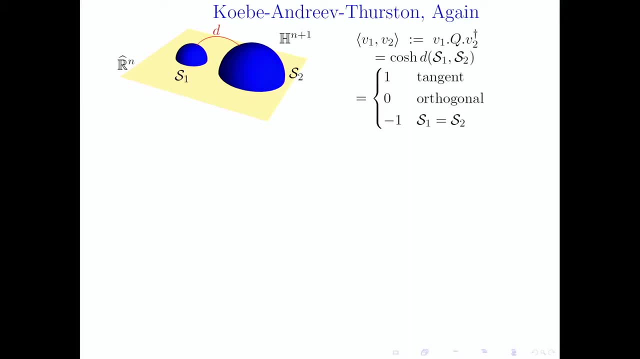 the inner product of their normal vectors is zero, or tangentially if one. So what does that mean? So what is Kobyandre of Thurston? You give me the tangency data of your polyhedron with N vertices, the dual polyhedron with M faces. Here's the equation you need to solve. You take Vs, So 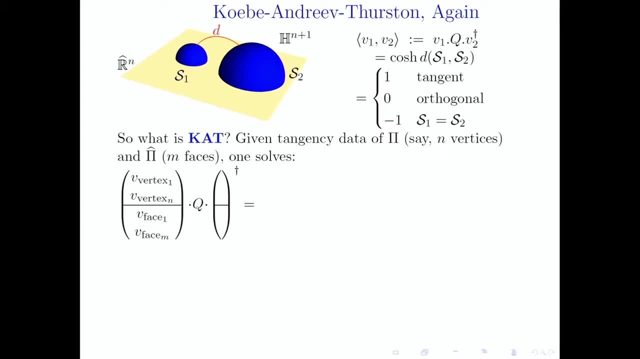 the Vs are the variables. The Vs in the N vertices and the M faces will have self-interproduct with Q, which is what we call the supergrammian. So it's the gram matrix not only of the vertices but also the faces and what the intersection looks like. I'll give you an example in a. 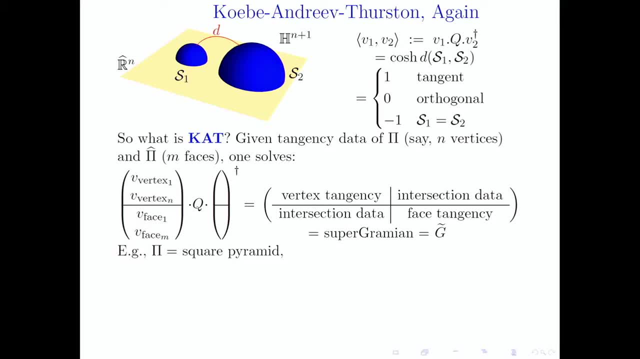 second so you can see what's going on. So let's do the example of the square pyramid. That's kind of the smallest non-trivial, non-Apollonian example. So what's a square pyramid? You know what a square pyramid is? Well, you can read it off from this supergrammian. 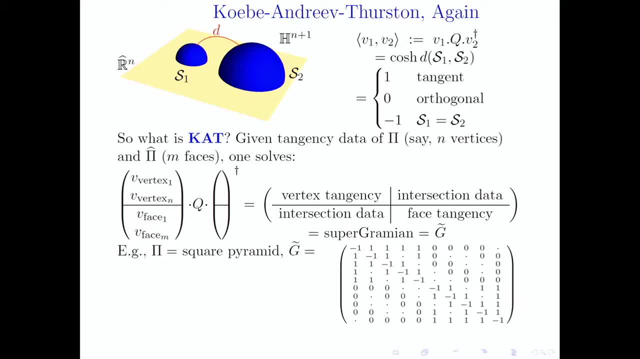 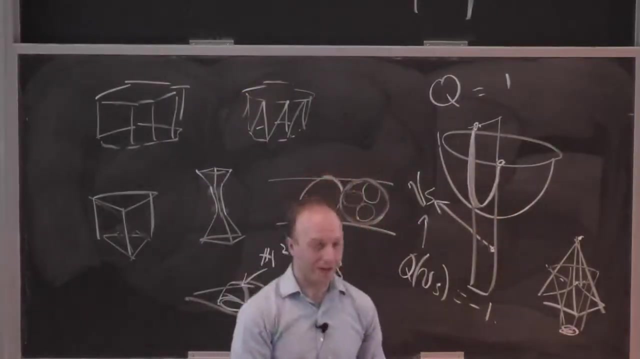 So this part is the vertical dividing line and this part is the horizontal dividing line. So the square pyramid has dual. It has four faces and one face that's touching all of them. Its dual is also a square pyramid, If you can see that. And let's look at this first line. So the first, the index, one vertex. 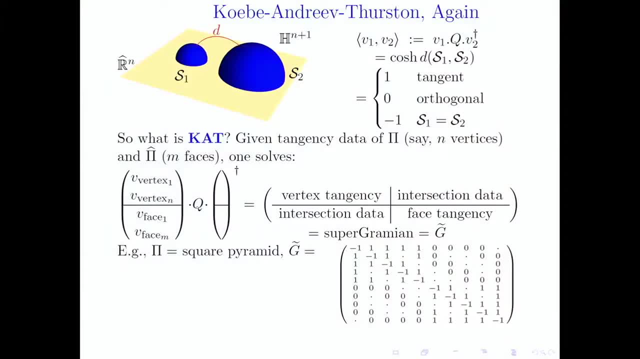 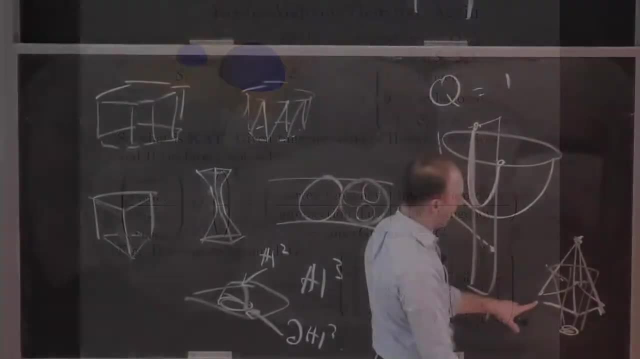 is well, there's always minus ones down at the diagonal. That's because of that. But then this one is tangent to the second and the third and the fourth and the fifth, So that means that's the top vertex. He's tangent to two and three and four and five, And he's 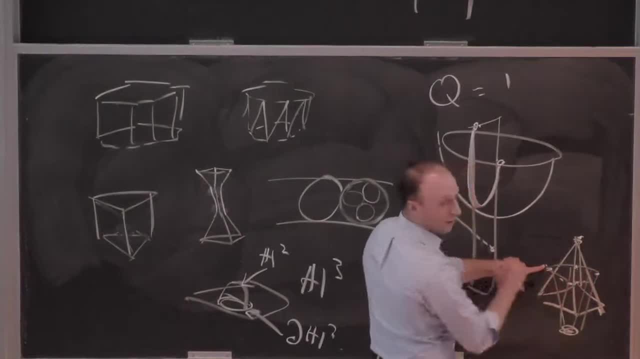 orthogonal to four of the dual faces, because he crosses those faces. But I have no idea what the relationship is between the bottom face and the top vertex. So that's this dot. The dot is an unknown. It's another variable to solve for. Okay, So the tangency data. so the tangency data. 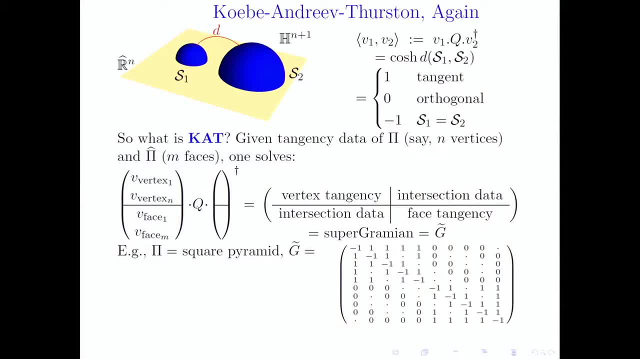 in this square tells you that you have a square pyramid. The tangency data here again tells you that you have a square pyramid And this is the intersection of the faces: which vertices lie on which faces. So that's just purely combinatorial data that you stick into this partial gramian. 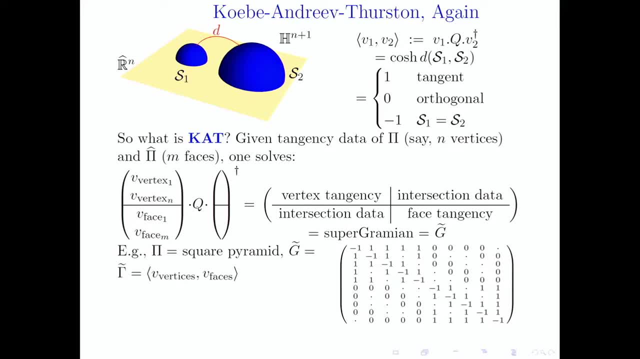 And then you need to solve for these vertices and faces and also these dots, which are also unknown, so that you get the equation: This thing times Q in a product with itself. Q is this supergram. So what is the super group? It's reflection through the vertices and the faces, and 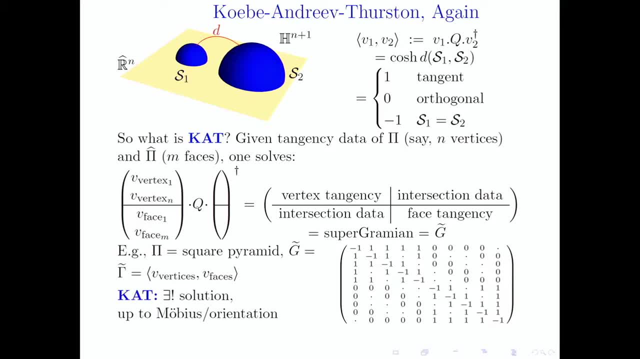 the squares, at this vertical line, In the Coby and Draythurston theorem is there is a unique solution up to orientation and Mobius transformations. There's a unique way to solve this equation that we set up. So in the case of the, so here's the gramian. in the case of the square, 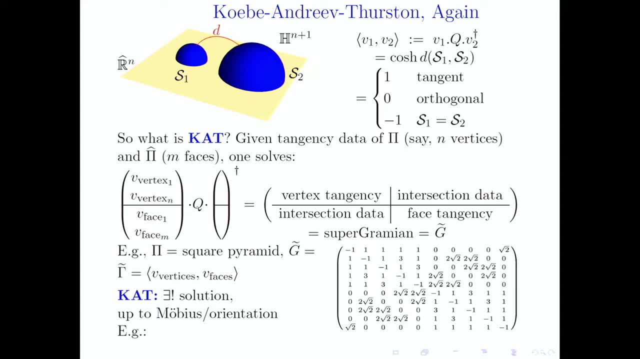 pyramid. Remember we had these dots, these unknowns. when you solve it, some of the unknowns become threes and some of the unknowns become like two, two's and two's and stuff. Okay, Does that make sense? Is it clear? 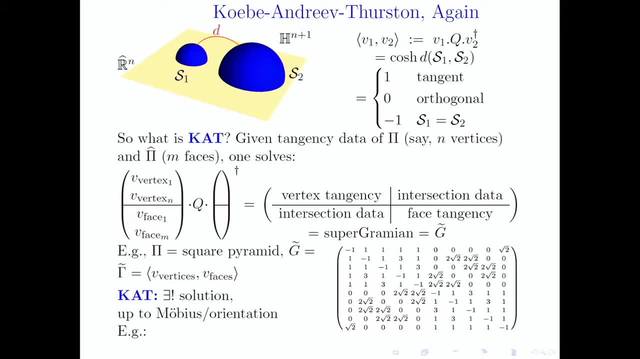 Okay, So that's the conundrum of theерum, Like we said, two. So the answer is yes. The answer Is it clear what we're doing. So this is the numerical step. You tell the computer once you have this unknown data. 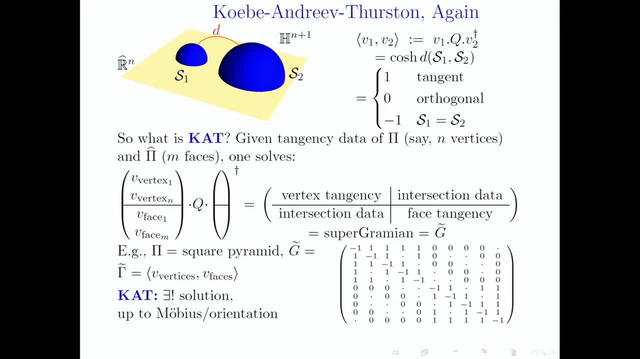 you tell the computer: find me some numerical solution to this system of equations, incomplete system of equations, and whatever it spits out, you then look to algebraize and once it's algebraized, you check: do I really get this exact on the nose? 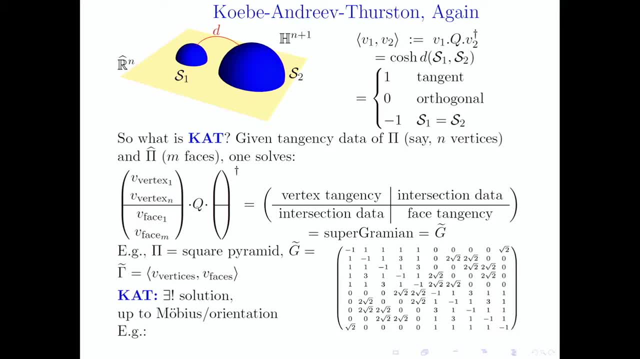 the ones and the minus ones and the zeros exactly where they're supposed to be. Okay, So what So? I claim that this supergramming is everything. This is the whole game. Once you have the super, whatever the supergramming happens to fill out to, 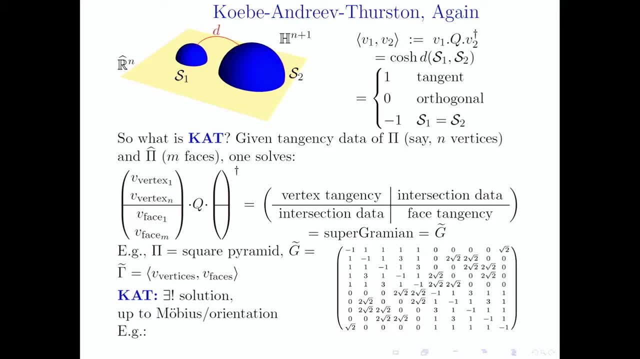 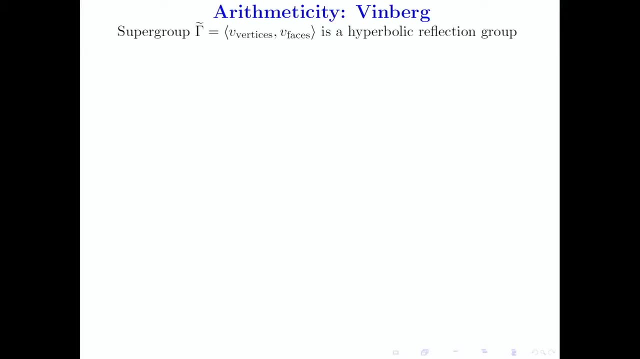 these unknown values. they determine everything, They determine the entire arithmeticity property by a theorem of Vindberg. So what's the theorem? So again, the supergroup is generated by reflections through the vertices and the faces, the polyhedron itself and the dual polyhedron together. 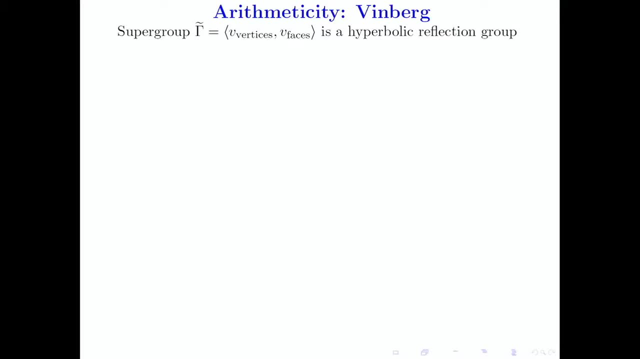 That's the lattice. So it's a hyperbolic reflection group, finite volume hyperbolic reflection group, And its gramian is exactly this, what we called supergrammian g twiddle. So for the four-pyramid, here it is again. 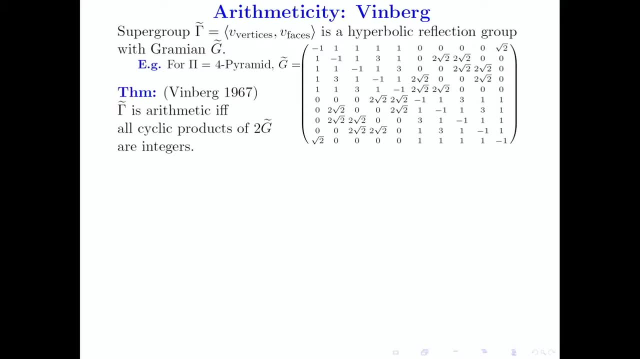 just so we can stare at it. So here's Vindberg's theorem. A hyperbolic reflection group. gamma twiddle is arithmetic if, and only if, all cyclic products of. well, you're allowed to have half integers. so let's say twice: the gramian are integers. 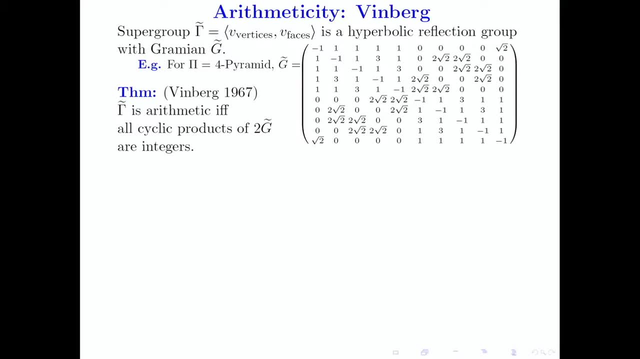 What does it mean to be a cyclic product? I start at some. this is what the 1,, 2,, 3,, 4,, 5,, 6,, 7, 8th vertex, So I can go from 8 to 4, to 3, to 2 and back to 8.. 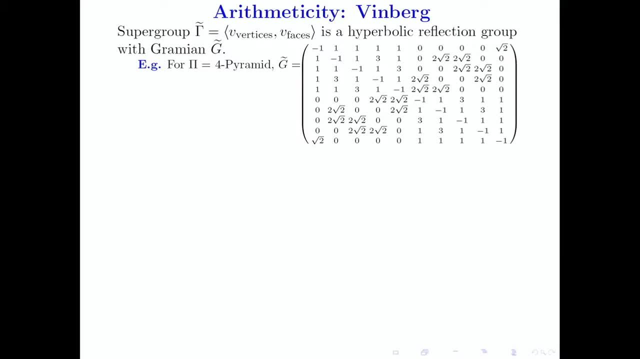 So you have some walk on the vertices, some cycle of the vertices, And every time you move from one to the other you multiply by that entry. So if I move from 8 to 7, I multiply by 2 root 2.. 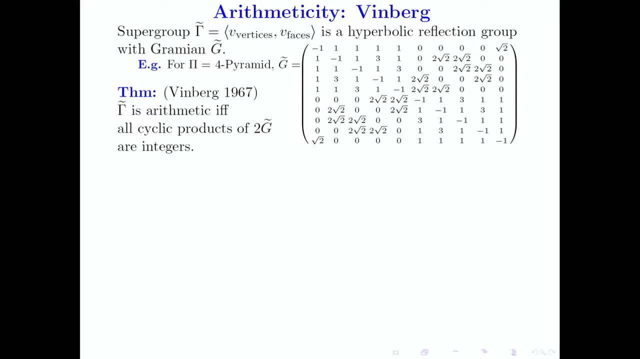 And then I move from 7 to 4 and I multiply by 3 and so on, And when you go around a cycle, what you'll notice here is, when you go around a cycle, if you stay within the polyhedron or stay within the dual, 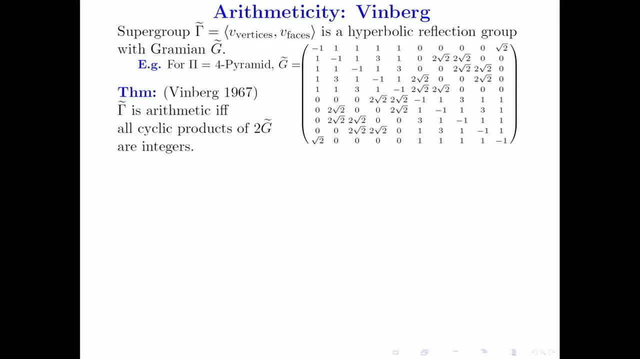 you're multiplying by integers, There's no problem If you leave. so, if you change from a dual, if you change from the polyhedron to its dual, you do it by one of these off-diagonal blocks, which means you encounter a root 2.. 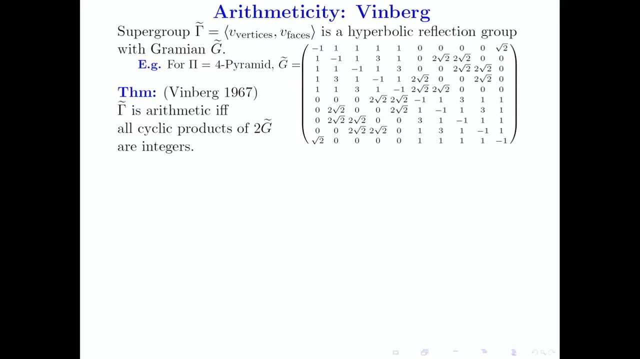 But because you have to cycle back around, you have to do it again. So the root 2s are gone. So this gramian supergramian does satisfy Vindbergh's criterion, And so this group is commensurate to SL2,. 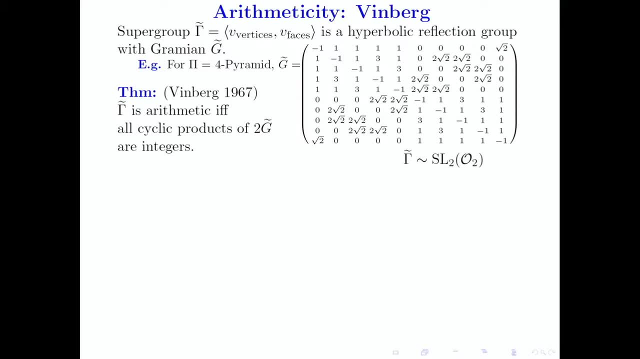 the ring of integers of Z adjoining square root of 2, negative square root of 2, and is arithmetic. So what I just explained is that the 4-square, the 4-pyramid, the square pyramid, is arithmetic and superintegral. 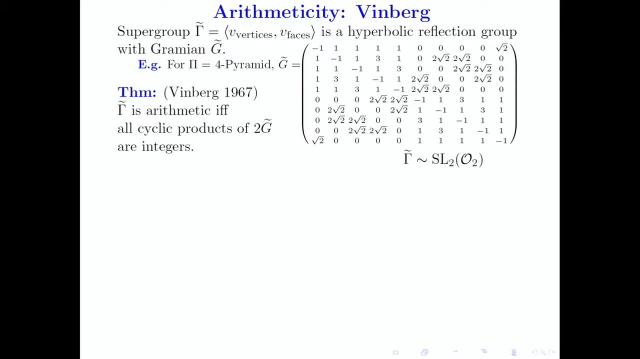 Does that make sense? So we're crucially- I'm sorry- You have one free variable to choose If you have like combinatorial data. you mentioned that matrix is not completely filled, So the matrix initially is not completely filled. 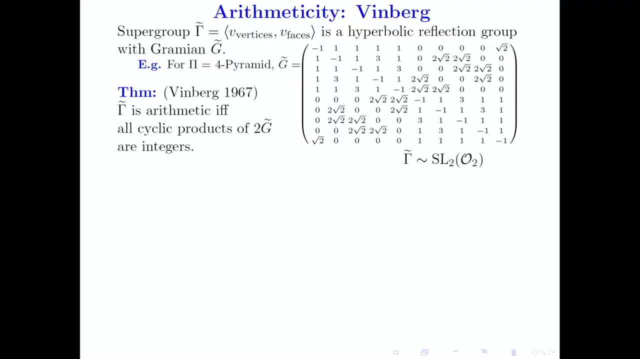 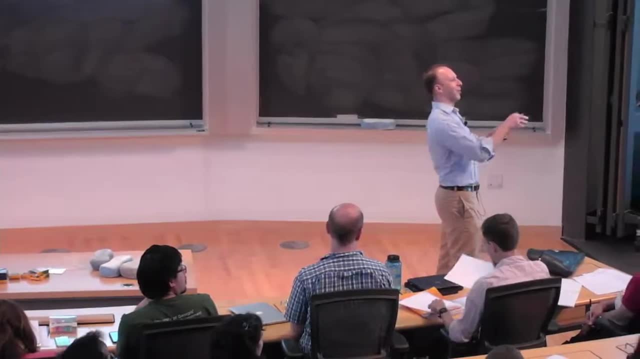 by the combinatorial data. but the Coby-Andre of Thurston is rigid and forces upon you the other entries. So the other entries are solved from the initial combinatorial data. So these root 2s and the 3s. 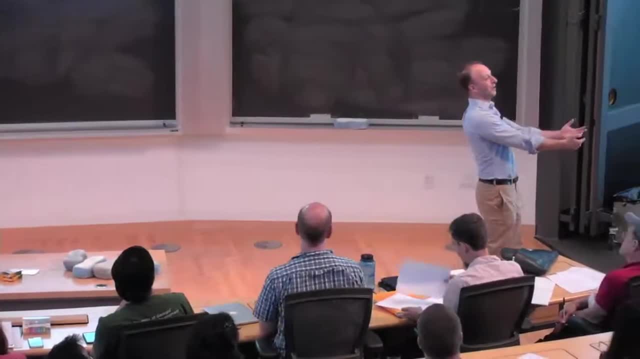 I don't have a choice. I don't have a choice about those. Coby-Andre of Thurston forces me once I say where the 1s and minus 1s and 0s are, all the other entries are determined. 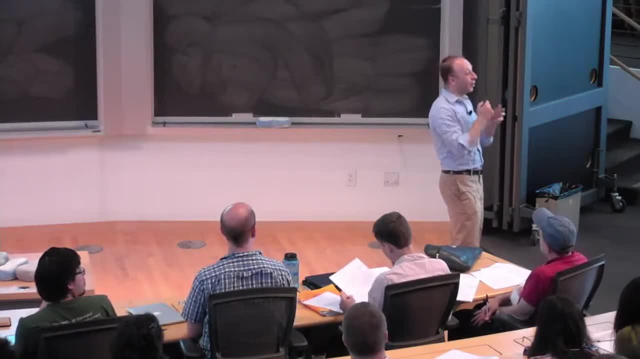 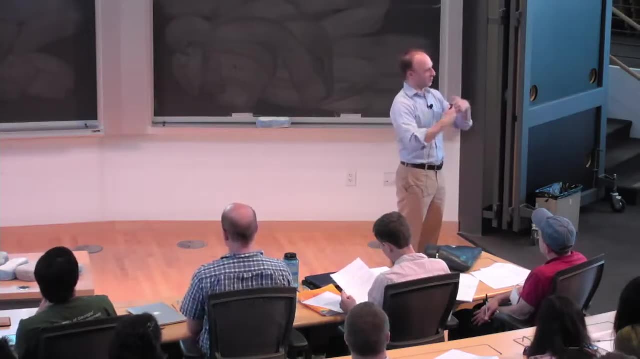 That's the theorem. So I don't have. So that's why I mean that's the guts. The guts is: how does the geometry affect the arithmetic? I give some, And really, how does the topology affect it? Because the topology determines the geometry. 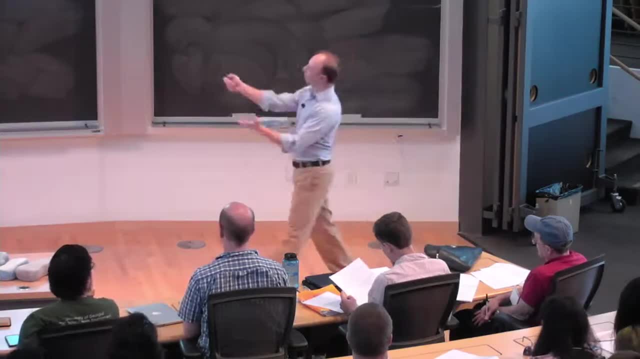 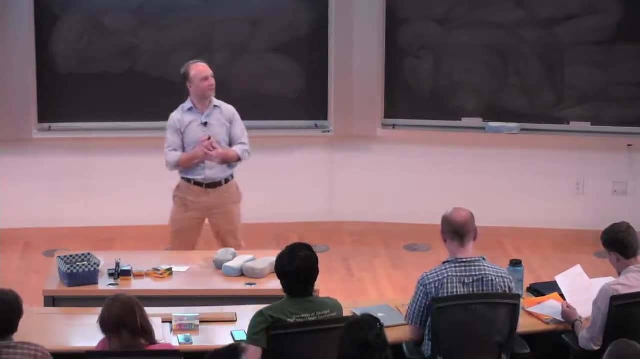 by Coby-Andre of Thurston. So this combinatorics forces these other entries, and then I have to know what's going on to the cyclic products of these entries, And if you come out with integers, then you're super integral. 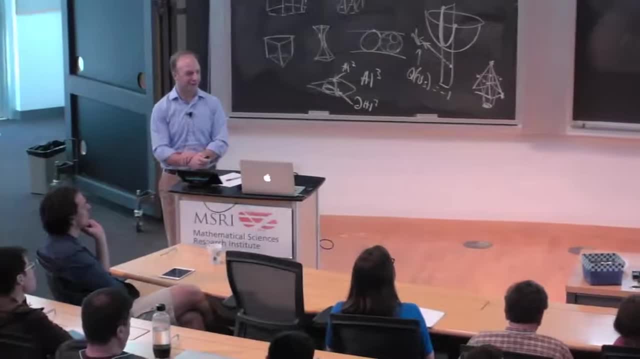 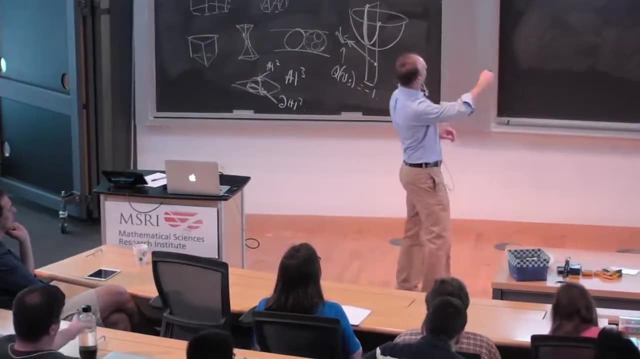 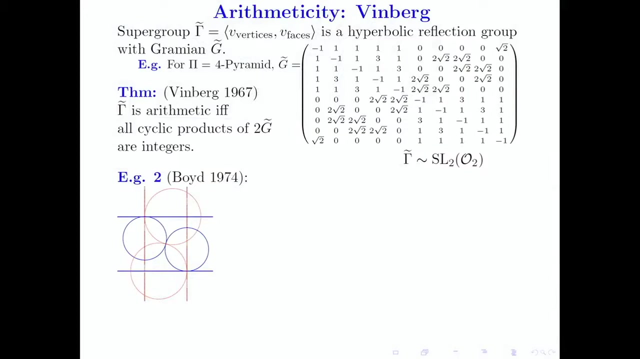 This is the key point, so I hope this is clear. Okay, So let's look at another example, because you'll see the role of a half. So this is one that I found recently in a paper of Boyd. So Boyd was actually studying what I call gamma packings. 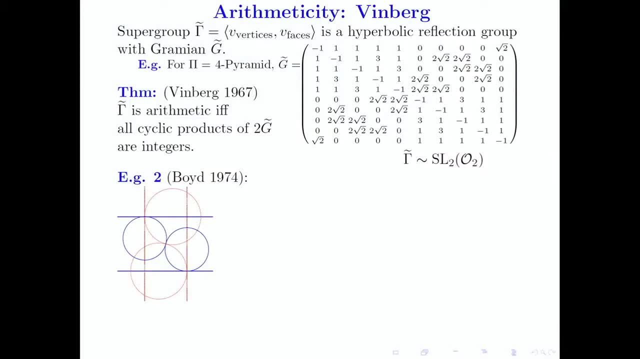 He was trying to produce them, but he wasn't giving himself the full clusters. He was only looking at tetrahedral packings. Question: Oh no, He was only looking at tetrahedral packings, So this is actually not one. 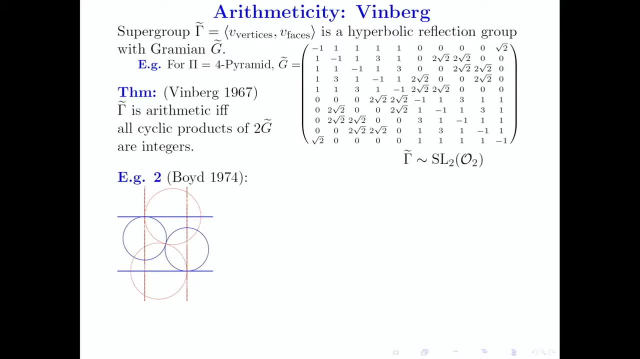 of our tangential tetrahedral packings. You can do more general things, like you can take a tetrahedron but assign distances instead of the graph, always denoting tangency. So this is a tetrahedron that I would label like this: 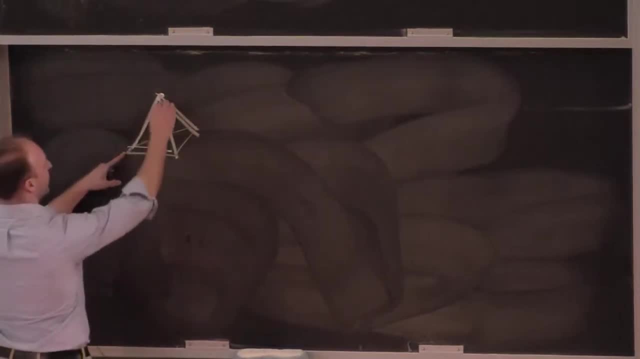 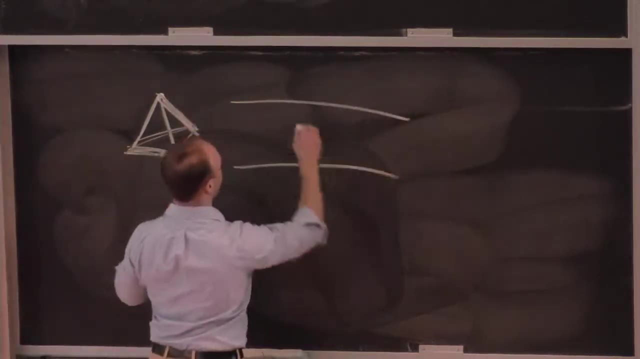 So the tetrahedron has tangency, tangency, tangency, tangency, and then these are some spaces. So I hope you can see that in the configuration there is tangency everywhere and then there's a fixed amount of space. 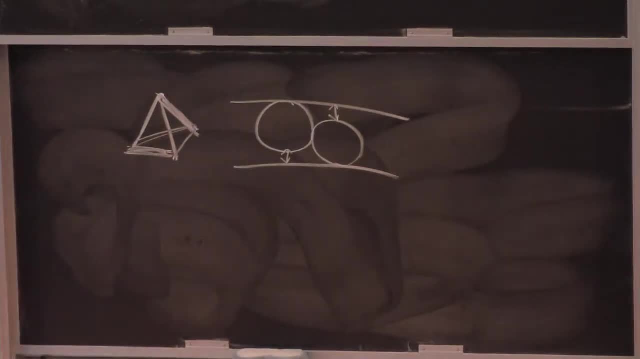 There's a fixed hyperbolic distance between the other four. So there's still only four circles. so the graph is completely determined by the structure. but I have to specify not just tangency but also distances. So you'll see that immediately in the supergrammian. 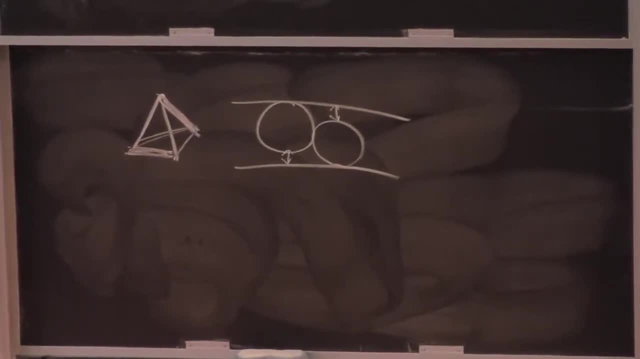 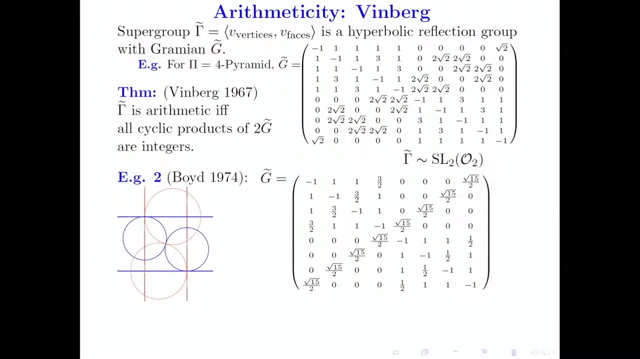 which Boyd had worked. So the supergrammian here has ones minus ones and these three halves. So you have to specify the three halves. Now, the three halves are not forced upon you. The three halves were chosen by Boyd. So that's the slight distinction. 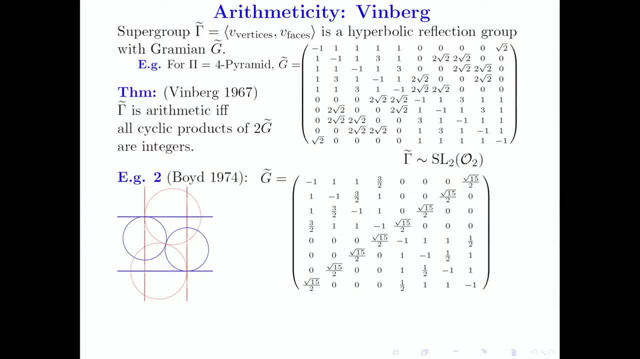 between the tangent configuration And then you solve for the rest of the grammian and you get these root 15 halves and you check that when you take twice the grammian and you take any cyclic product again, the root 15 is your only problem. 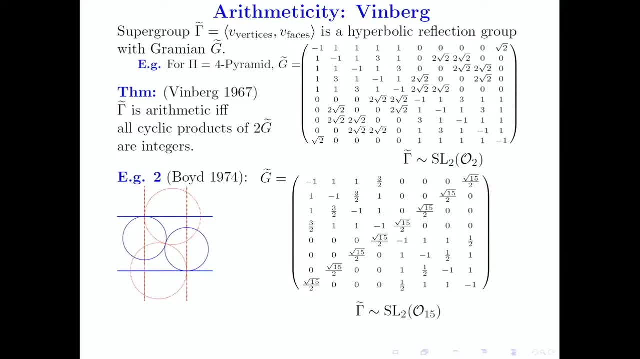 but it always comes in pairs. So this is also superintegral and commensurate with this Bianchi group. And what Boyd wasn't interested in at the time, I guess, is the integrality. so this is another superintegral circle packing. 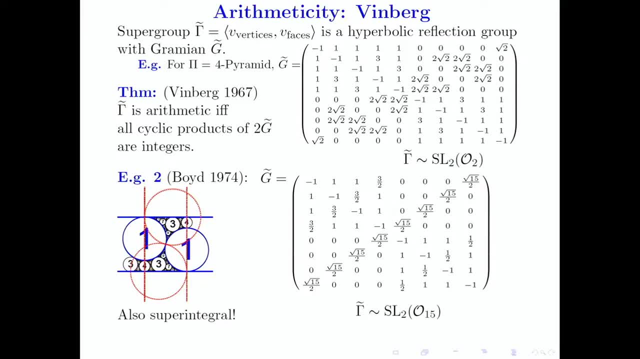 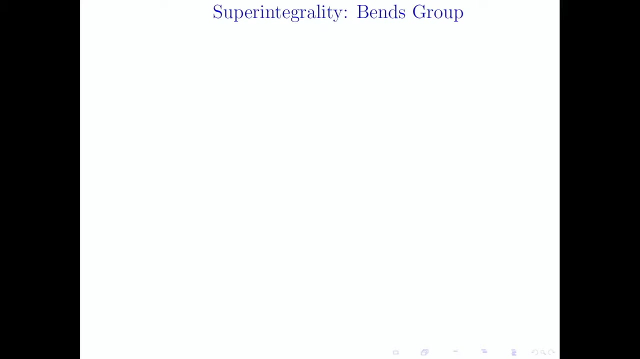 which satisfies the superpack conjecture? Okay, Okay, so any questions on where we're gonna get arithmeticity from And the role of this supergrammian? Okay, so where do we get the superintegrality? So I have to explain what the role of Ben's group. 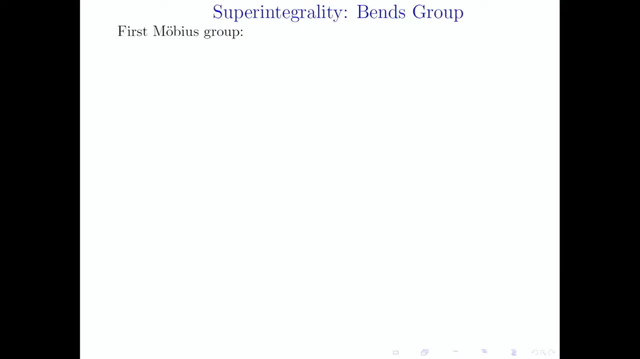 The Ben's group, which in the Apollonian case is called the Apollonian group. So first let's talk about the Mobius group. We remember what is a reflection through one of these spheres. This reflection, so the sphere, determines a hyperplane. 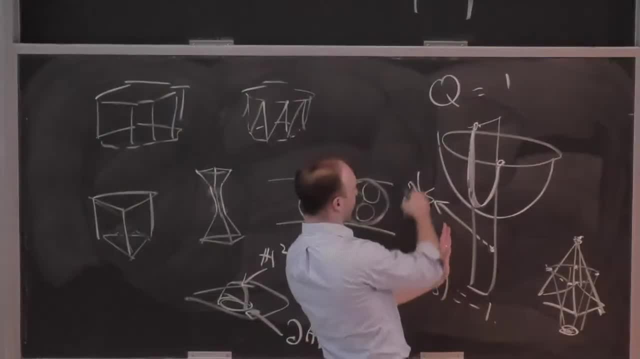 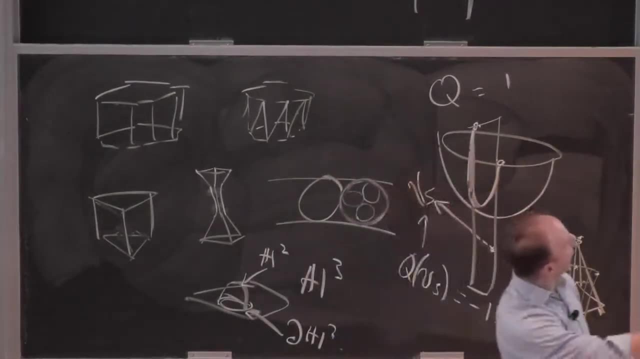 and the hyperplane determines a normal vector, or the other way around, the sphere determines a normal vector, if you like, And then reflection is literally reflection through this plane given by this formula. So this is a linear, the whole point of using inversive coordinates. 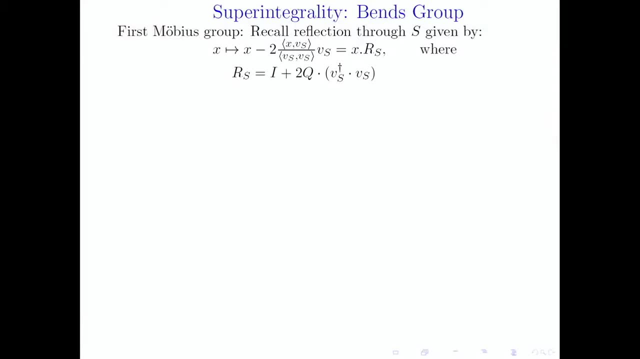 is that Mobius transformations, which are fractional linear, they're not linear. they're fractional linear, But once you use inversive coordinates they become linear functions. These extra variables linearize the operation and it's very easy to see that this map is obtained by taking x and multiplying it by the. 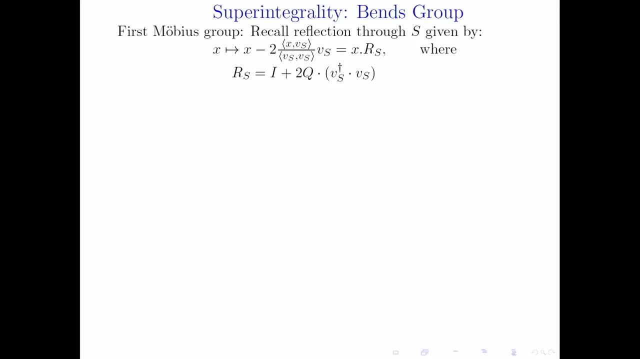 matrix. so in the case of circles it'll be four by four matrix identity plus twice q. and then- this is a funny thing to do- you take a column vector, multiply it by itself as a row vector, So you get a rank one n by n matrix. 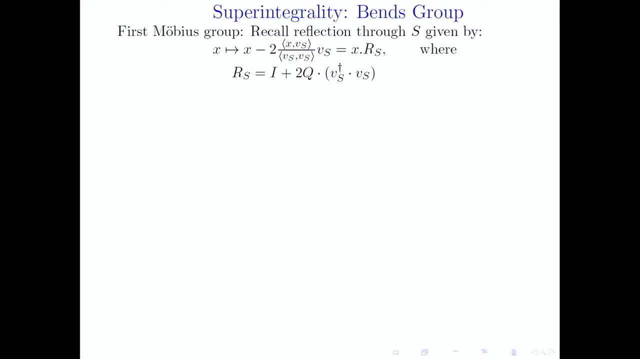 you multiply that by q and add to double it and add to the identity. So this is going to be a matrix by construction in the orthogonal group, preserving q Or the extended orthogonal group. Okay, Then the symmetry group. remember, we have this gamma. 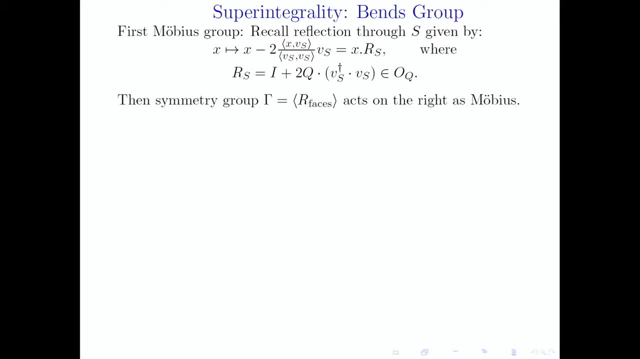 the symmetry group acting on the packing is the group generated by reflections through all the faces And that acts on the right, as here, by these Mobius transformations. These are all Mobius actions. So if you have a cluster, if you have a cluster modeled on your polyhedron, 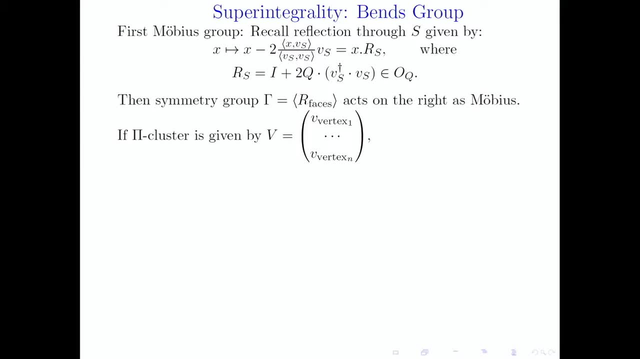 and it's given by these vertices, these vectors, v these normal vectors, the bends. you remember what each of the vertices looks like. it looks like bend, co-bend, bend-center. The bends are in the first column, But the Mobius group is acting on the right. 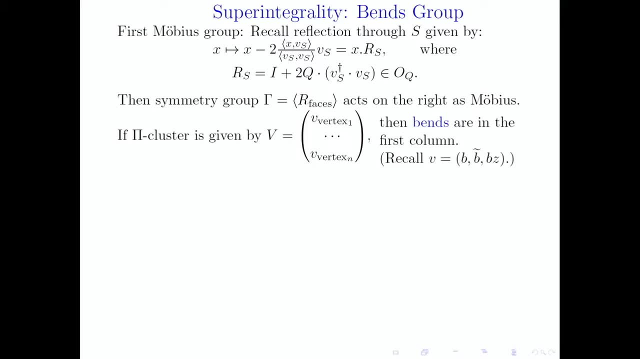 So that's not acting on columns, that's acting on rows. I want something acting on columns. This also I learned from Jeff's paper: that you should study the left action and not the right action. So if you want to understand the bend action, 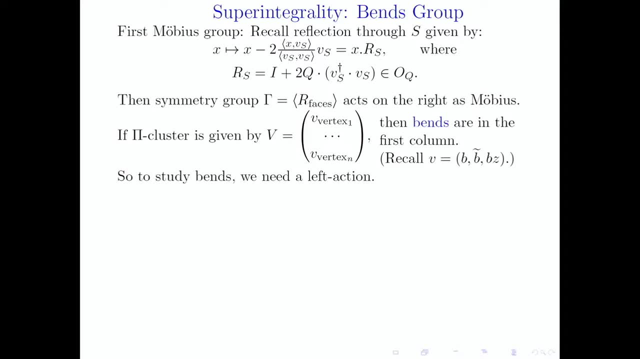 to understand superintegrality, you need left action instead of a right action, and you get that by just writing the equation. I have these vertices, I have these, you know, geometrized circles, and I want the Mobius action of a given sphere. 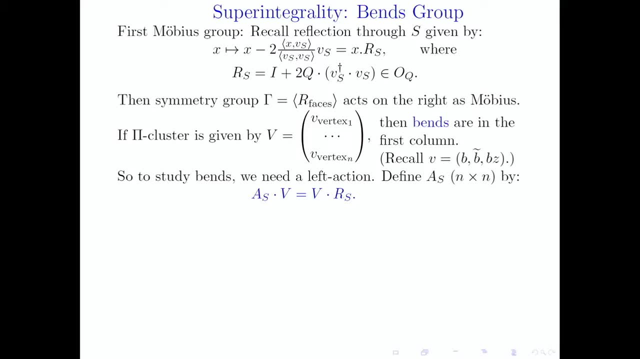 on these vertices to be the same as some left action on the same vertices. So there's going to be a left action which is corresponding to the right action by Mobius, And the important thing to note is that, well, wasn't there a choice? 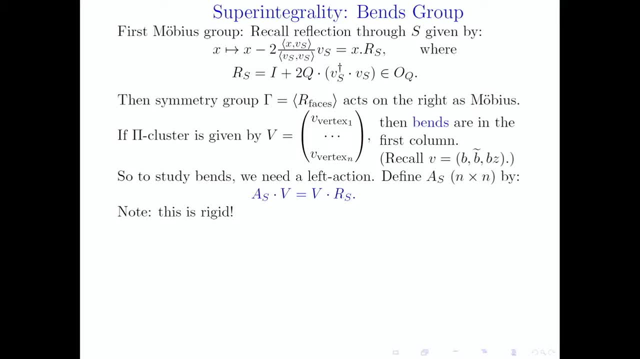 you know which particular vertex, which particular axis, because all the vertices are rigid up to Mobius transformations. but once I take Mobius transformations, V is changing but R is also changing by a conjugate of the same Mobius transformation. 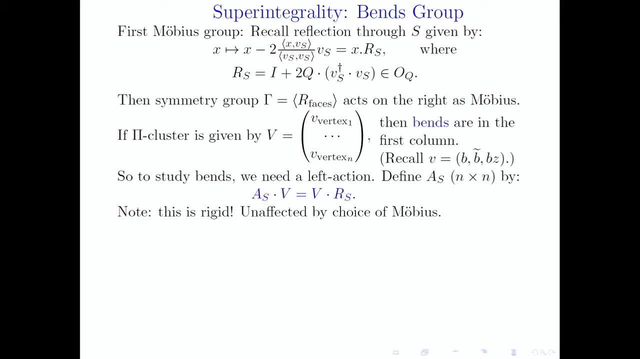 So this equation is actually conformal. Okay, It doesn't depend on the choice of the initial configuration up to Mobius, But the distinction between what Boyd and others were doing was that they were only studying tetrahedra, If you allow larger clusters. 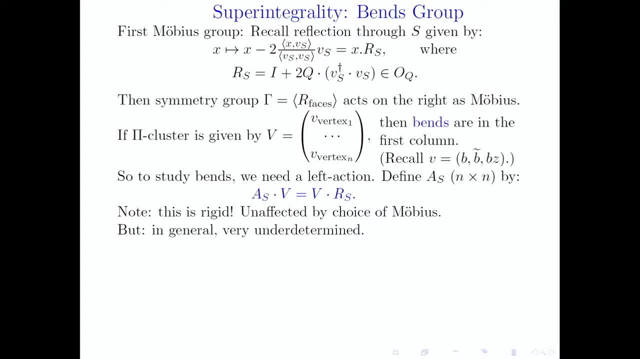 then this equation is underdetermined. So A is an N by N. matrix of rank. Oh, I have too many Ns. N is the number of faces, but N is also the dimension of the. so let's say this is capital N. 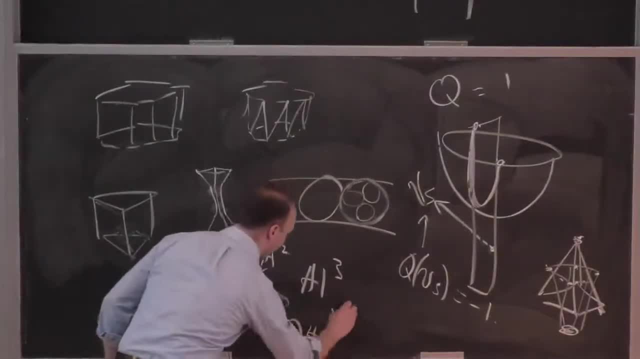 So I have spheres. These are spheres in capital N, which is S N minus one, And this is hyperbolic N space and hyperbolic N plus one space. So the rank of this thing, or the rank of V, is capital N plus two. 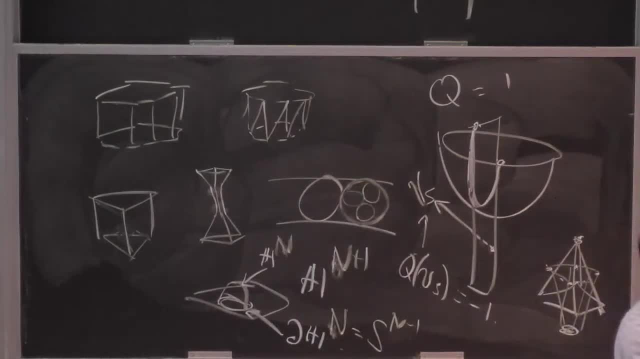 but A in general can have many more entries. Little N can be many, much, much larger. So let me just show you an example of that. The four pyramid is the first example where the ranks, where the thing is underdetermined. 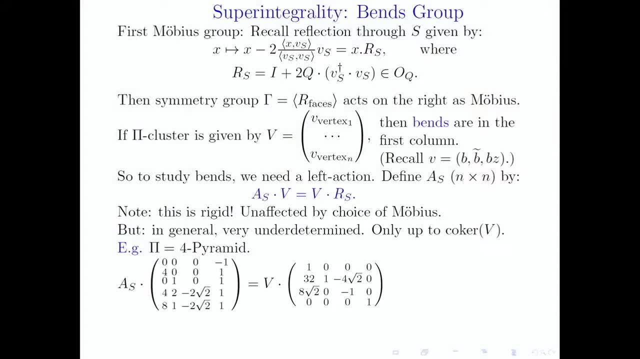 So let's look at this equation. So what's the? so these are the vertices. You remember, I'm taking the bend, co-bend and bend-to-bend, So this is the bend, co-bend and bend-center. 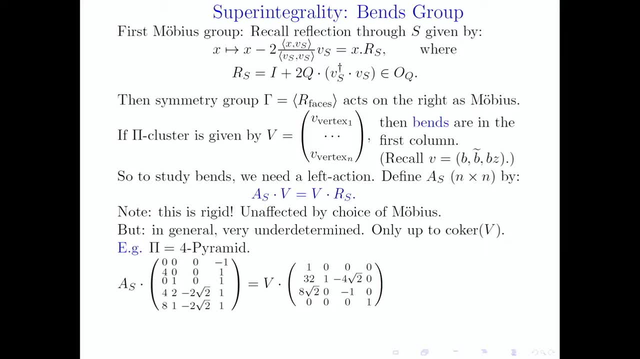 Well, when the bend is zero, that's the limit of a sphere going to infinity. So it's actually the normal to the plane. So this is the following configuration: Zero, zero, zero negative one is the normal vector: zero, negative one. 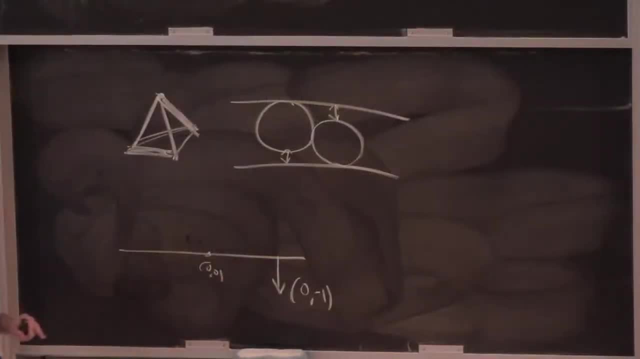 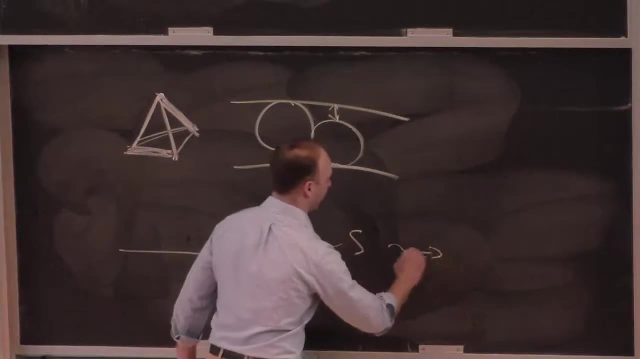 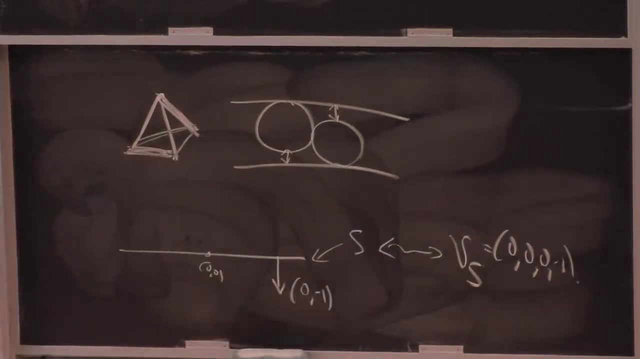 which goes through the origin. So that's this horizontal line. Okay, so if this is your sphere, this is your oriented sphere, then the corresponding normal vector is zero, zero, zero negative one. And then there's another one here at some height. 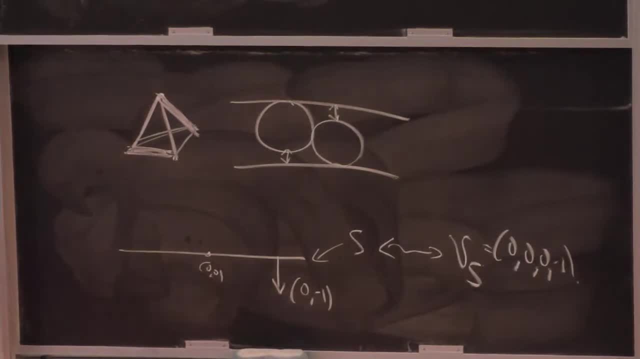 So the co-bend is still zero. Let me not bother drawing the configuration. I'm sure I'll get it wrong at this moment. But this is the Mobius action. So it's a four by four matrix, And what I'm looking for is a five by five matrix. 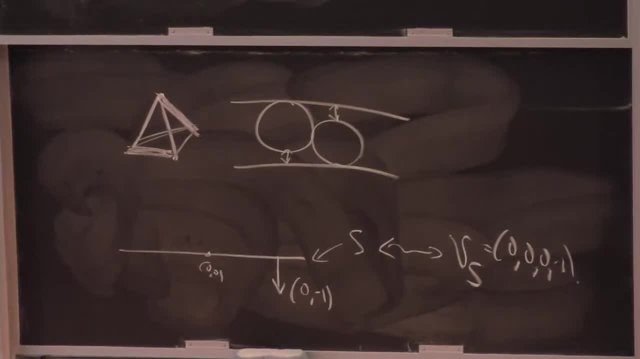 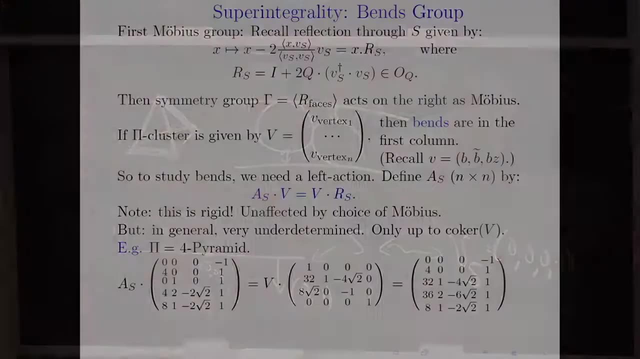 that realizes the action of a four by four matrix. Obviously there's a co-kernel And if you stare at this thing, well, you can kind of see what's going on. I'm looking for matrices that will realize this And I have some choice of how to find them. 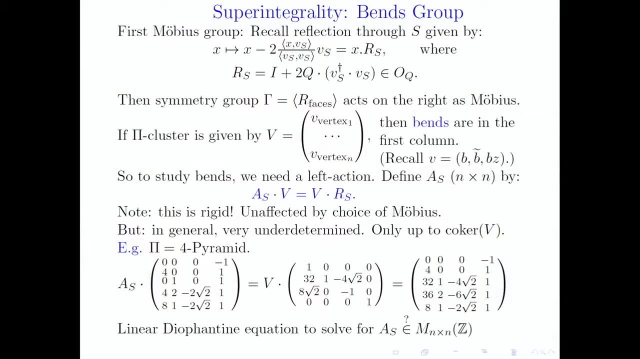 But what is this? This is just a linear Diophantine equation. So superintegrality is a question of linear Diophantine equation. Once the data you get out of Kobe-Andreev-Thurston tells you what these vertices are and what these Mobius transformations are. And then you have to solve: can I find an end by end matrix in the integral? And then you have to solve: can I find an end by end matrix in the integral? And then you have to solve: can I find an end by end matrix in the integral. 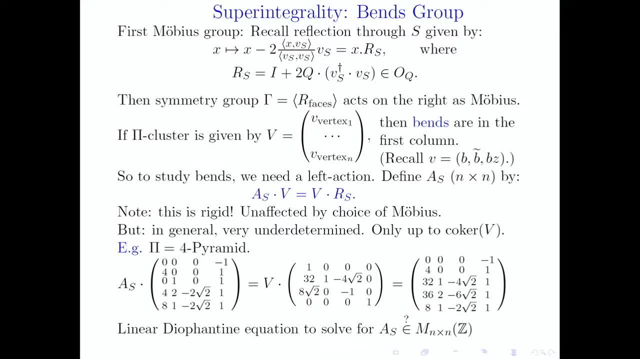 And you have to solve. can I find an end matrix in the integral Which realizes this right action on the left, which realizes this right action on the left? Okay, so this is a linear Diophantine problem. And if all of these matrices are integral? 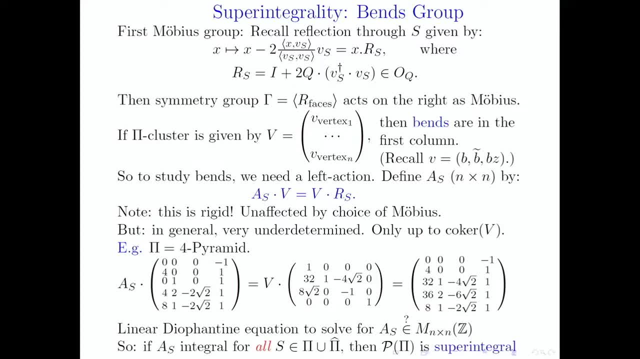 for every sphere, both in the packing and the dual packing. then you're always moving the bends by integers. So again you have this integer linear combinations. And that's what's going on in the Apollonian packing. It's that both the dual and the 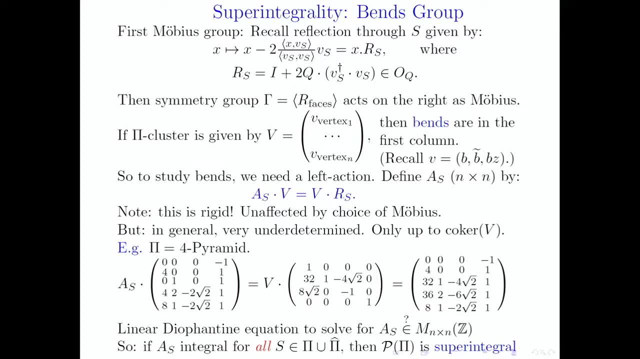 Both the original polyhedron and the dual polyhedron have all integer bend matrices, so the bend group is completely integral. Does that make sense? I think I have another example. Oh, I have a non-example. Let me show you this non-example since I'm almost out of time. 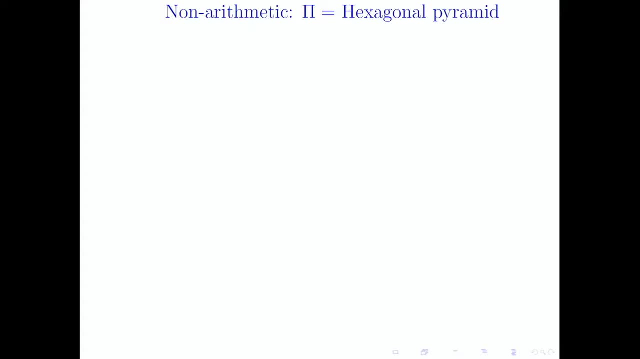 So what's going on with the hexagonal pyramid, which is related to the hexagonal bipyramid, which is dual to the hexagonal prism, which was the guy I promised I would tell you about? So here's what's going on. 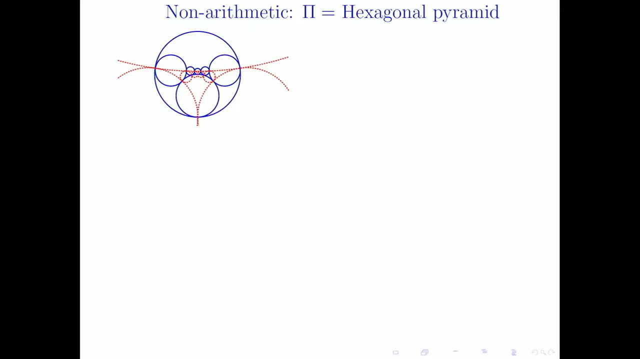 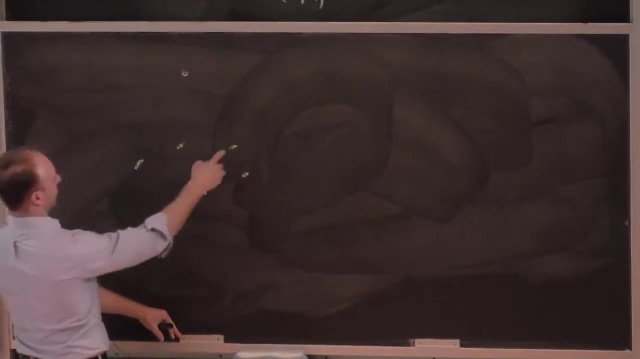 So here's a geometrization of a hexagonal pyramid. So this, Where's my sixth pyramid. So the sixth pyramid is a hexagon. on the bottom, One more And then everybody reaching to the top. Okay, So the outermost circle is the top circle. 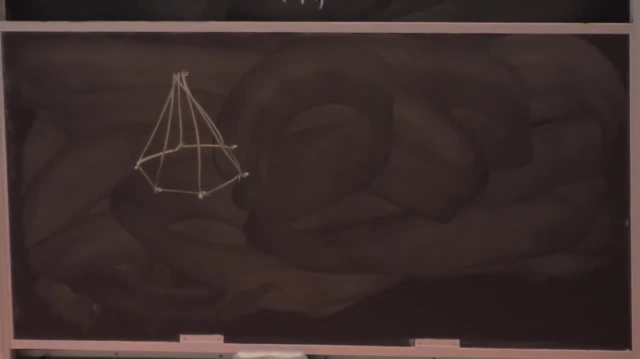 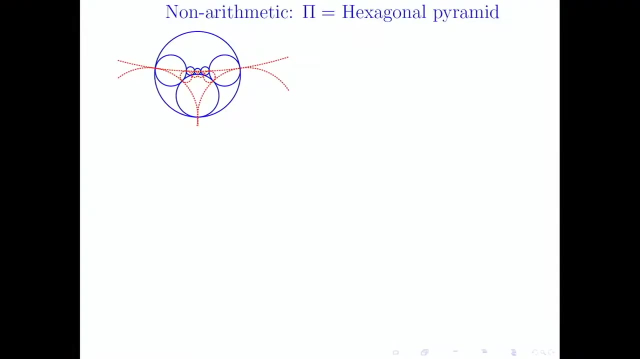 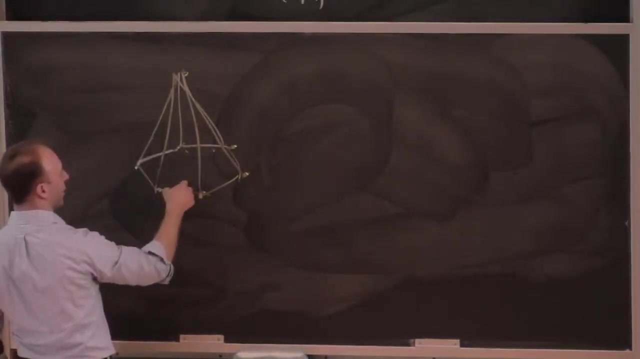 Sorry, Who's the top circle, This circle here? This circle is the top circle because he's touching all the other ones, Is that clear? And then the dual again will be a hexagonal pyramid, because you have six triangular faces all touching a single hexagonal face. 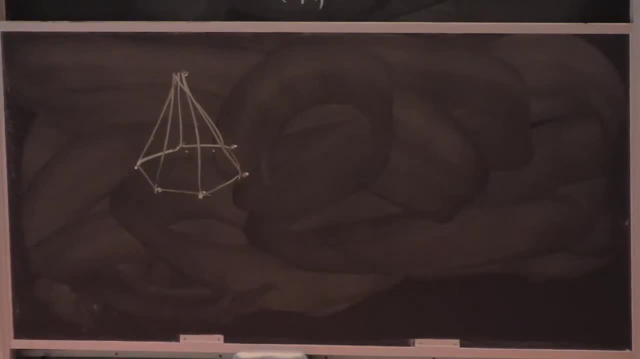 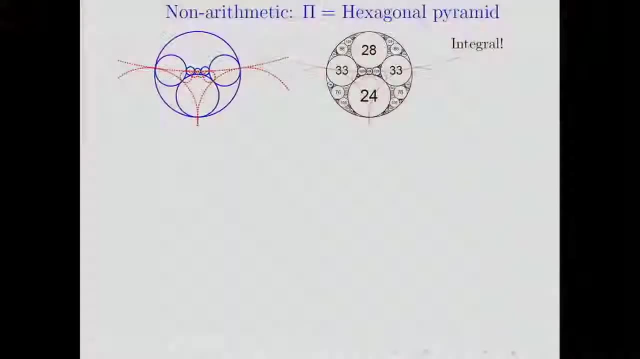 So that's what the red guys are: the dual. And again, when you act by Mobius transformations, this is the packing that you get, And maybe you don't. You don't believe me, but if you look a little bit more closely, 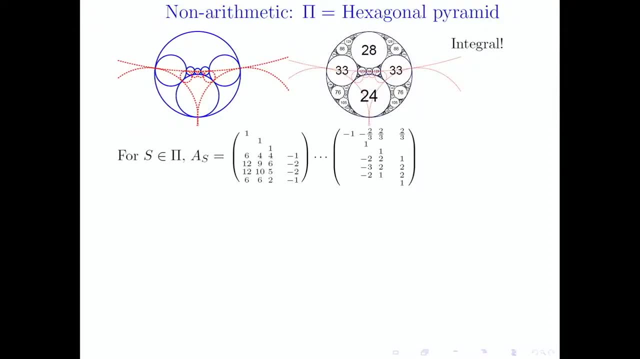 you get integrality. Now let's look at the bend matrices. So the bend matrices that come out will be seven by seven matrices. Seven because there are seven vertices of a hexagonal pyramid, But they're rank four because they're circle packing. 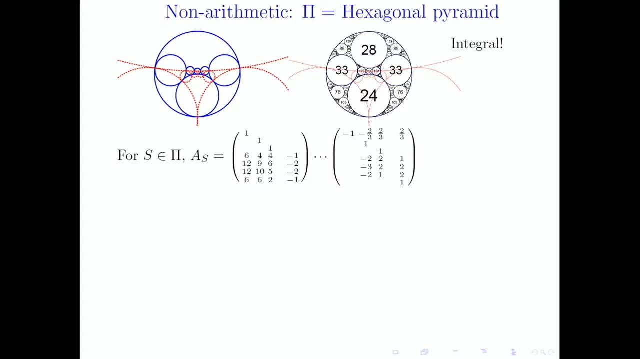 So it's seven rank, you know. so there's some choice here, And you can't quite make them all integers, but you can make them all. at least for the polyhedron itself, you can make six of them integers, and the last one will have these denominators three: 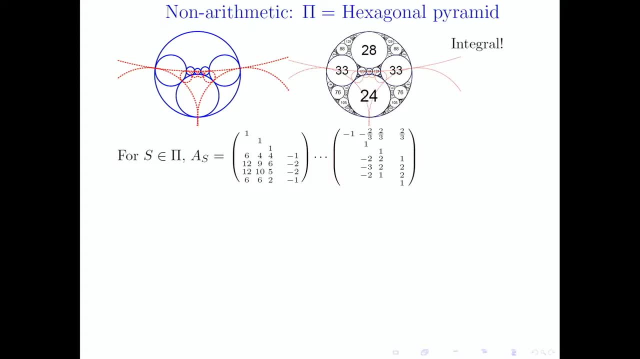 You can make six of them integers and the last one will have these denominators three. And the funny thing is, when you act, when you take multiples of these matrices, you see these guys all have, all are multiples of three. So those denominators three don't grow. 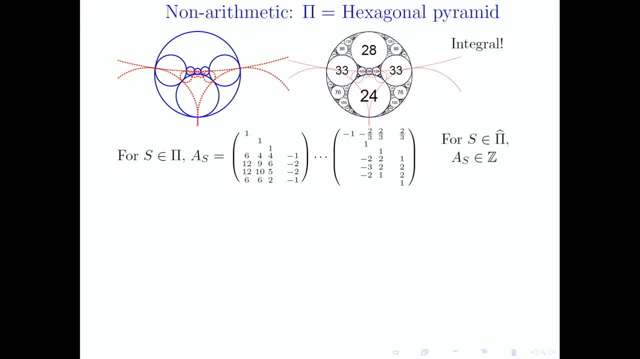 That's what's responsible for the integrality And, by the way, for the dual packing. all of the matrices are also integral, So you should start thinking that maybe this thing is super integral. But then you look at the Gramian and the Gramian looks really good. 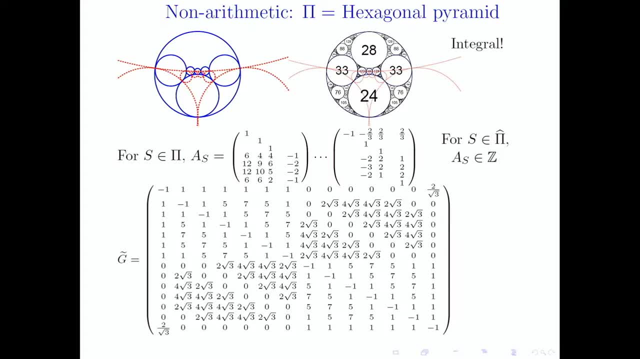 These are all integers. These are all integers. And then on the off-diagonals I have some square root threes, But again I just get them twice as they go around any cycle. But again I just get them twice as they go around any cycle. 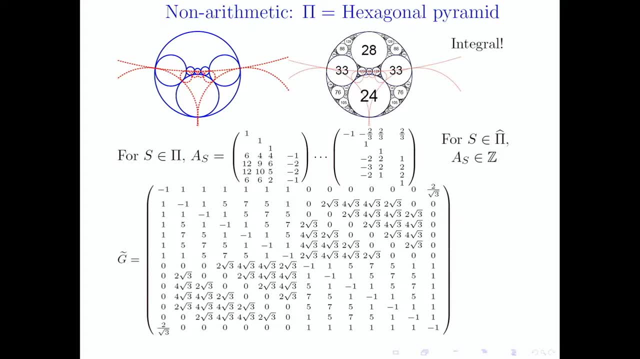 So it's arithmetic right. There's a denominator root three. You do this one twice, you get two thirds or four thirds. You're not allowed to have threes in the denominator for arithmeticity. So what's going on is that this piece. 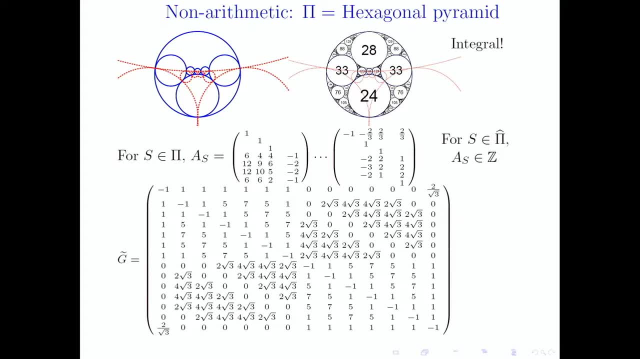 piece of the. so if you think about this non-arithmetic group as a lattice in hyperbolic three space, there's a piece of it that's acting discreetly and integrally. There's another piece that's also acting integrally and discreetly, but when you have the two together. so these other, 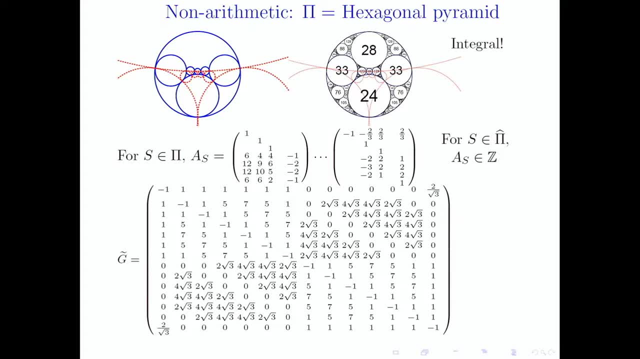 matrices which I didn't write down, for you don't have this property, that these entries are divisible by three, and so when you start acting, when you start playing between the dual and the original polyhedron, these threes start to build up, and they build up forever. so that's why. so this is. 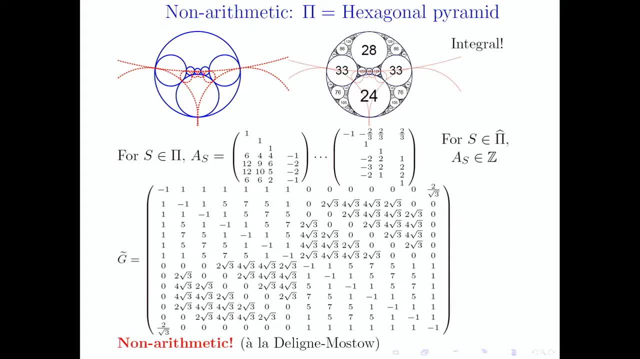 non-arithmetic. and this is why it's a type of Deligne-Mastow example, because they were looking at s-arithmetic groups which how do you construct a non-arithmetic group? Well, you make an s-arithmetic group, but then you force it to already be a lattice in the first factor It's supposed to be dense in. 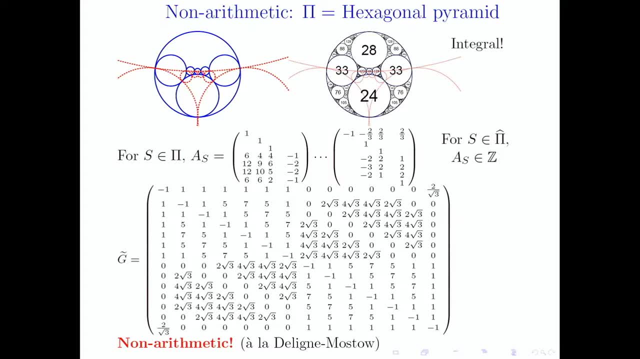 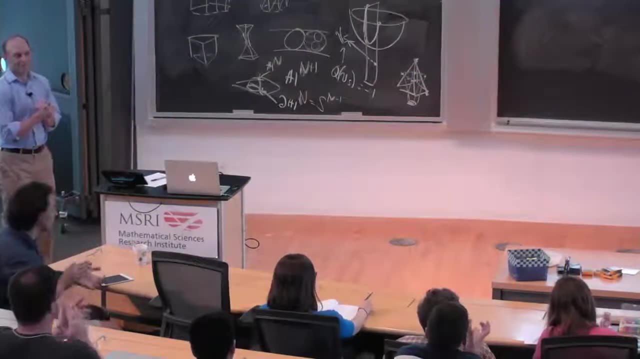 the first factor If it's actually a lattice in the s-arithmetic group. so this is a an example that's. that's like that one. Okay, so I'm out of time, let me stop there, Thank you. Thank you for the talk. Any questions? 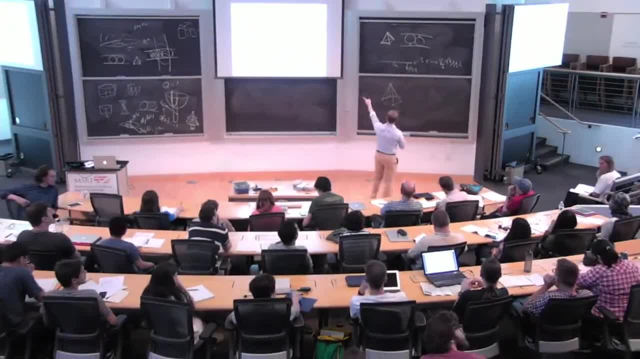 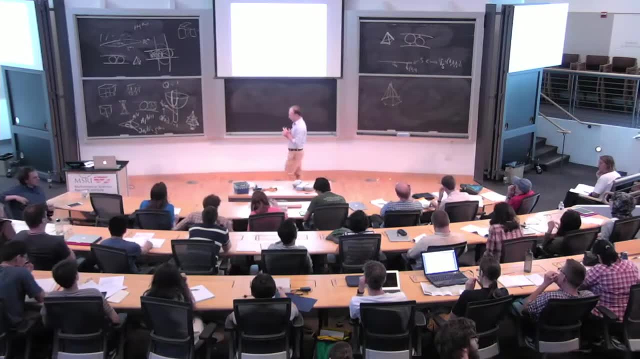 You said a word or two about how you came to your conjecture. This is how he came to the conjecture, But why should I? Okay, so what should be happening is that, if you're superintegral, it should be coming from. 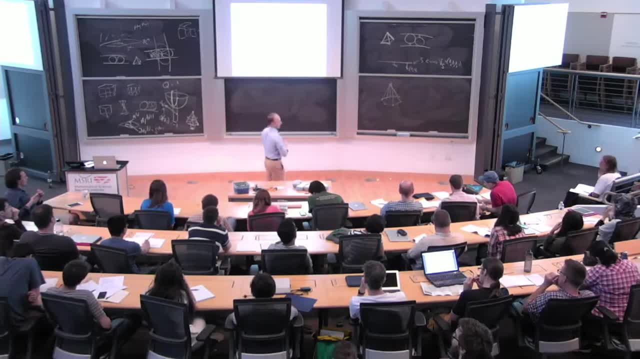 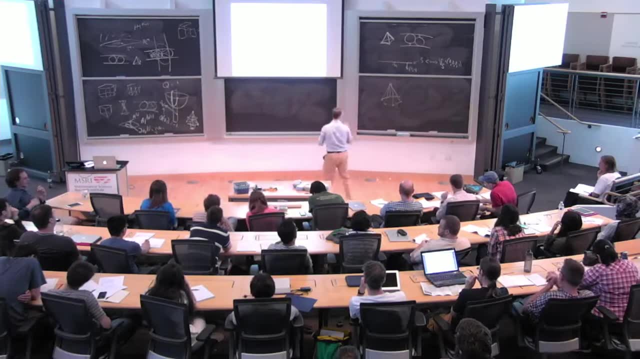 there should be some realization of these bend matrices, which is completely integral, And if that's the case, then that should itself be. I mean, it's a conjecture, right? So I'm telling you what I think should be happening. If that's the case, then it should be forcing. 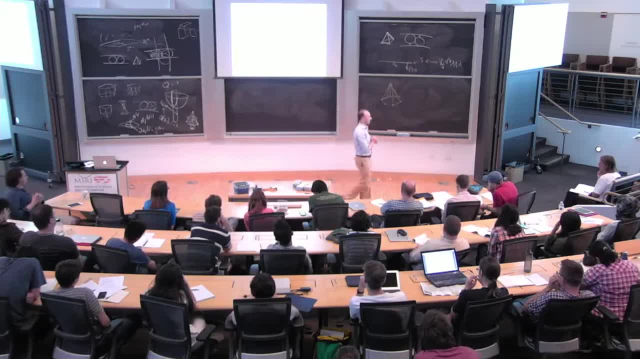 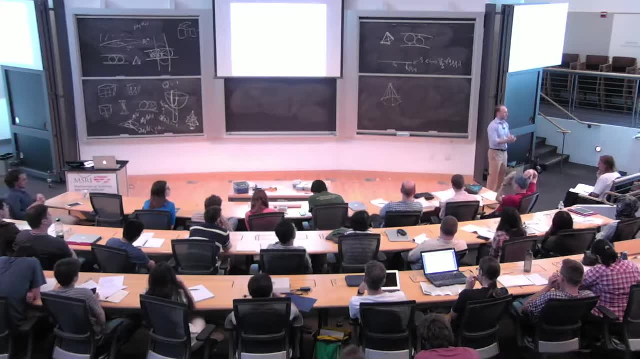 the Gramian to have the Vinberg criterion. So that's what we would like to show And at the moment we're doing it by example. We're just, we're plowing through all arithmetic groups known to have reflection to be commensurate with. 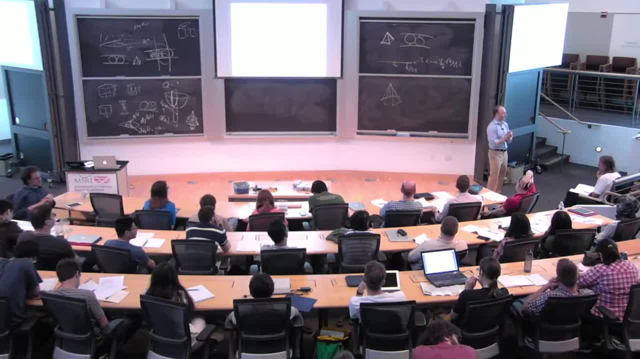 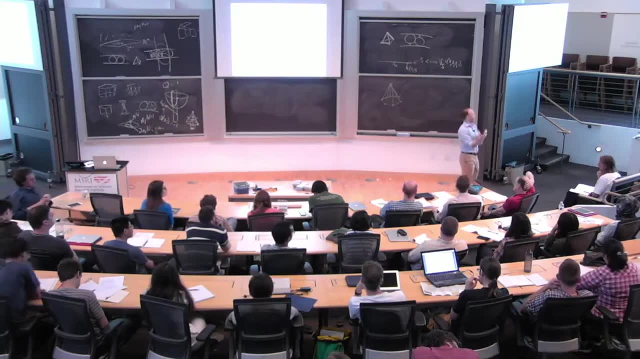 reflection groups and seeing which of them support sphere packings. So we have a lot more examples than what I showed you, but the general theory is finally forming And the right question seems to be not integrality but superintegrality, for exactly this reason. 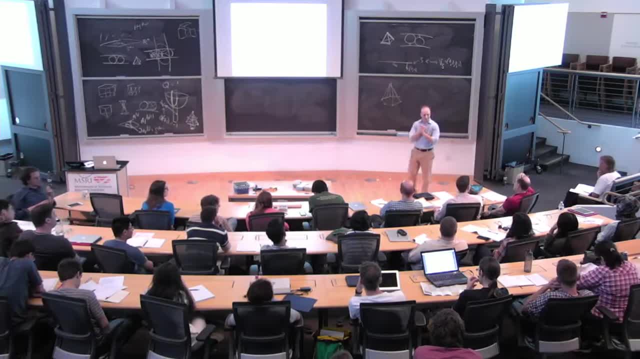 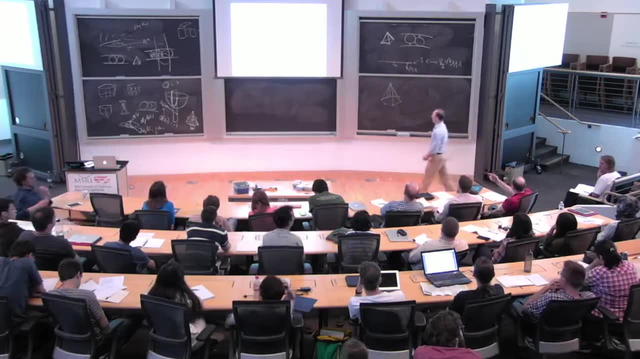 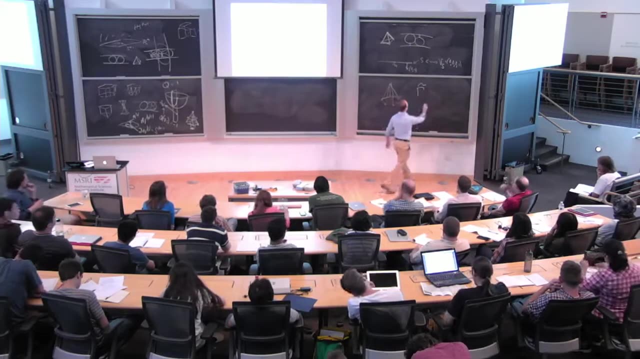 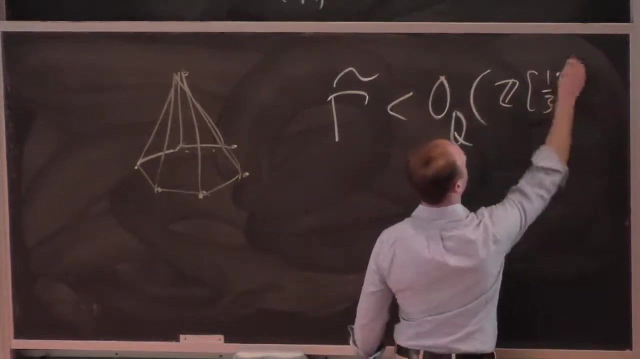 Jeff, This example here at the end is S-arithmetic, but it's not arithmetic, So it's right. so we have this group, gamma twiddle, right, It's a subgroup. it's certainly a subgroup of O, Z, a joint, a third. So what I would like to do is see it as a lattice. as a lattice. 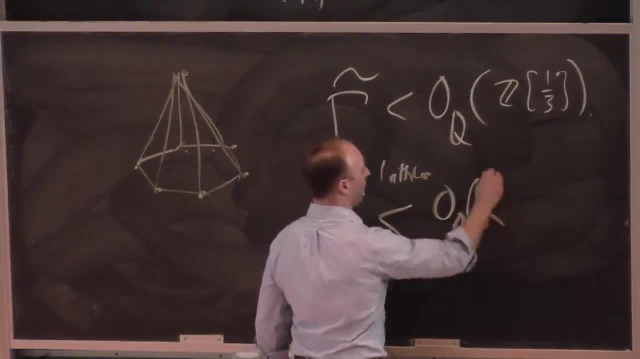 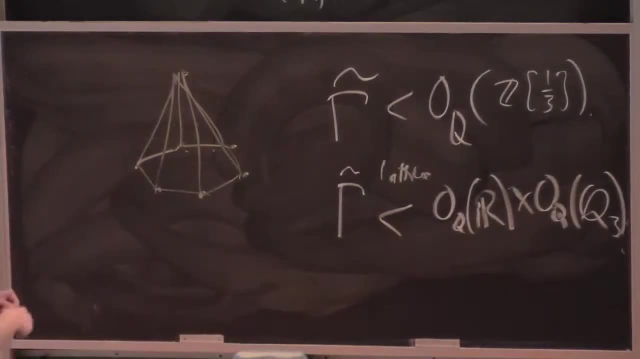 in OQR cross OQQ3.. So these denominators- threes, if you, if you put it like this, then the denominator, the three denominators that are that are ruining your integrality, aren't ruining anything. right? That's what it means to be S-arithmetic is to be a lattice in here, But this is not a lattice in here. 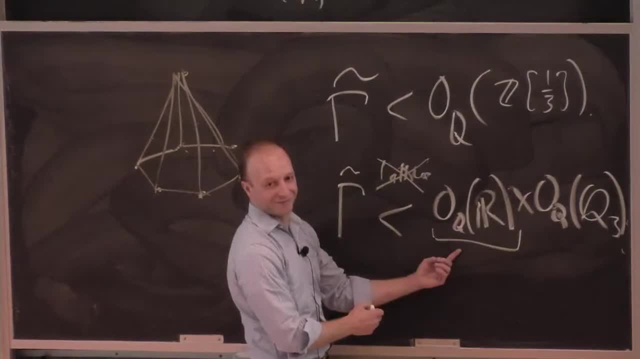 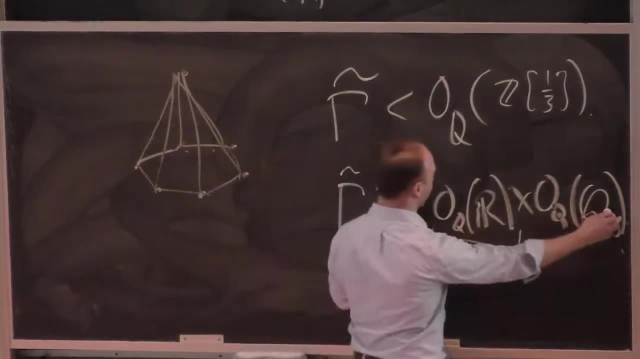 because it's already a lattice in the first factor. That's what these D'Aline-Mastau examples of non-arithmetic groups were. They constructed S-arithmetic groups which already were lattices in the first factor and hence had to be thin in the in the product. 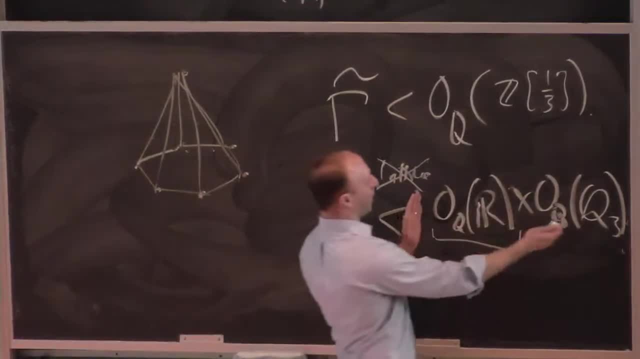 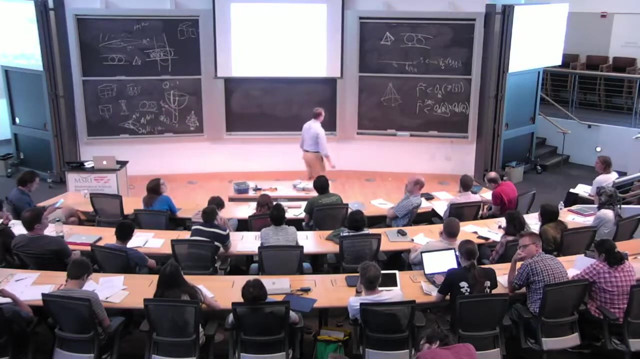 So it's actually a thin group of the S-arithmetic group because it's already a lattice in the first factor and that's what makes it non-arithmetic, if that makes sense. Yeah, Male Participant 264. So so you're asking about the Descartes theorem, The relation between the bends. 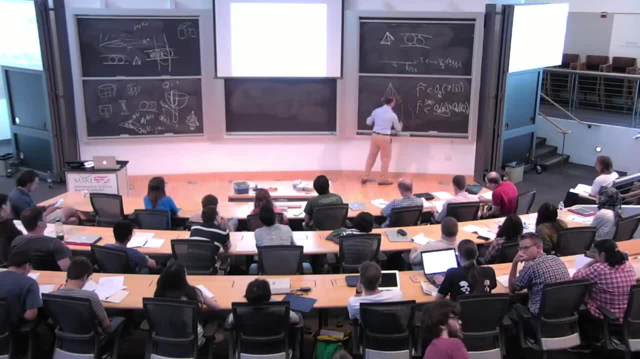 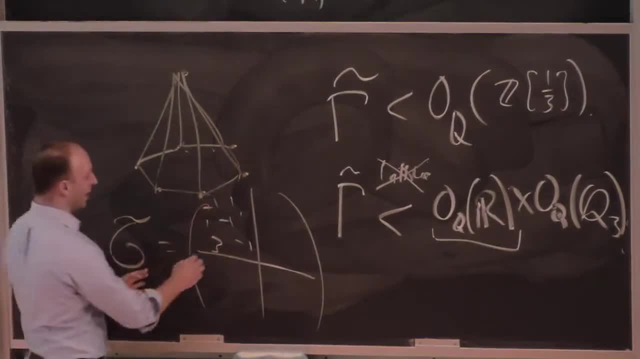 The Descartes theorem is nothing more. so we have this Gramian, which is the, the. there are some entries that are forced upon us, and then there were other entries that came out of the proof. The Descartes theorem is. 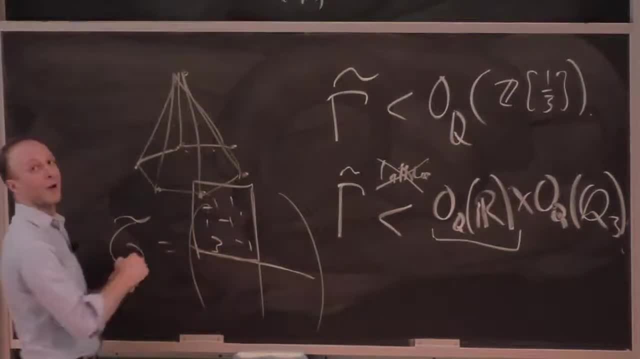 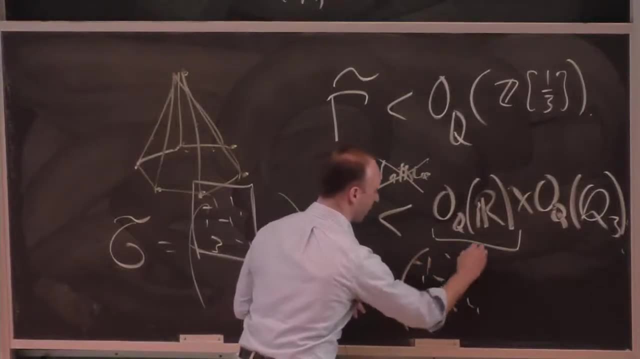 nothing more than the 1, 1 entry of the inverse of this piece of the Gramian. So in the case of the Apollonian packing, you had minus 1s and then 1s everywhere And there was nothing indeterminate because it's a tetrahedron. So the inverse of this matrix is actually: 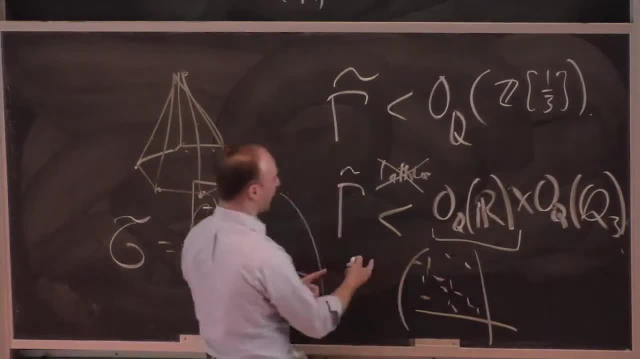 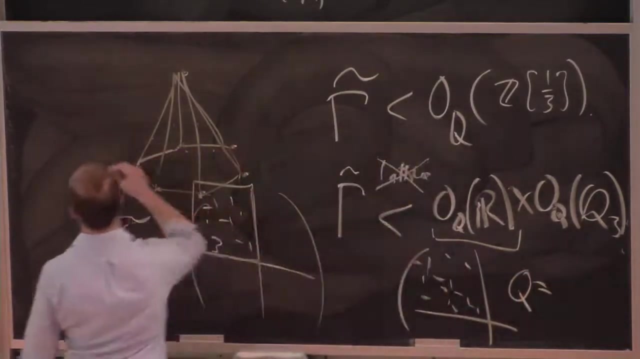 itself. And the 1, 1 entry is: if you work out what this form is, it's the sum of the squares minus half the square of the sum equals 0.. And it equals 0 because the inverse Gramian is related. So there's the bend. If you take the bends and you measure them by the inverse, 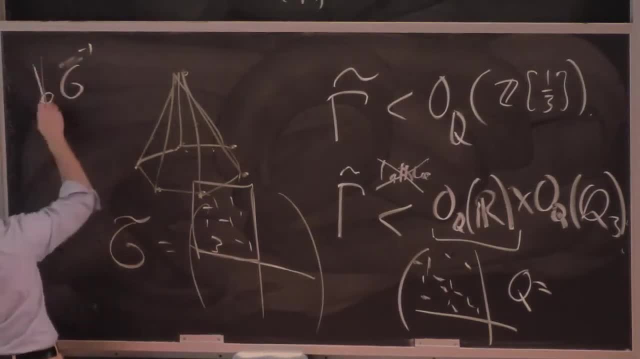 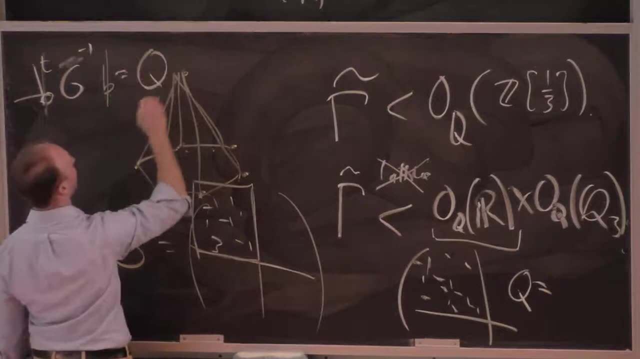 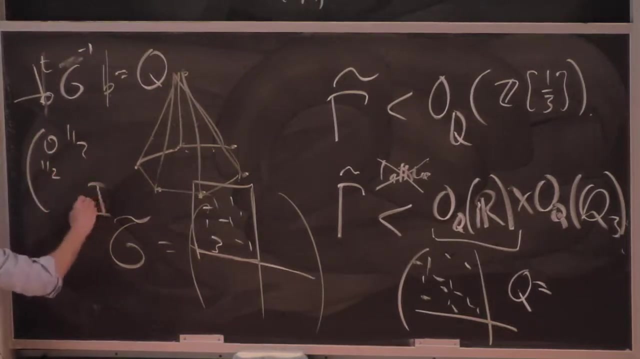 Gramian, not the super Gramian, but the inverse Gramian. So this is the bend column vector. No, I don't want to do that Transpose. So the transpose of this column vector will be q And q. well, it'll be the 1, 1 entry of q And, if you recall, q had a 1, 1 entry of. 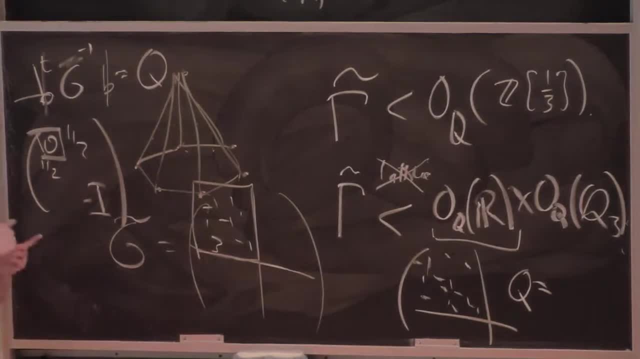 0.. So that's why the sum of the square is minus half, the square of the sum is equal to 0.. Now if you go to hyperbolic, if you pack not the real plane but a sphere, or pack hyperbolic, 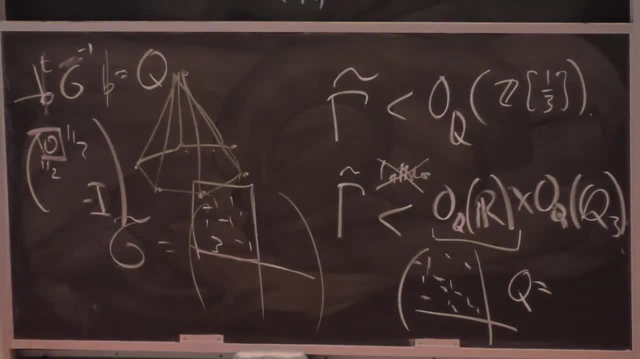 space, then q changes And then the sum of the square is minus half. the square of the sum will be negative 1 or positive 1.. This is worked out in Ligarius and Mallows, Wilkes, Yann Graham. I think I got everybody. Good question. 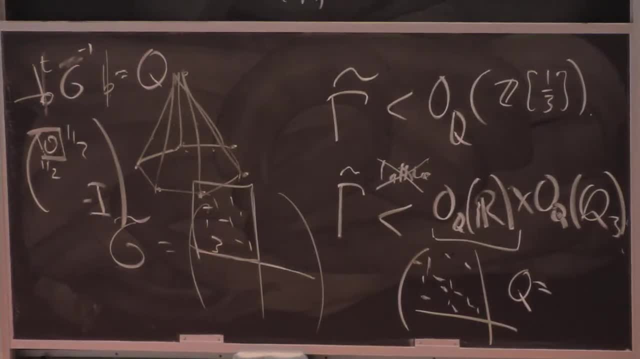 Yeah, so you mentioned at some point that the Covey-Andreyev-Thurston result gives you a unique solution for the super Gramian. Yes, But at least as I recall and wrote it down, there was, or, let me ask, is there a uniqueness? 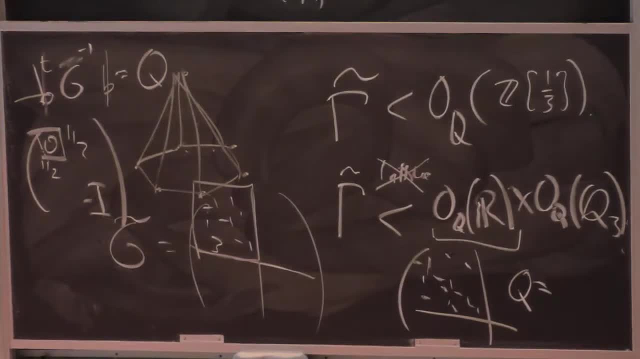 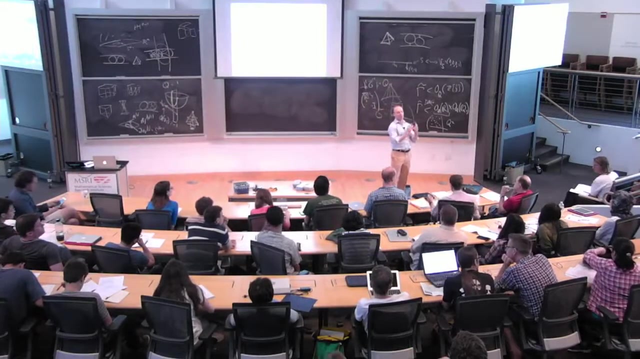 condition in their theorem. So the uniqueness condition in their theorem is that the polyhedron be triangulated. That's the distinction between Covey-Andreyev-Thurston and Schramm. So the way I stated, Covey-Andreyev-Thurston, 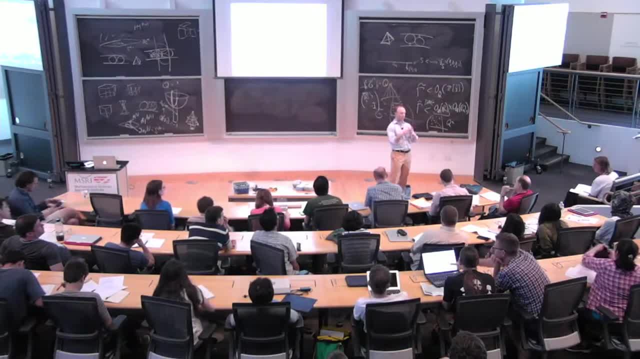 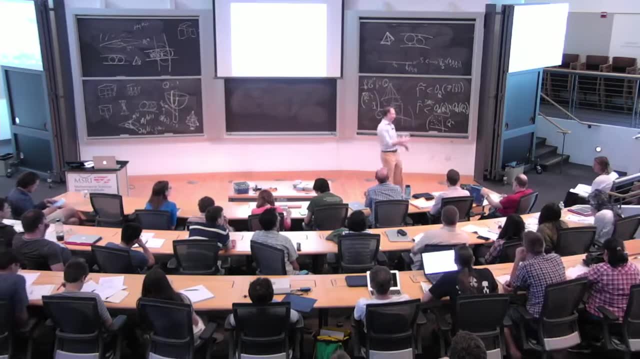 was for an arbitrary polyhedron and using the mid-sphere. So if you don't use the mid-sphere and you just say there exists some cluster- not the cluster and the dual simultaneously, then it's not rigid And the way you would geometrize a square pyramid is just to arbitrarily. 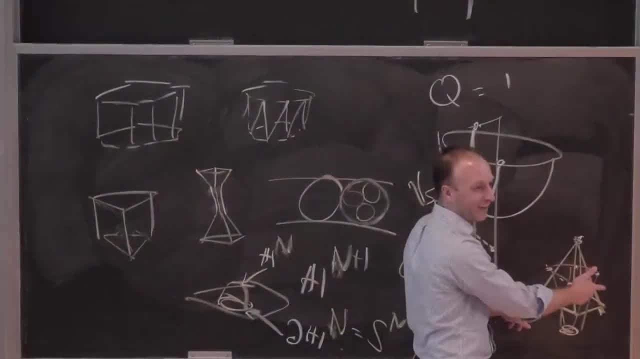 triangulate it, triangulate any face that isn't triangulated and then just forget that face when you draw the once you construct the packing. So it's not rigid unless you insist on this mid-sphere condition Simultaneously, the cluster and the dual cluster meeting it. 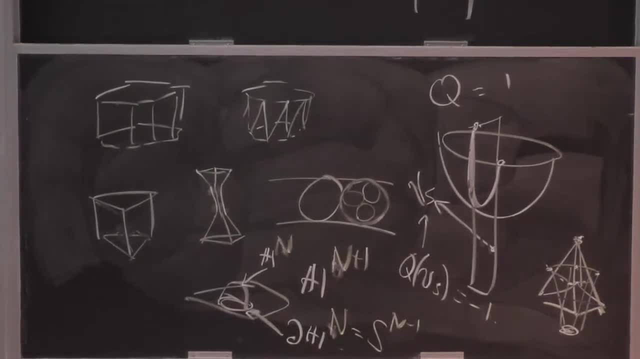 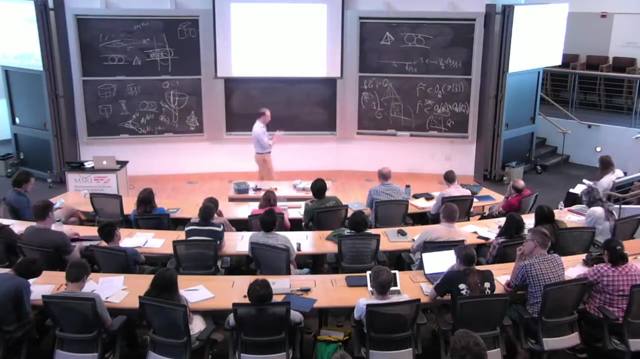 orthogonally, then it is rigid. So you're absolutely right The way it's stated most of the time, because people want to do conformal maps, approximate conformal mapping theorem from circle packings is just for triangulations. That's all you needed in that setting. Yeah, 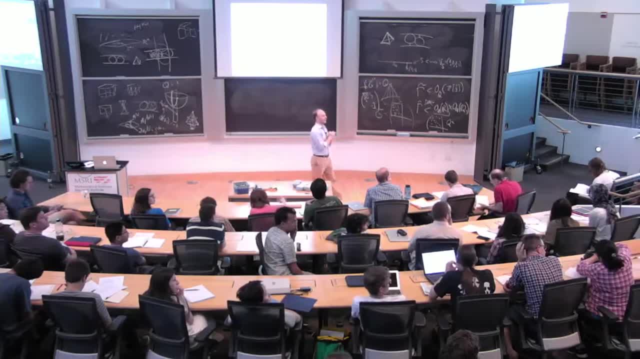 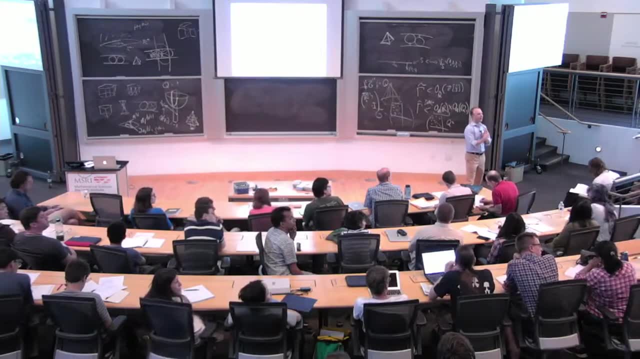 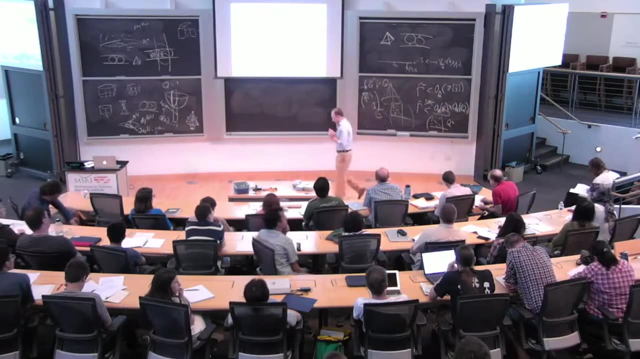 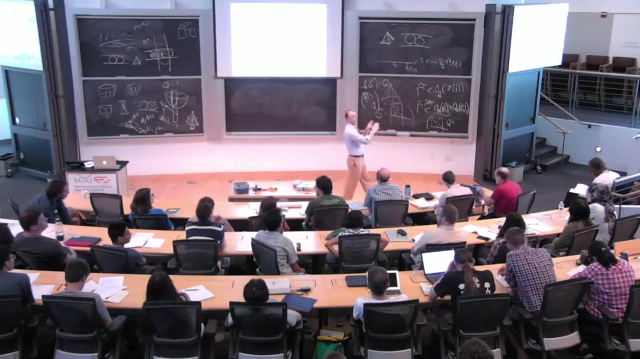 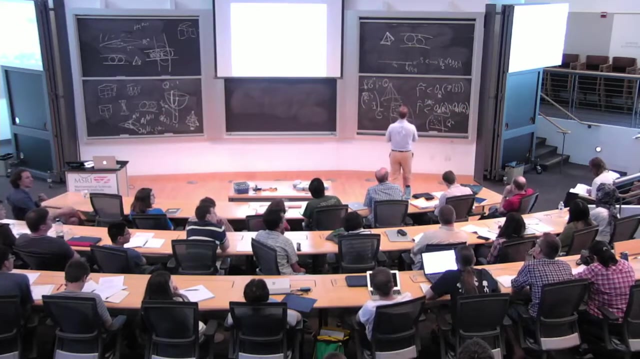 So let me rephrase your question. Maybe this isn't your question at all, but so you're saying what happens in the cases when you can't get integer bends but you can get algebraic integer bends, So what you'll get. so I didn't state the full Vinberg criterion, The full in general. 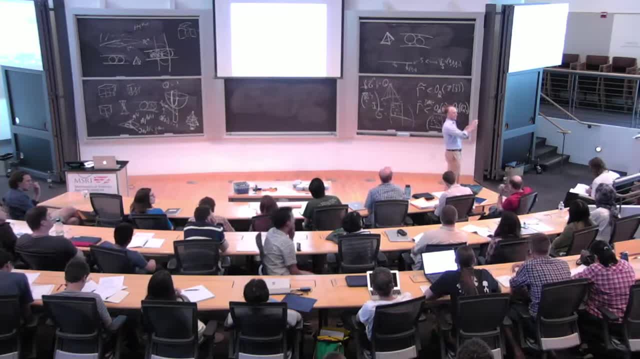 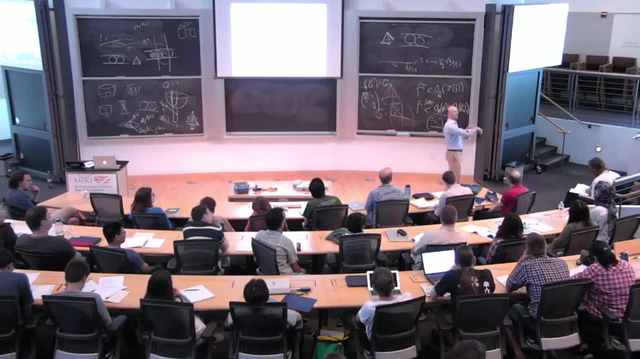 what does it mean to be arithmetic? Not just that you're some OQZ, it's that you're OQ of some ring of integers, of a totally real number field, with all but one embedding giving you, giving you definiteness, And when the one embedding gives you signature n plus one. 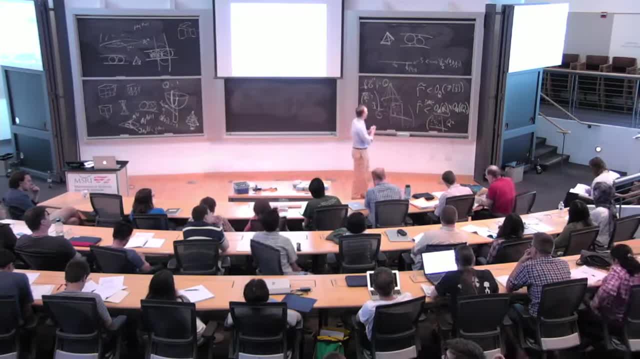 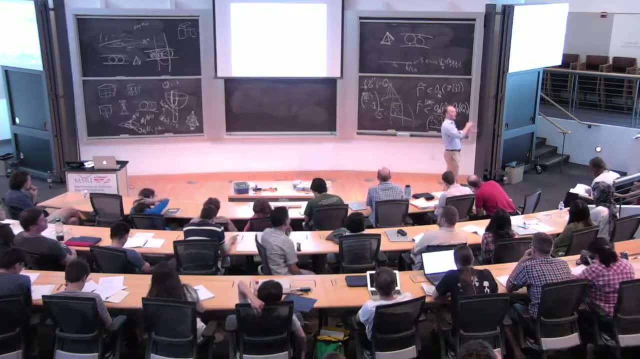 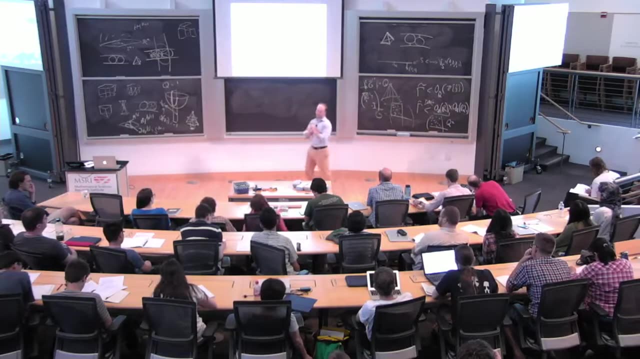 one right. That's the general criterion, And so some of these other packings will be arithmetic, not in Z but in other number fields, And the reason I want to stay away from those is because what I'm really interested in, the hope of generalizing this stuff before 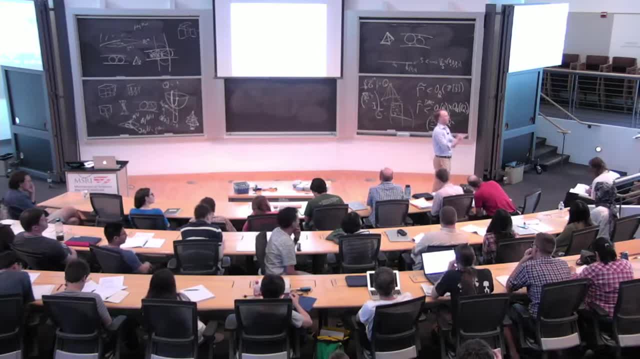 I got interested in just generalizing for the sake of understanding what's going on. I wanted to prove the local, global conjecture. So we get, we have this density, one version of it. I said: let's see where else this thing could crop up. And can we use that, Can we? 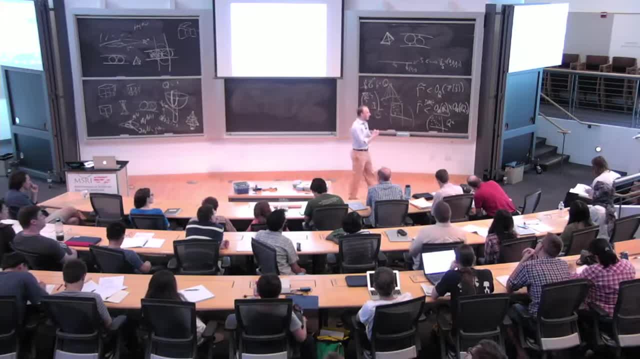 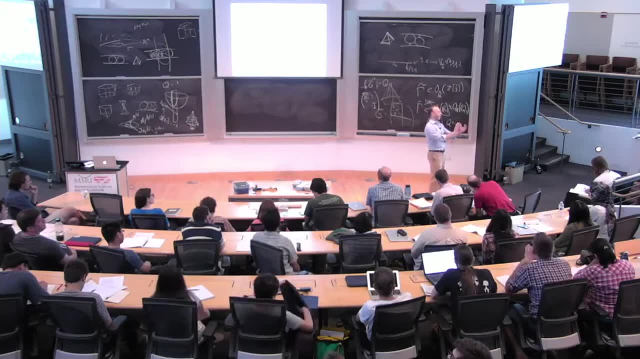 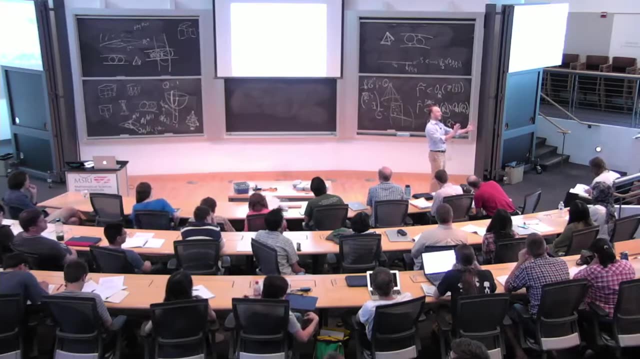 learn anything new and use that towards the local, the local global. So once you go to quadratic integers, the local global is hopeless. because even in the Apollonian case, if you allow quadratic integers, the number of circles counted with multiplicity up to up to a given. 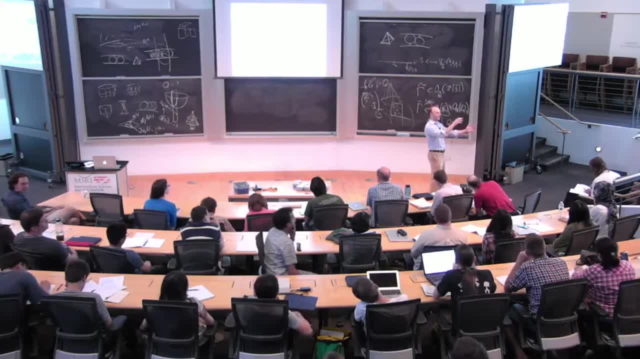 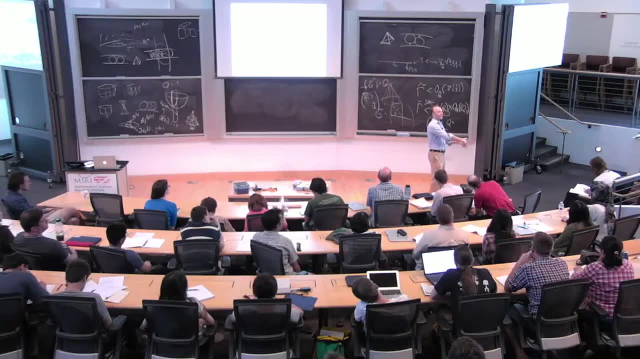 height is X to the Hausdorff dimension, So it'll be something between one and two, let's say one and a half. But if you want there to be a local, global principle, it has to hit every algebraic integer. but now they're, it's in a rank two, abelian group, And so there's. 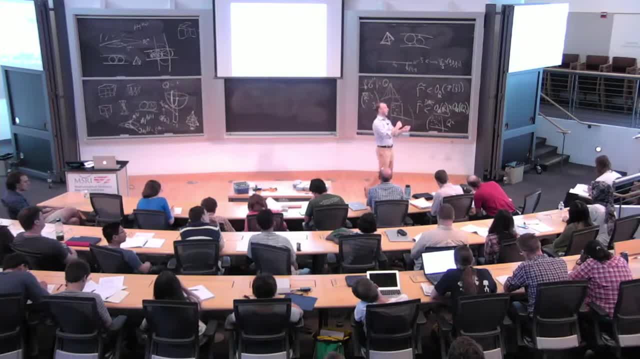 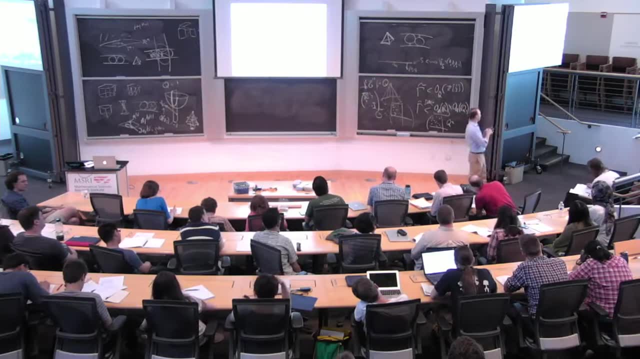 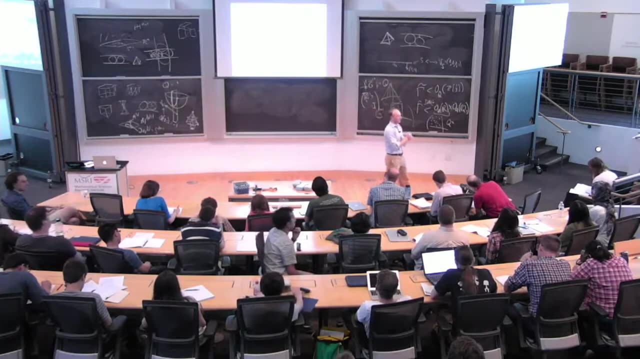 X squared of them, So it's not a chance. So from that point of view, the count is just off And what I really care about is the local, global principle. So I'm sticking to integers, but you're absolutely right that the general question of, uh, arithmeticity. I should allow these these more general examples. 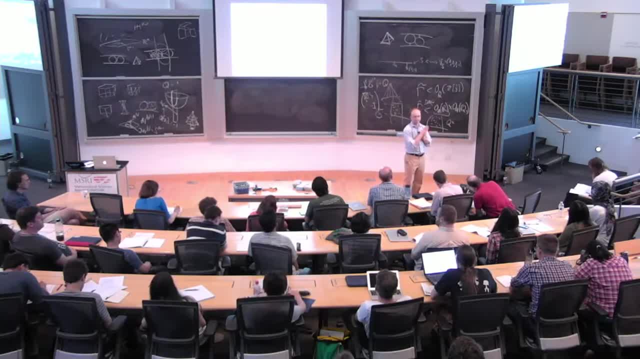 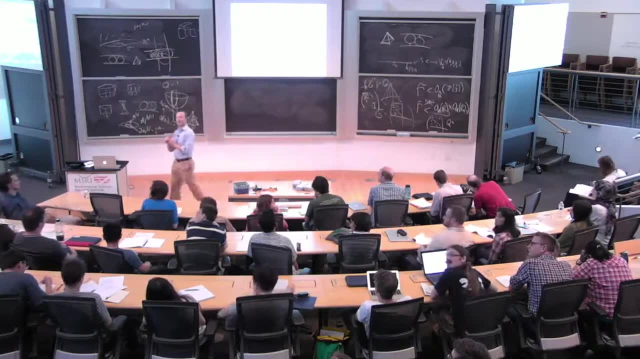 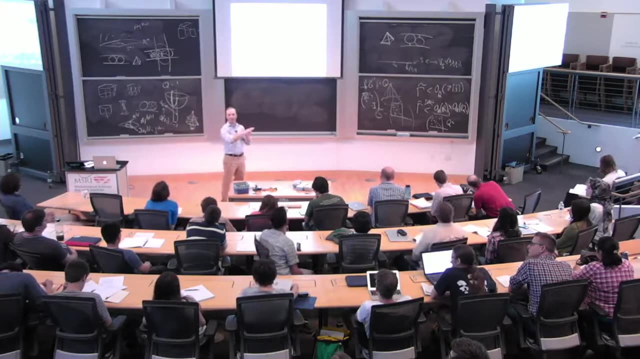 And that's something we're we're also looking at There. Oh yeah, Okay, Okay, Okay, Okay, Okay, Perfect. So let's study that. So the, the super packings are, or the packing is coming from poly J, the super packings are. 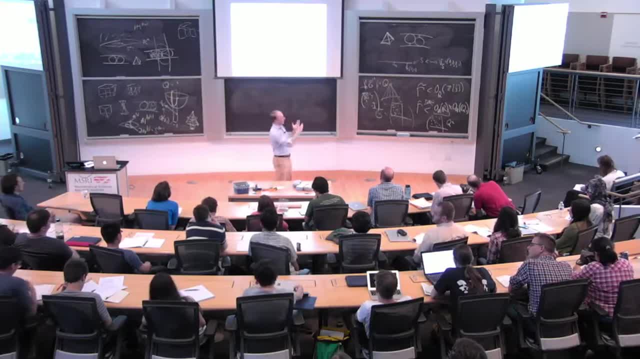 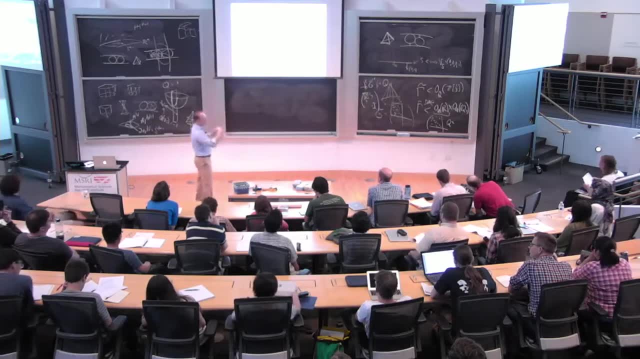 dense. So they're not a but the the. these other packings have all different wild, uh Hausdorff dimensions Each one, and we have an infinite collection of com of different House Turf dimensions. You know, from these growth of these glueings along, um, along. 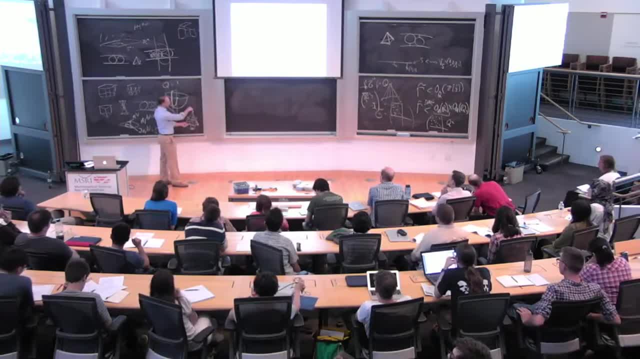 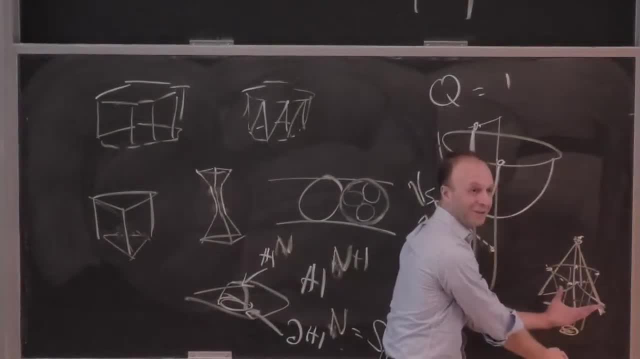 vertices and gluing his long faces. by the way, the square pyramid is half of an octohedron, because 3.5 magnitudes for Three would be taking the square pyramid and gluing along a face another square pyramid down here. 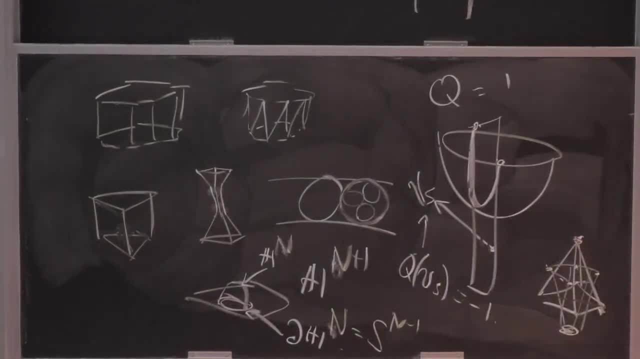 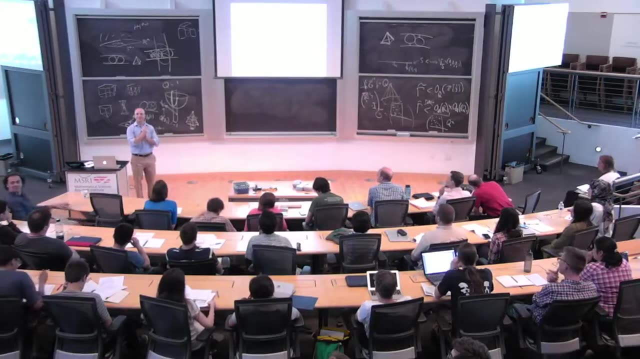 So that's another reason. that's the same, essentially the same- as the octahedron. So the octahedron is not maximal. The square pyramid is maximal. Yeah, did I answer your question? Okay, Yeah, the Hausdorff dimensions, yeah, 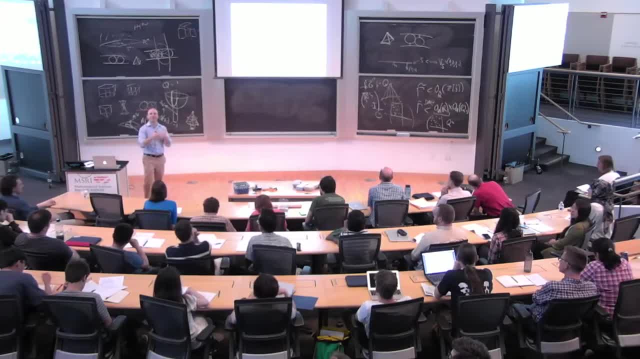 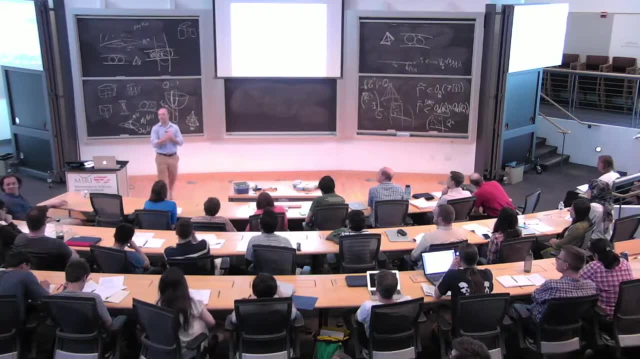 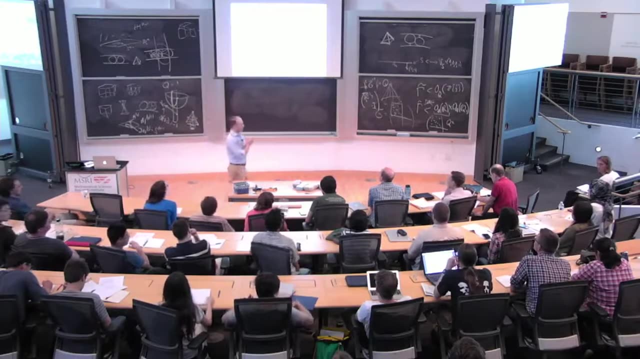 The Apollonian one is. I used to think it was a special number. No, it's just some random number And there's a million of these. There's infinitely many of these random numbers. So, if the thing you okay. so this is essentially.